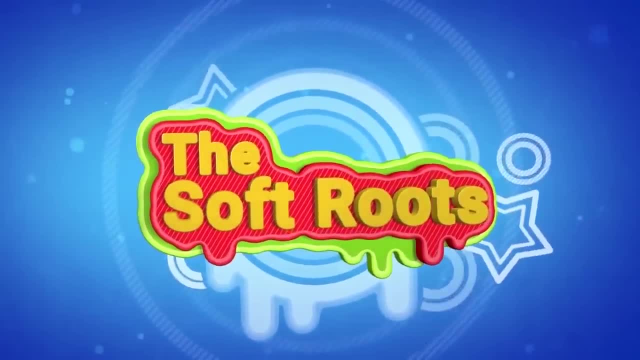 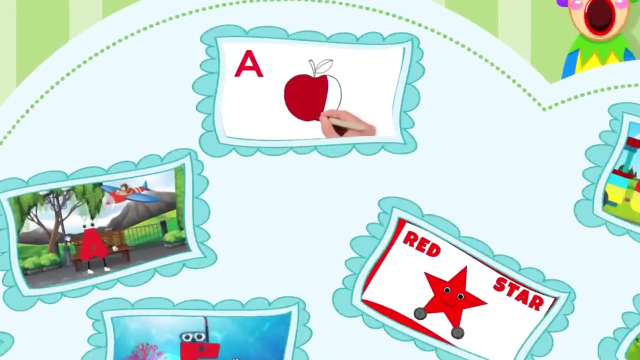 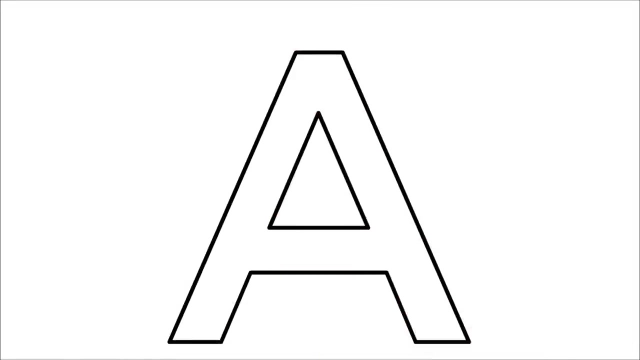 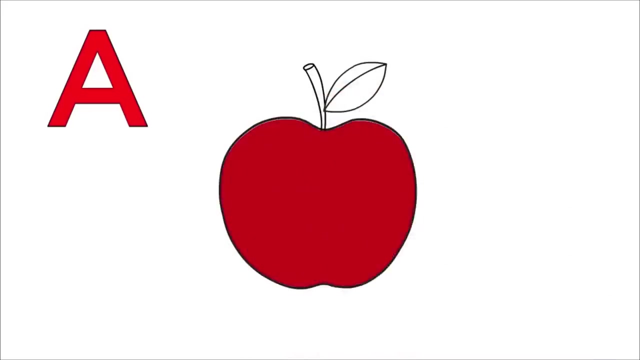 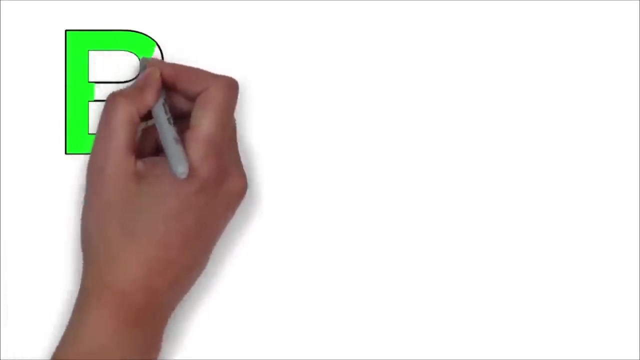 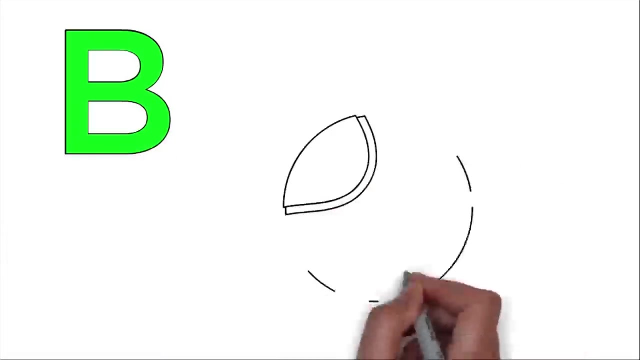 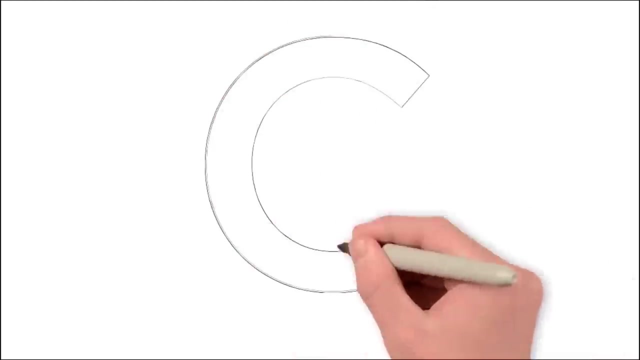 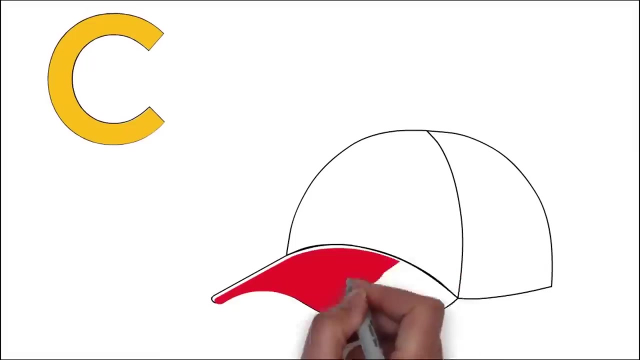 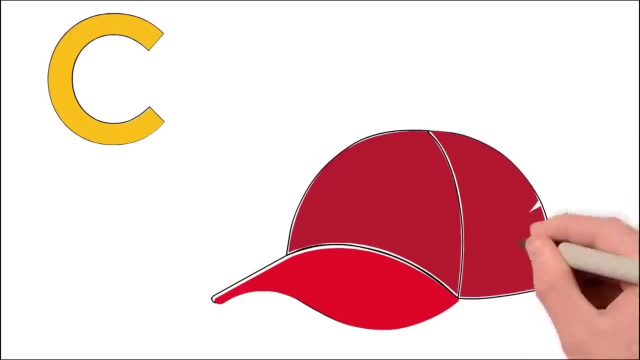 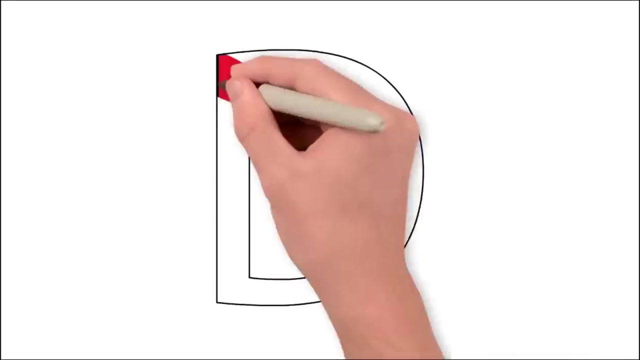 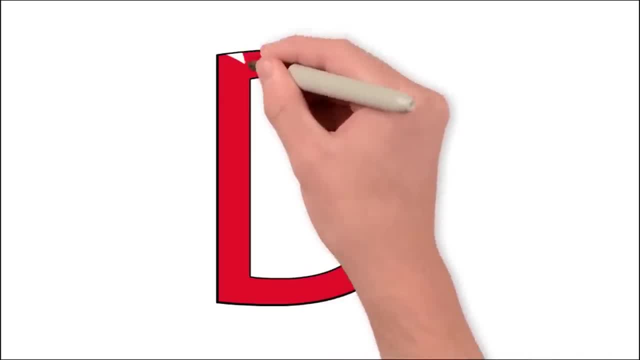 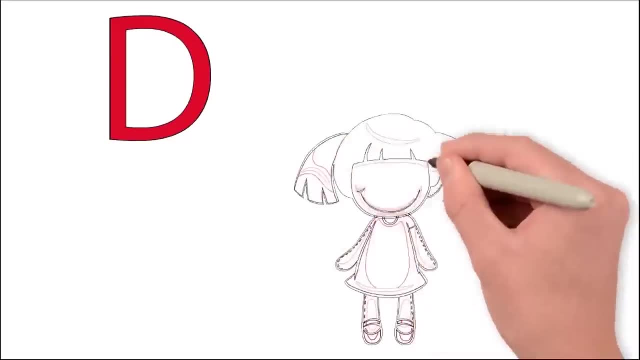 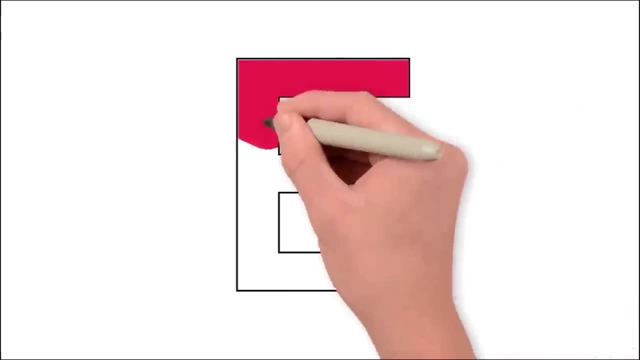 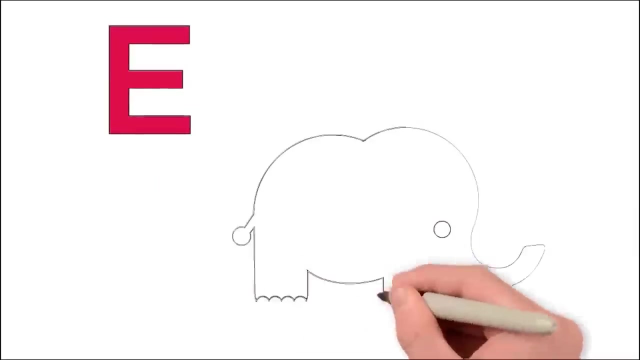 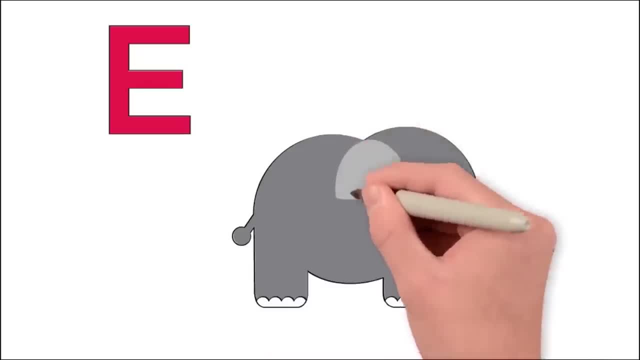 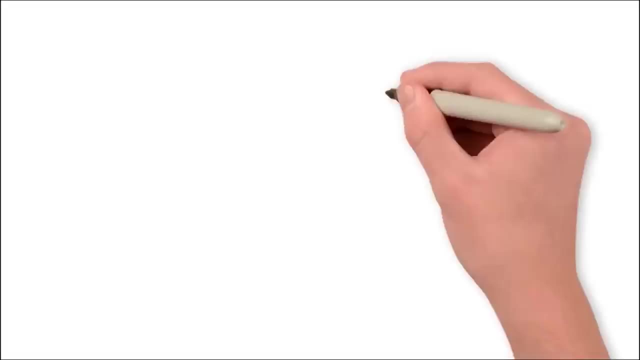 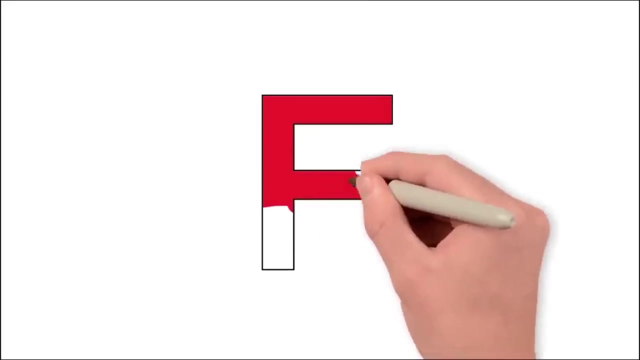 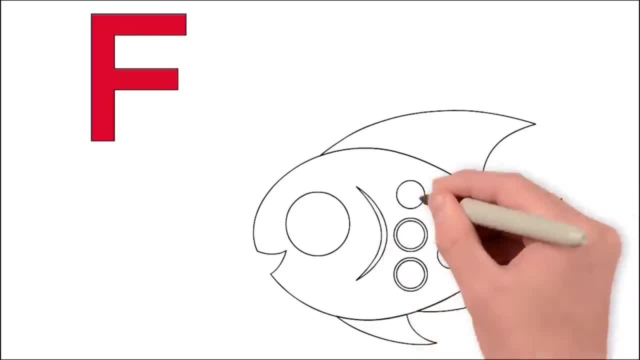 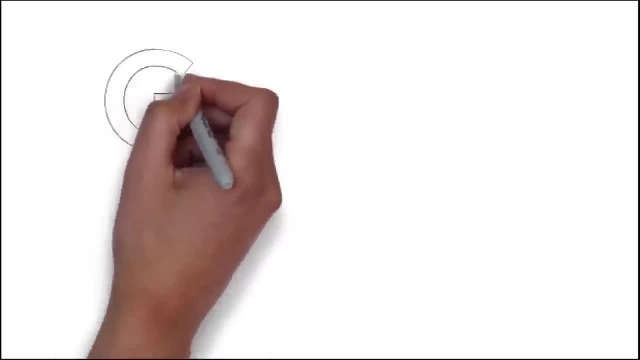 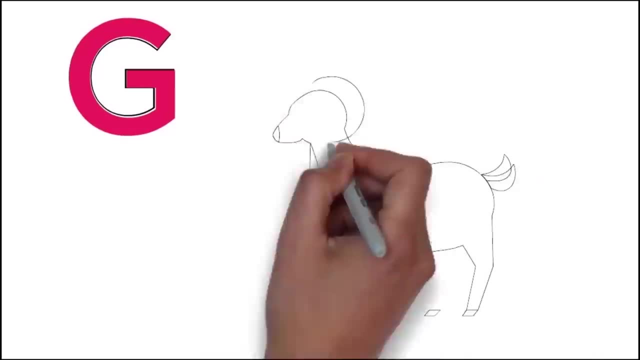 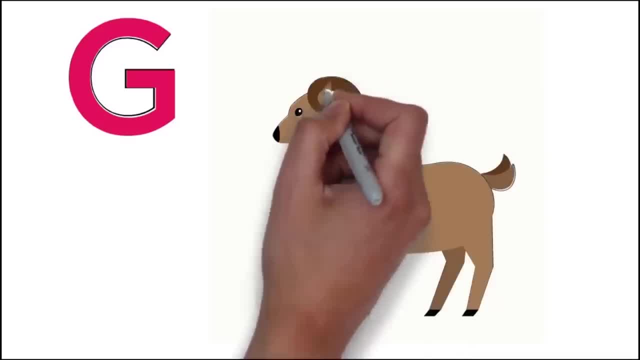 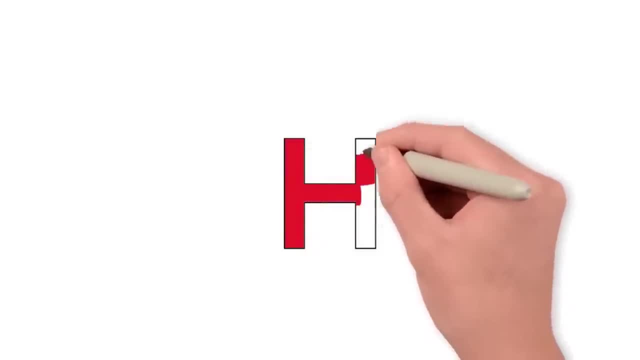 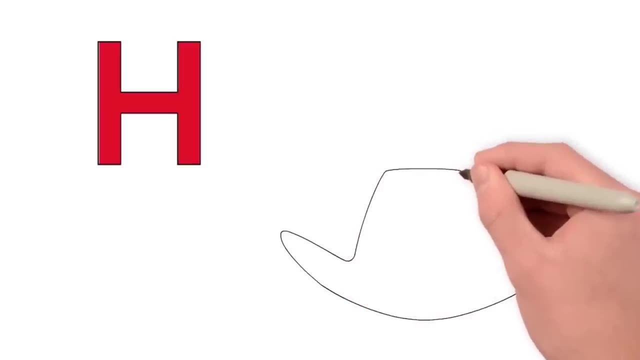 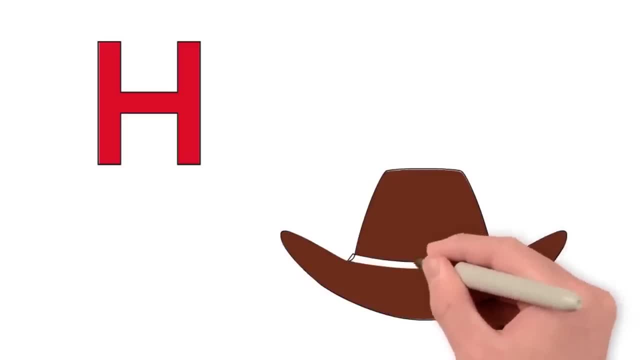 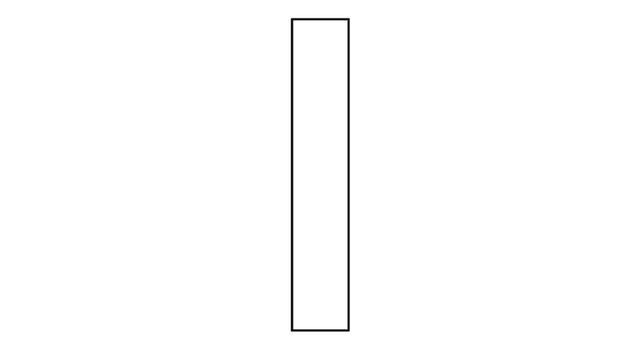 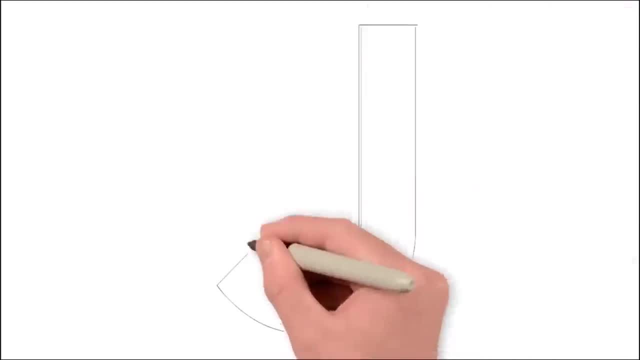 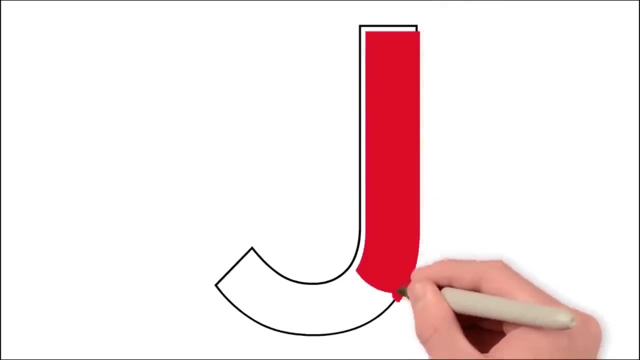 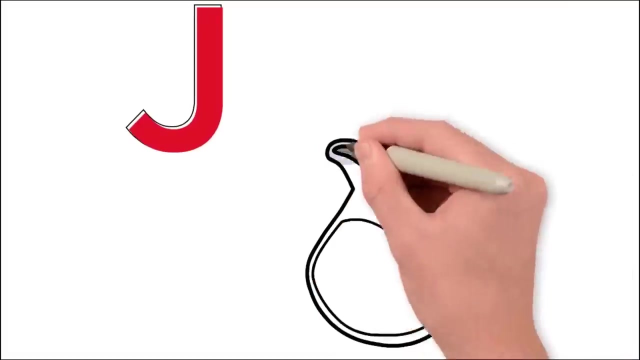 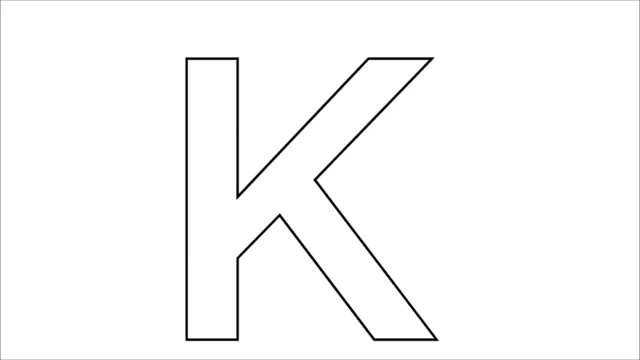 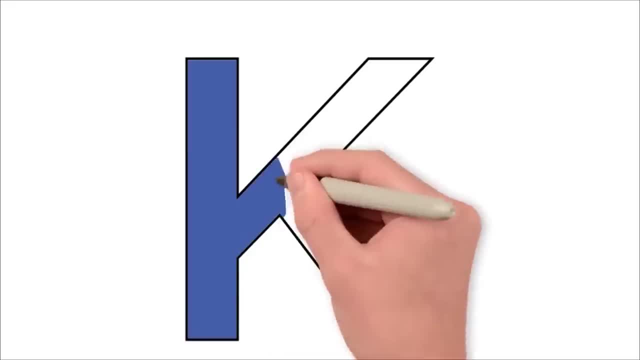 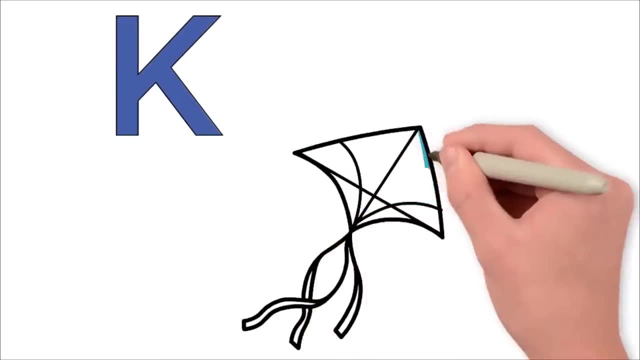 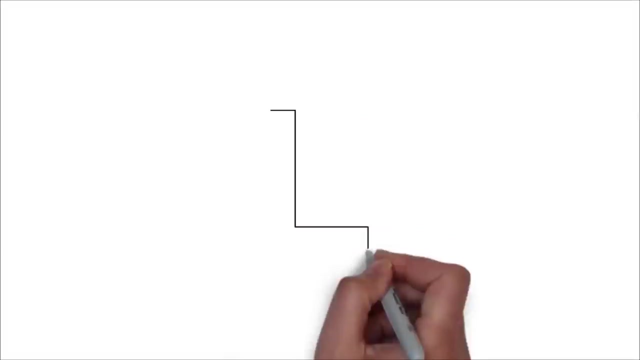 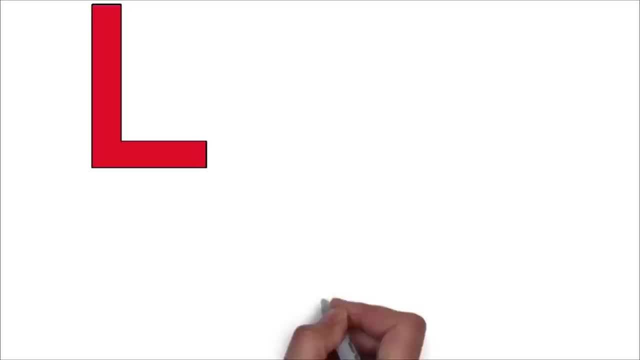 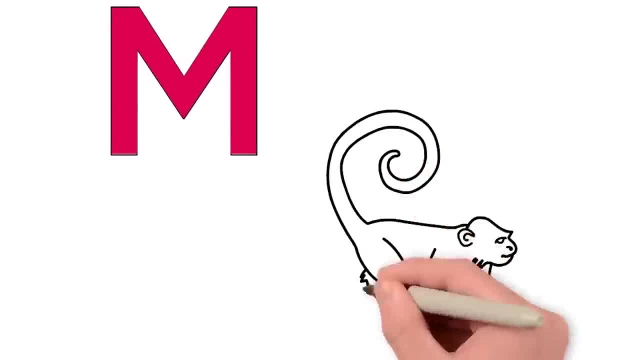 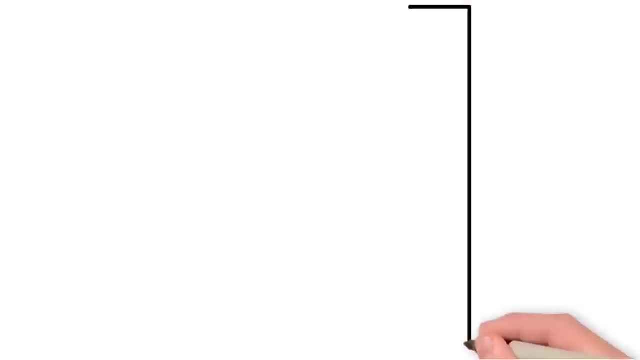 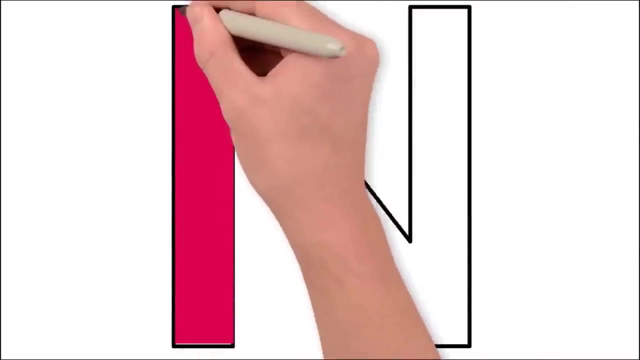 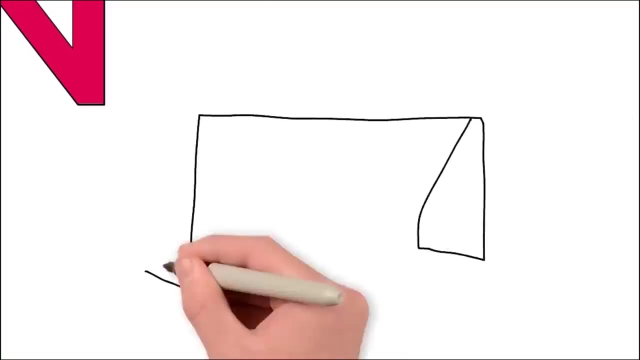 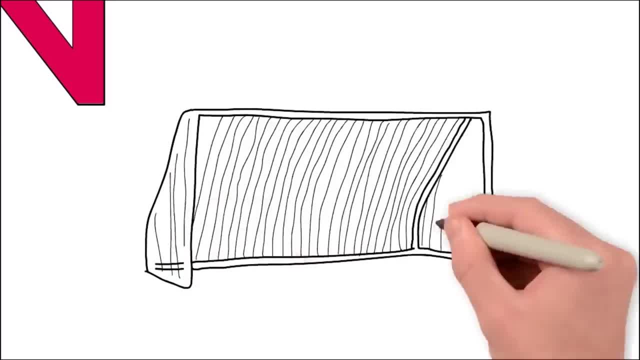 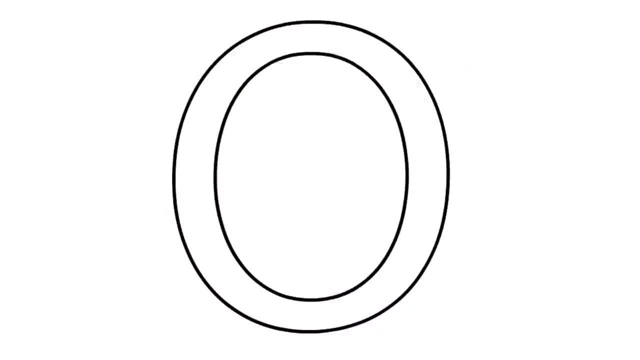 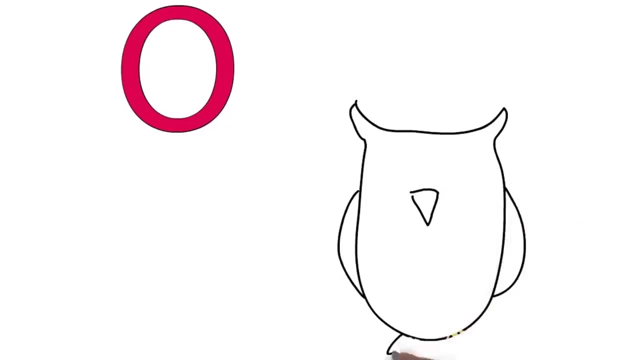 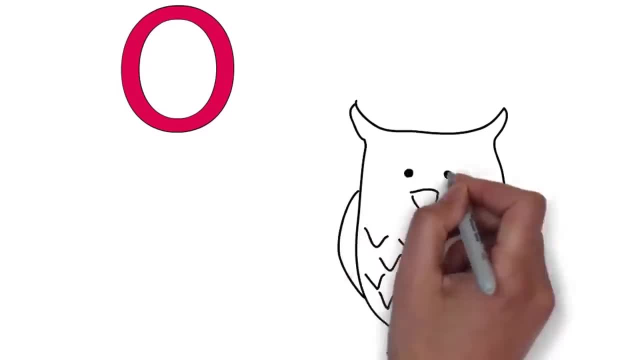 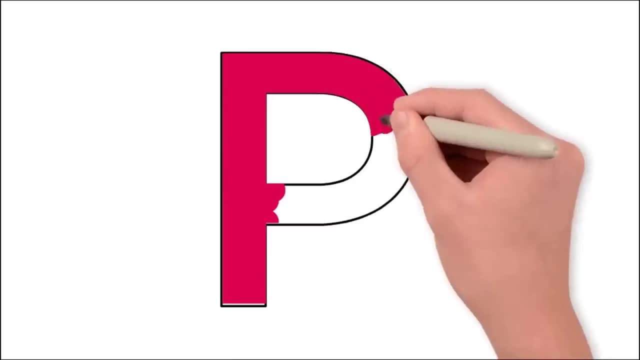 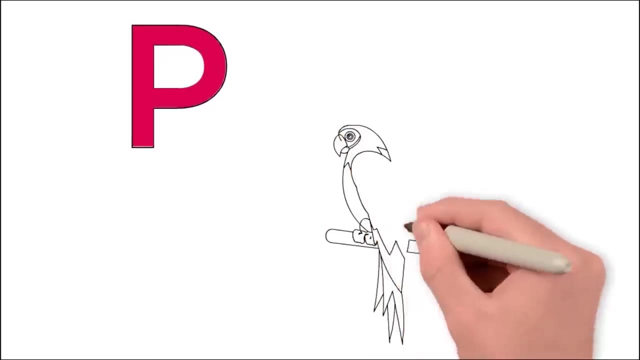 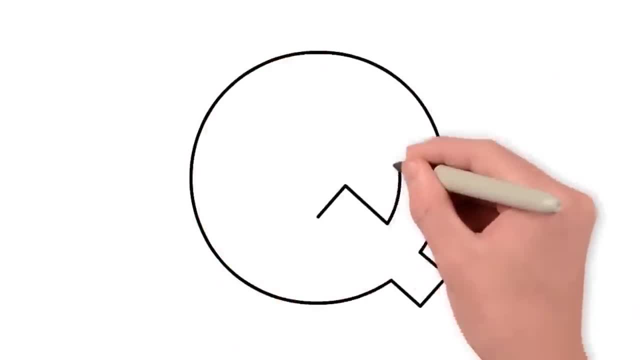 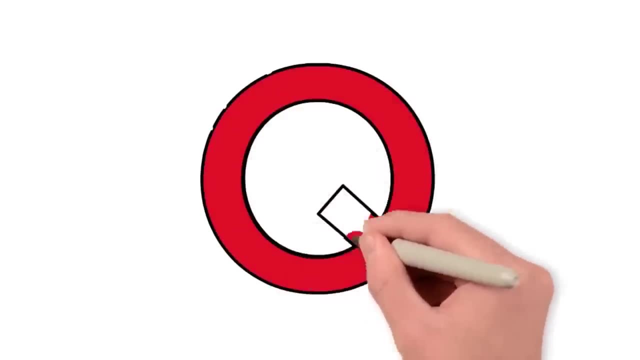 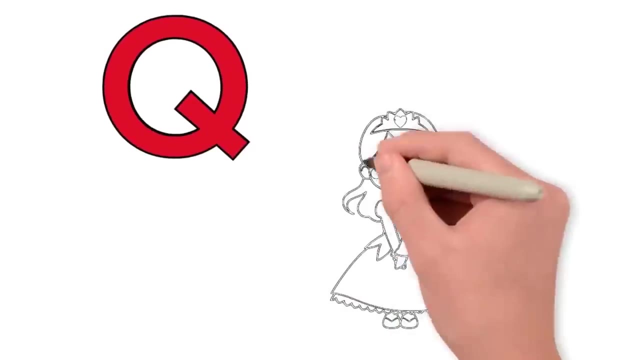 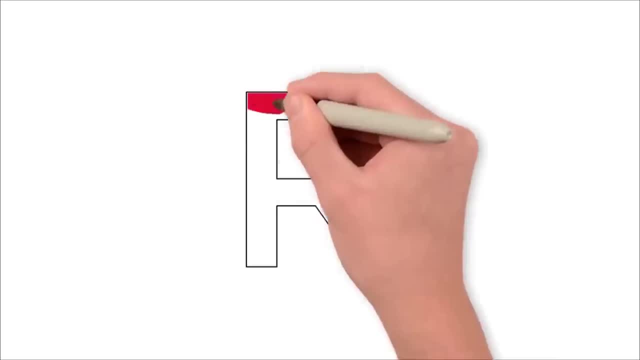 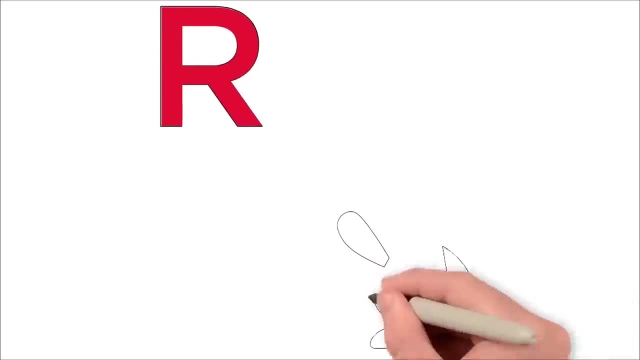 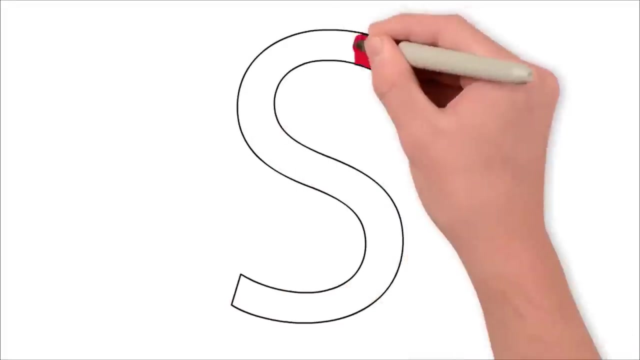 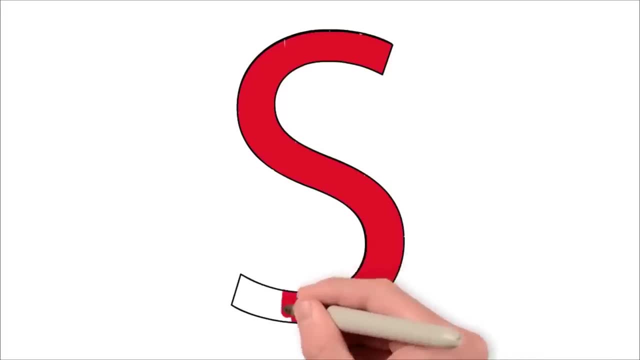 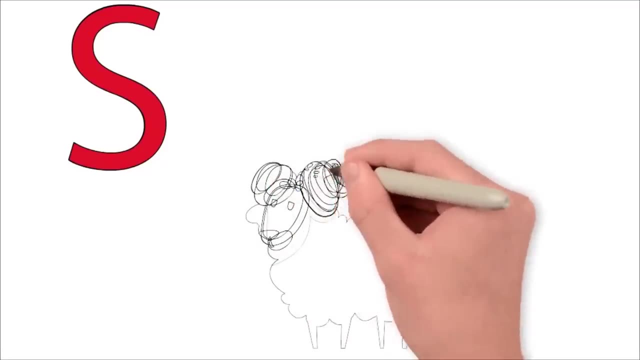 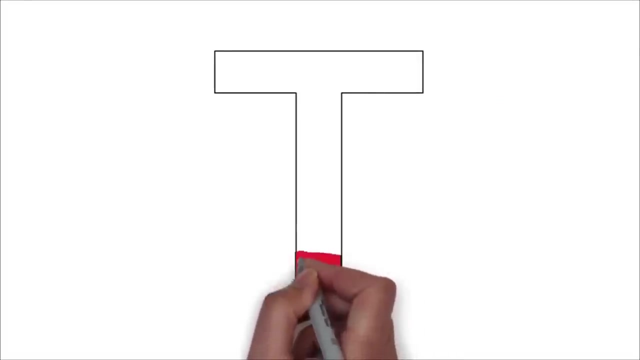 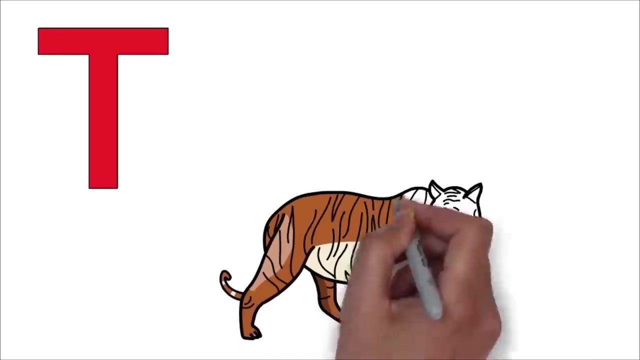 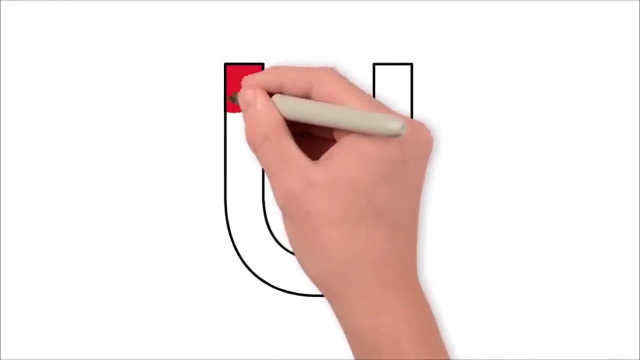 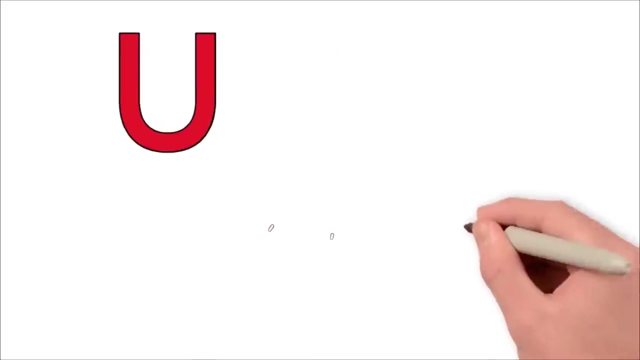 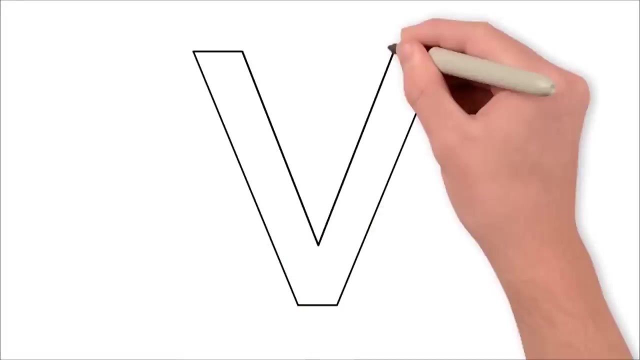 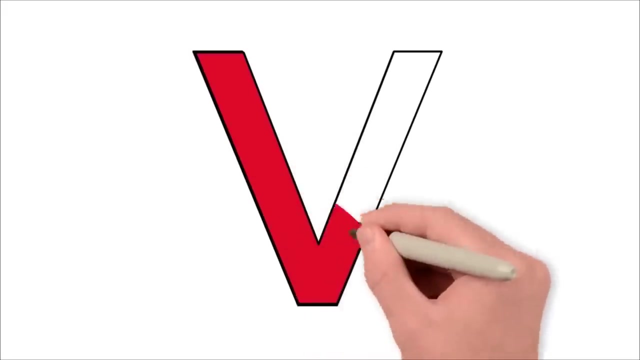 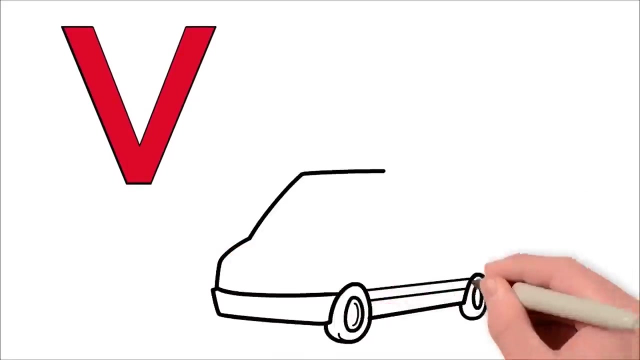 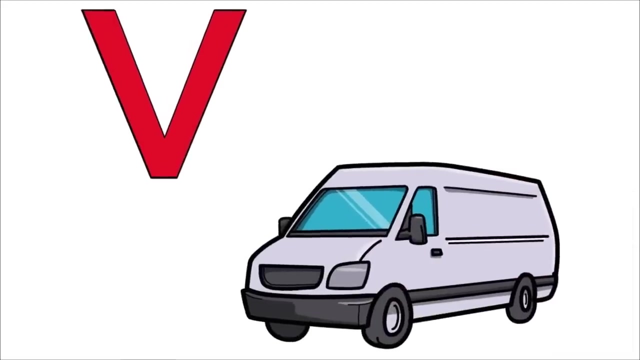 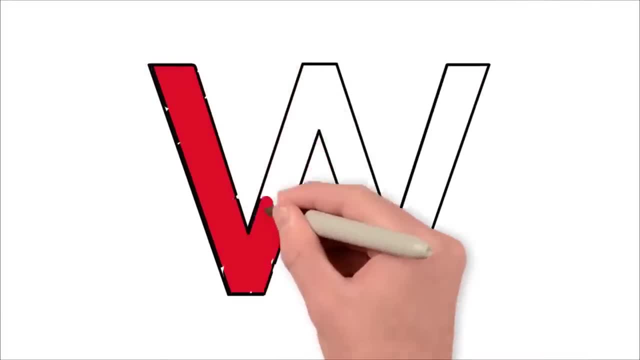 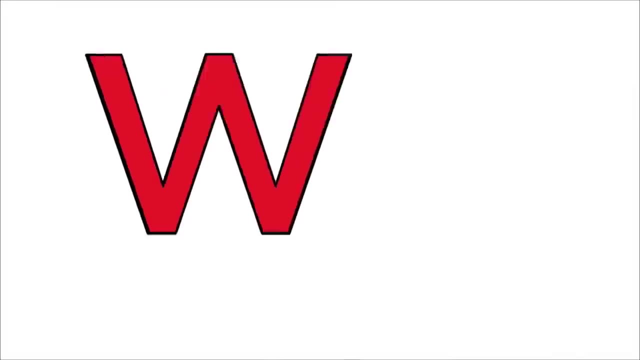 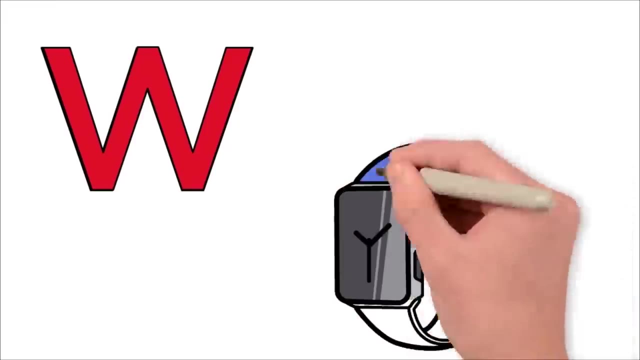 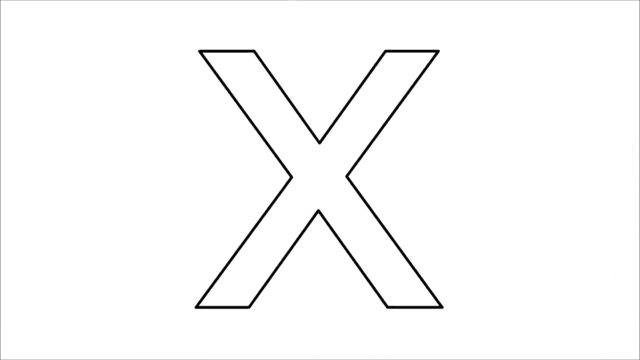 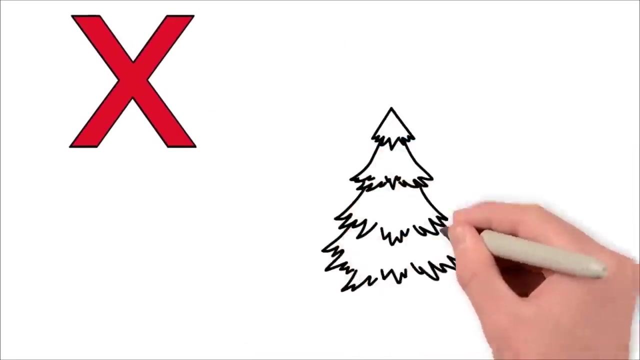 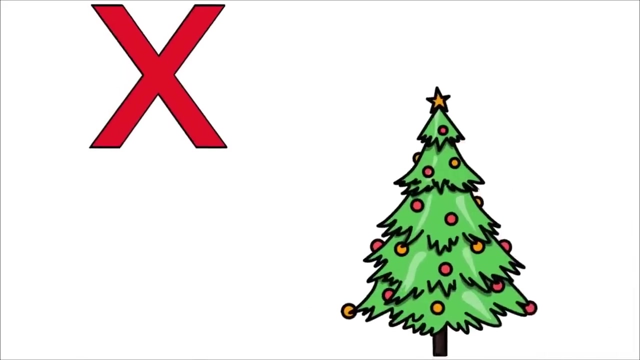 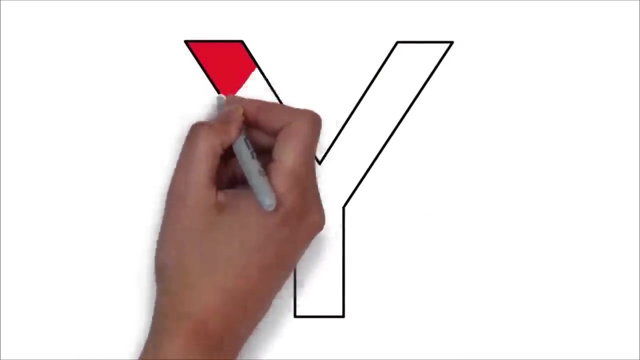 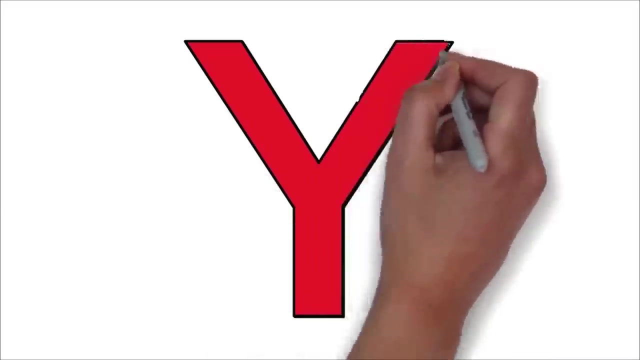 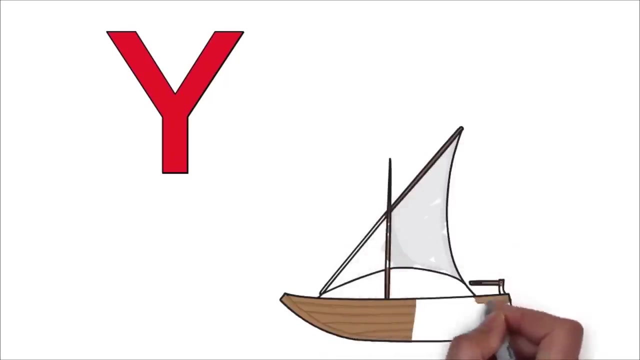 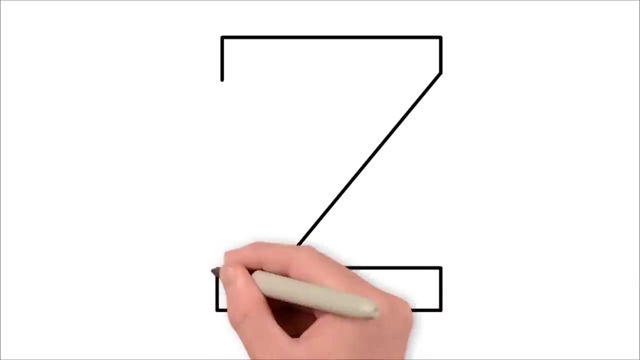 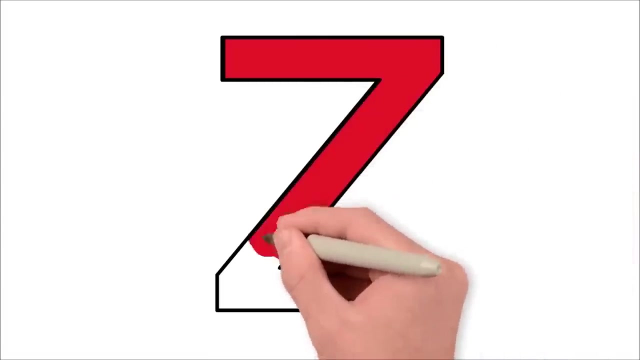 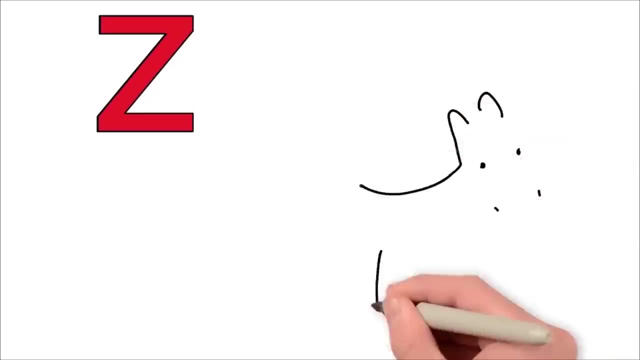 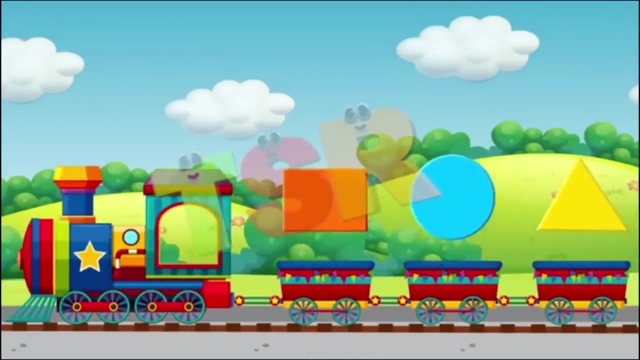 W. W Watch Blue Watch X X Christmas Tree- Green Christmas Tree. Y Y Y Y Yacht Yacht Brown, Yacht Z Z, Z, Z, X, X, X, Y, Y, Y, X, Y Z, Y, Y X, Y, Y, Y, Y, Y, Y, Z, Z, Z, Y Y Z. 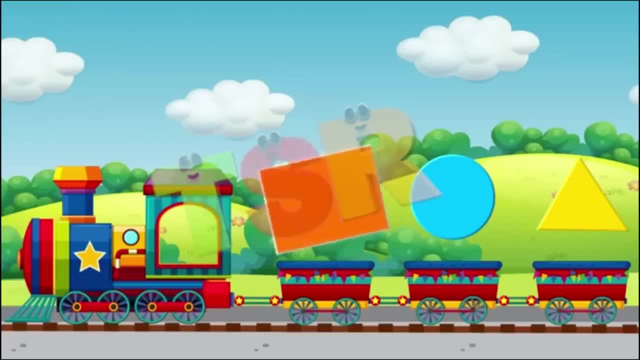 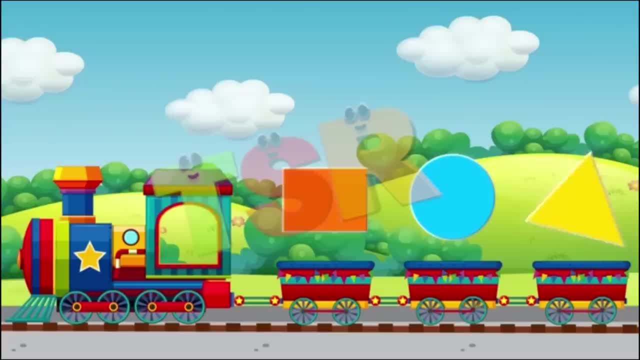 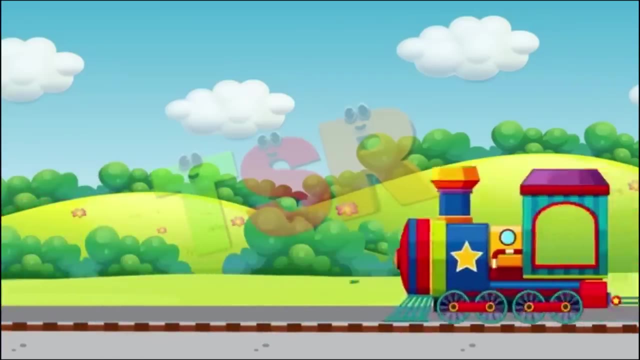 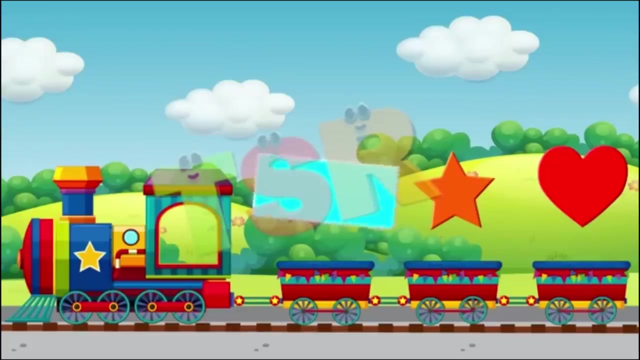 I have three sides. I'm a triangle- triangle. We are shapes. you can see us everywhere. I'm a rectangle rectangle, like a really long square. I have four sides. I'm a rectangle rectangle. I'm a star. I'm a star in the sky. 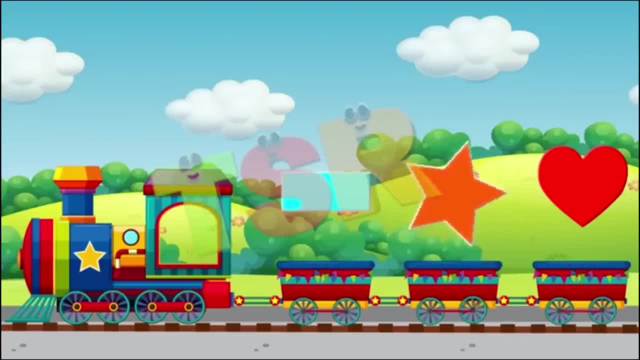 So so far, I have five pointy arms. I'm a star, I'm a star. I'm a heart, I'm a heart. I'm so curvy and so smart. I'm a really lovely shape. I'm a heart, I'm a heart. 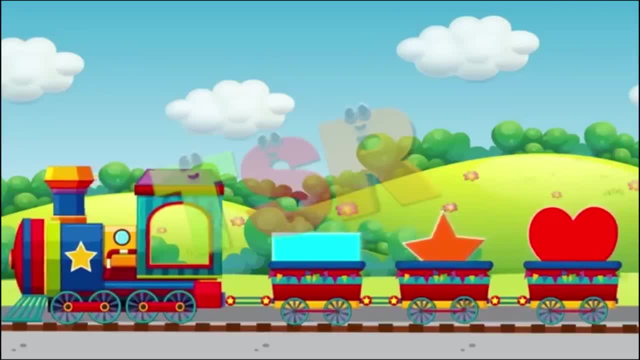 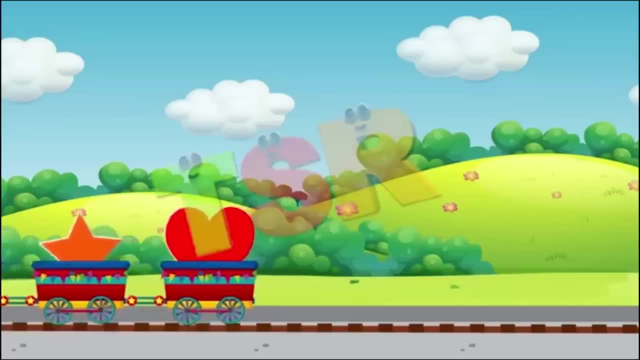 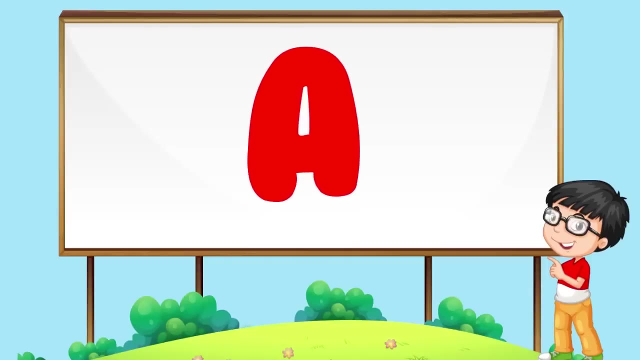 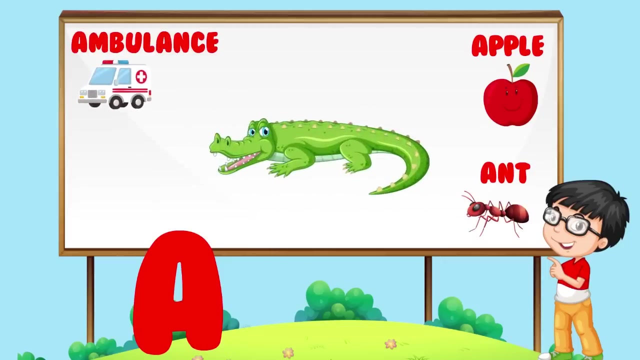 We are shapes. you can see us everywhere We are shapes. We are shapes. you can see us everywhere We are shapes. I'm I'm a square, I'm a triangle. I go round and round and round. I'm a triangle, I'm a circle, I go round and round and round. 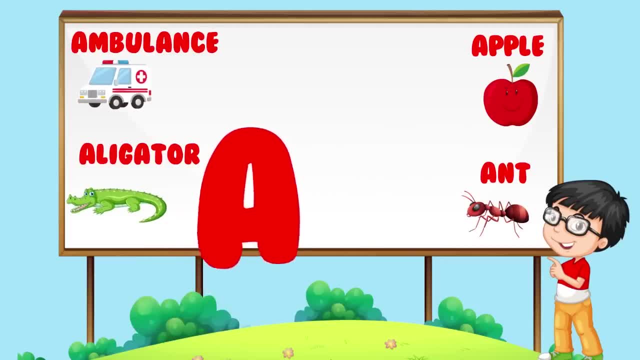 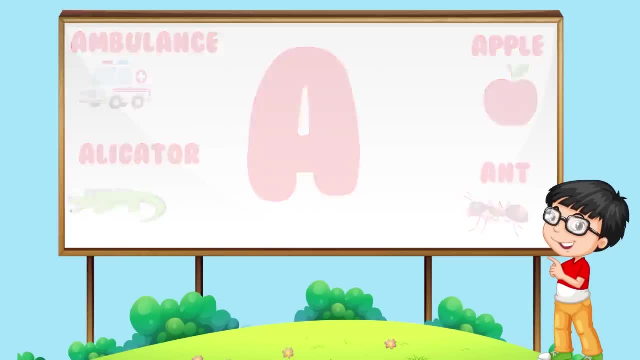 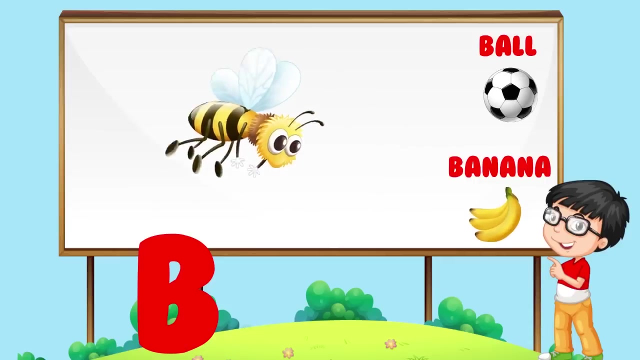 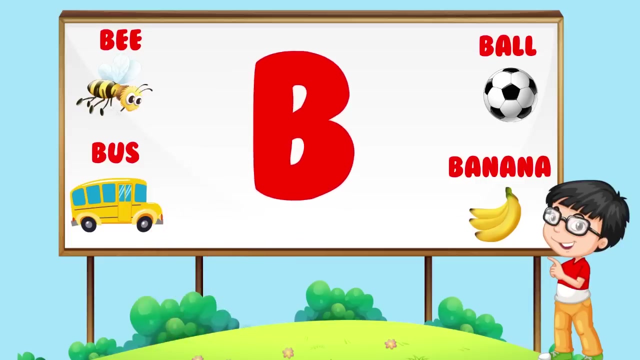 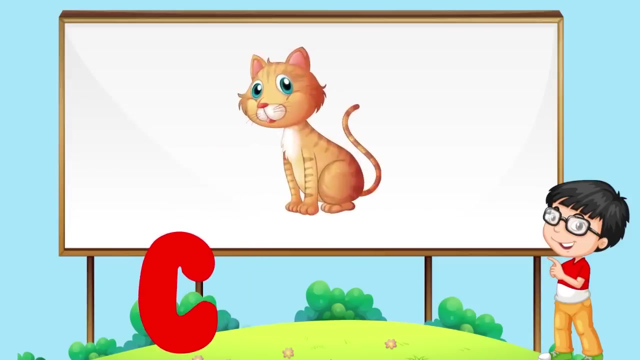 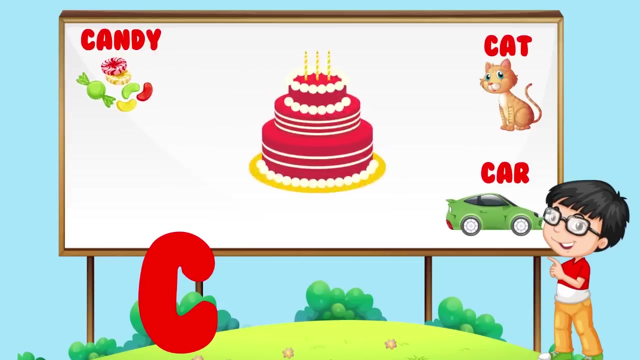 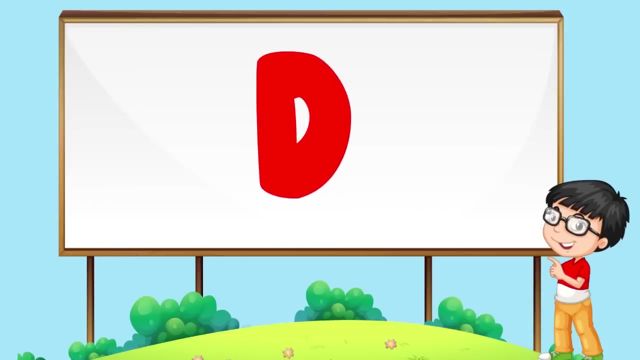 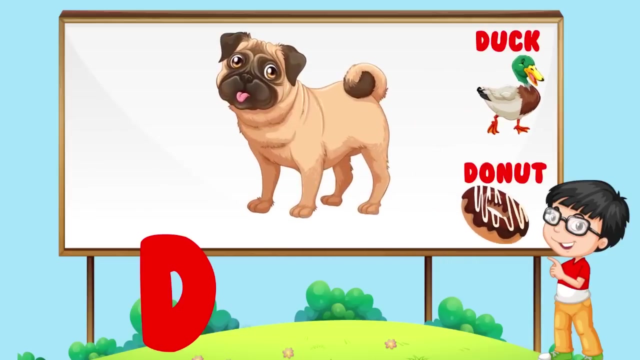 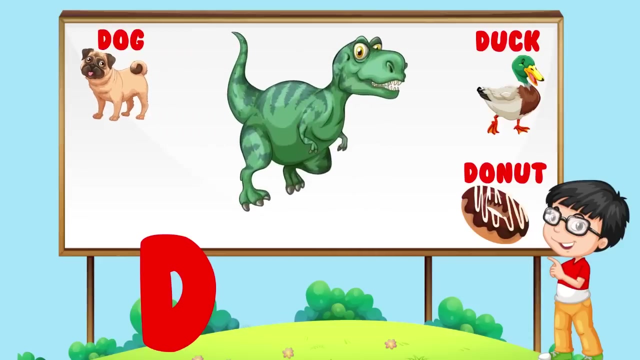 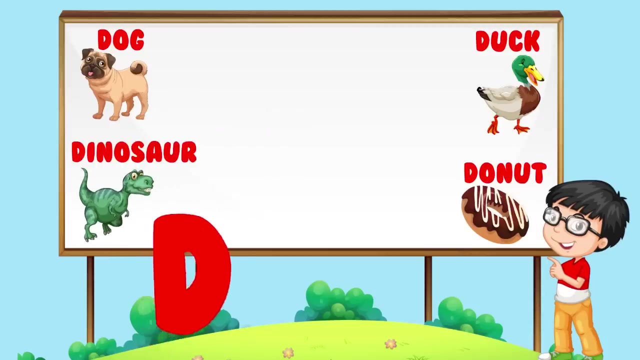 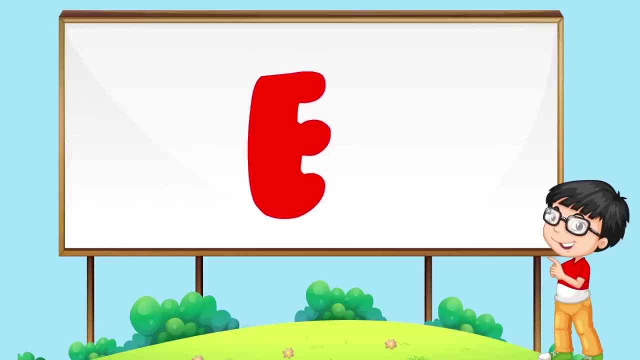 B for Alligator, B, B for Ball, B for Banana, B for Bee, B for Bus, C for Cat, C for Car, C for Candy, C for Cake, D for Duck, D for Doughnut, D for Dog, D for Dog, D for Dinosaur, E. E for Elevator. 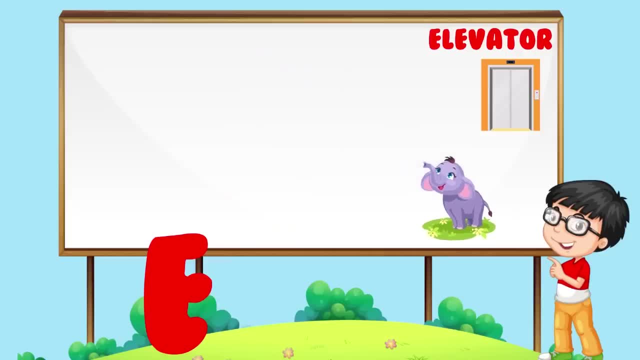 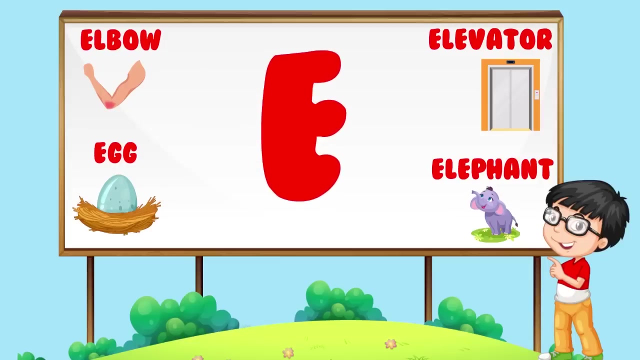 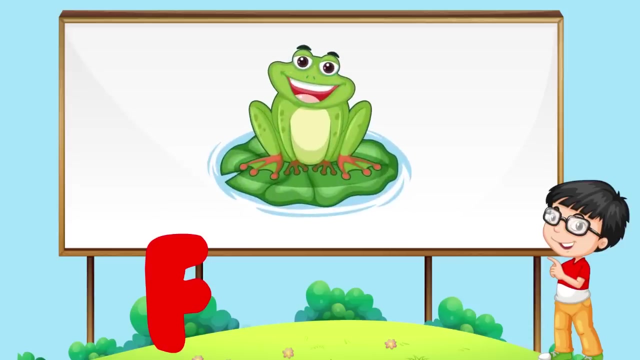 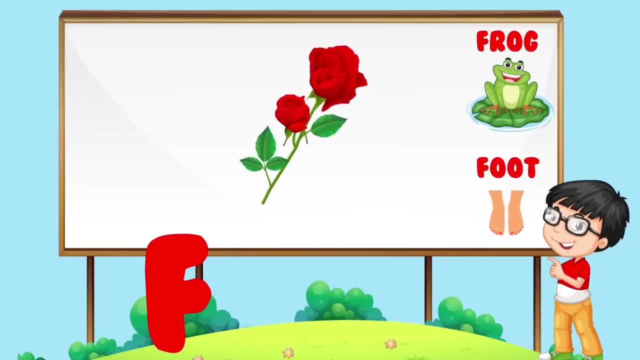 E for Elephant E for Elbow E for Egg E for Rabbit E for Bastard E for Kale E for Fizz E for Cousin E for Cousin E for Frog E for Frog E for Frog. E for YEAR F for Frog, F for Frog, F for Frog. 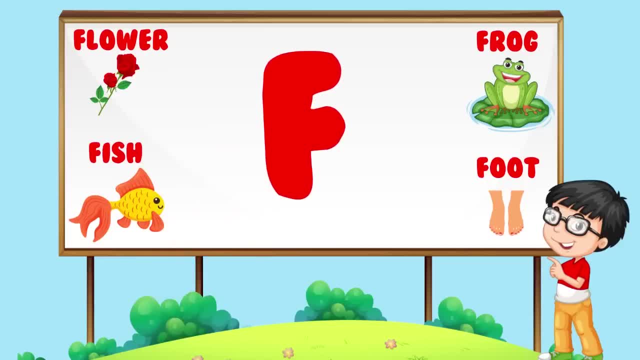 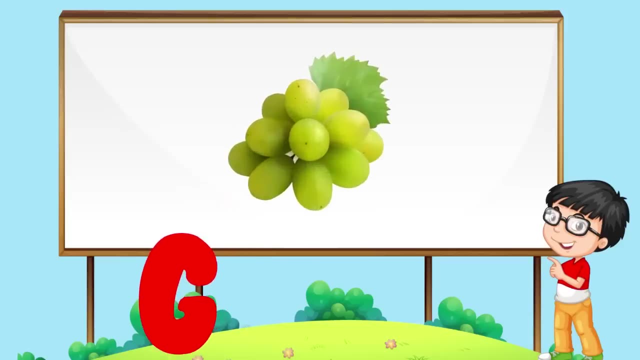 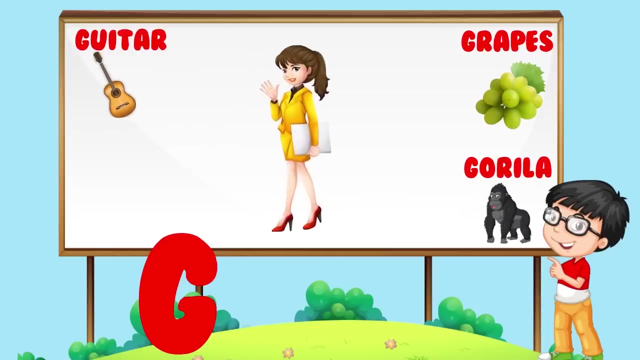 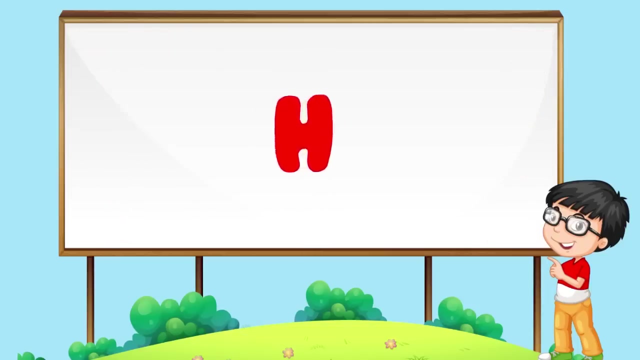 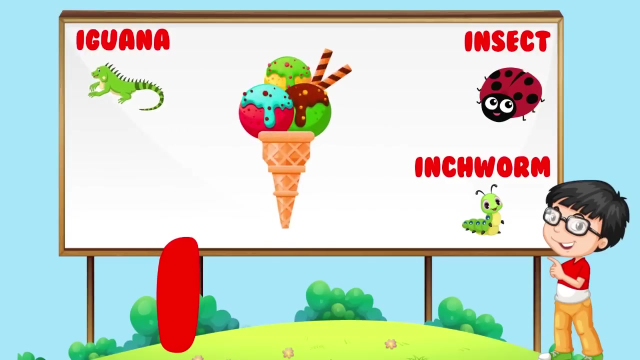 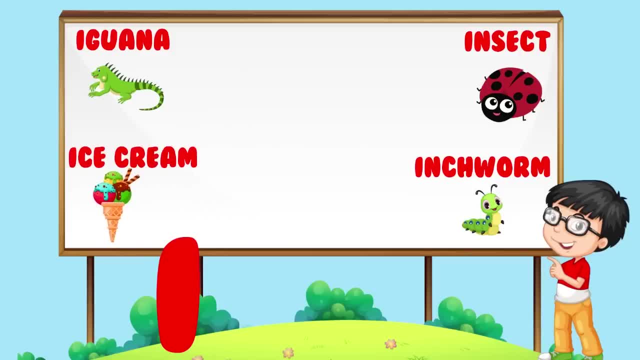 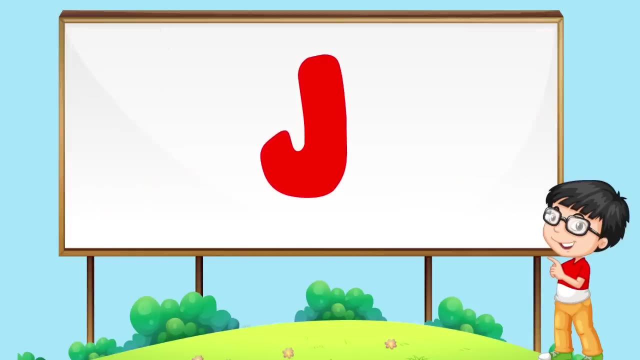 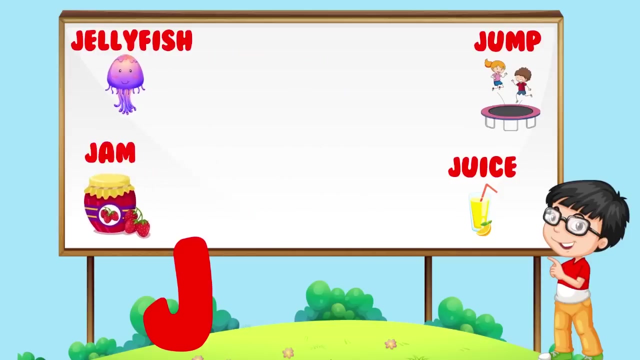 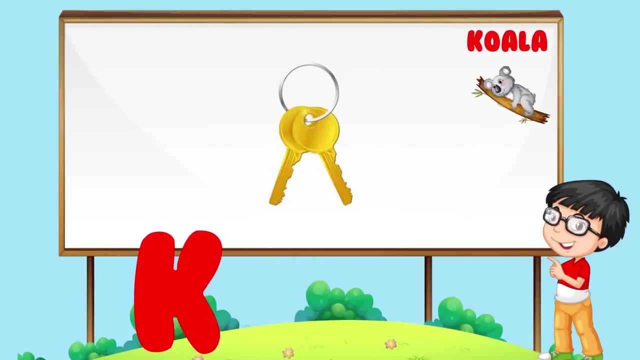 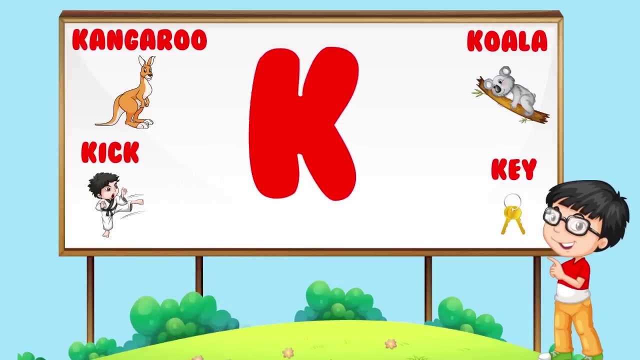 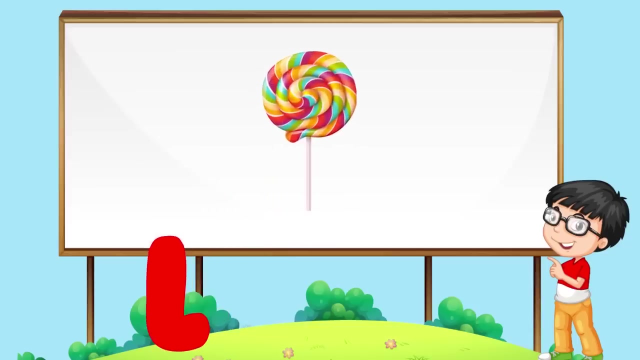 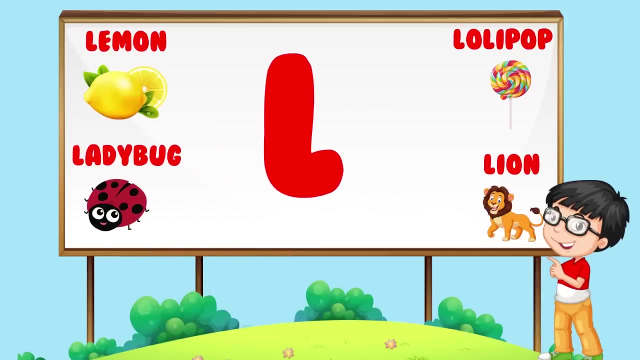 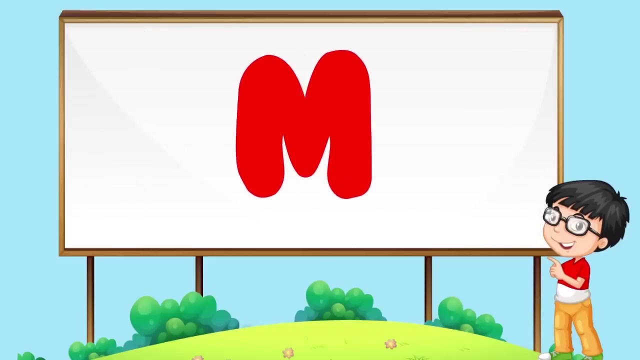 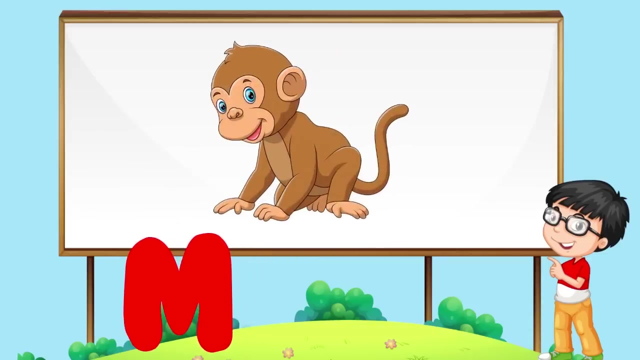 Thank you for watching. J for Jump, J for Juice, J for Jellyfish. J for Jump. K for Koala. K for Key, K for Kangaroo, K for Kick. L for Lion. L for Lemon. L for Ladybug. M for Monkey. M for Monster, M for Monkey. 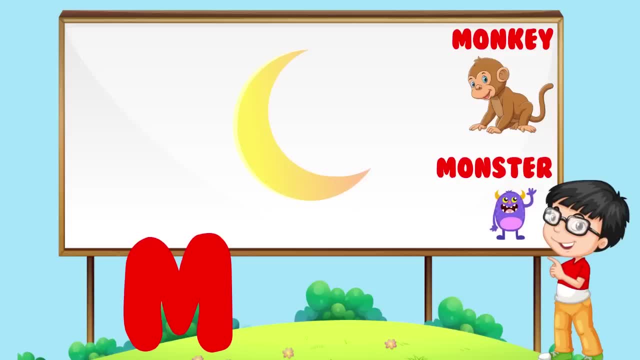 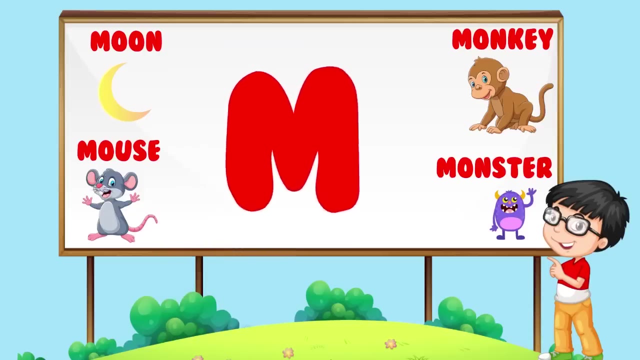 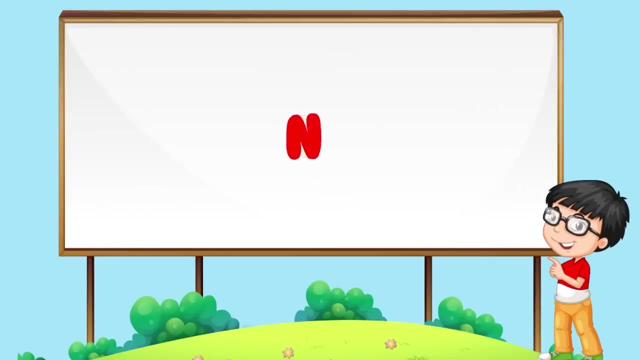 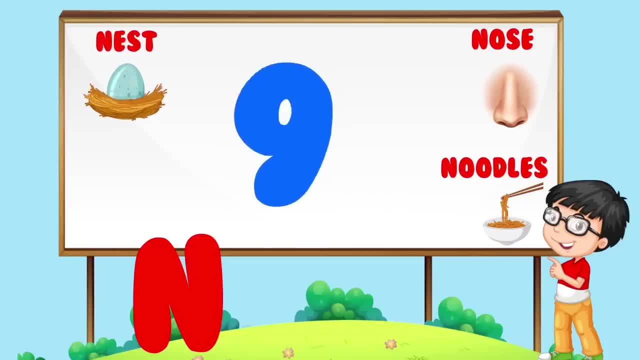 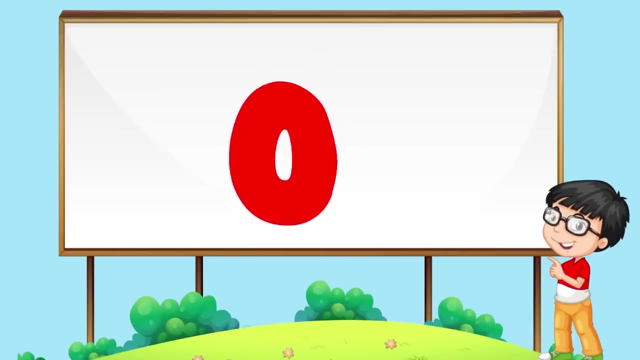 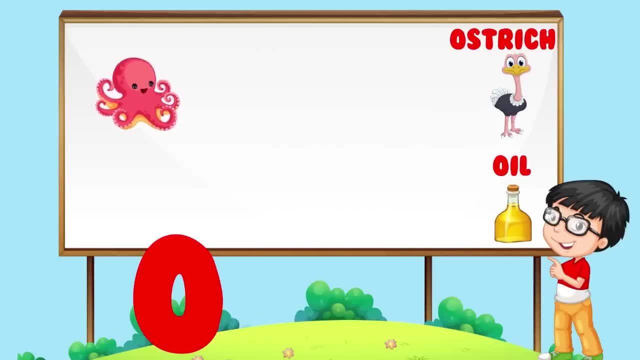 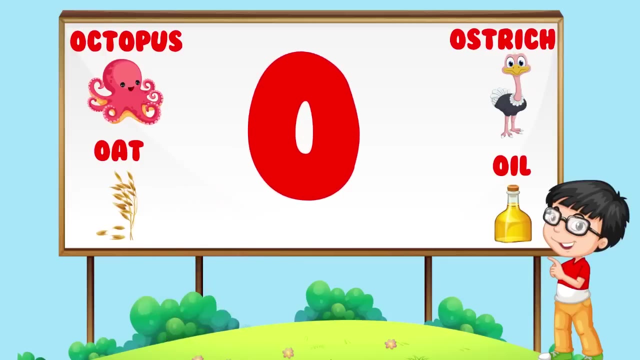 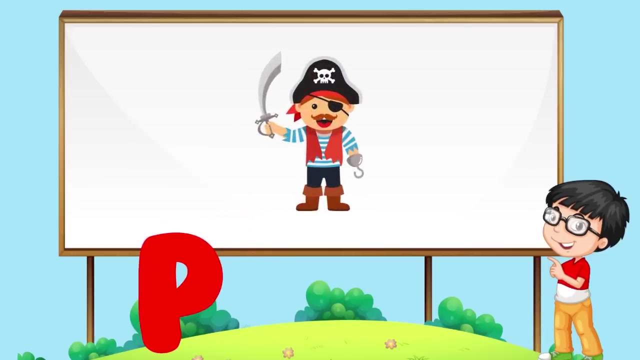 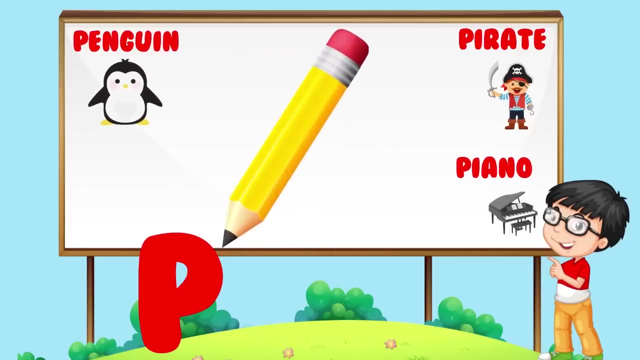 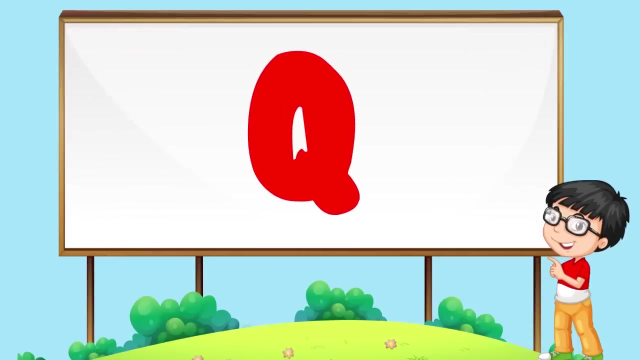 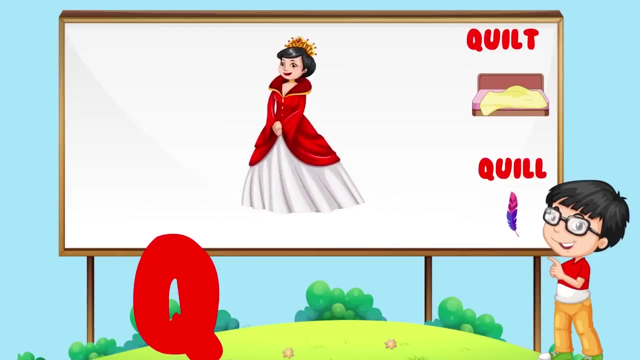 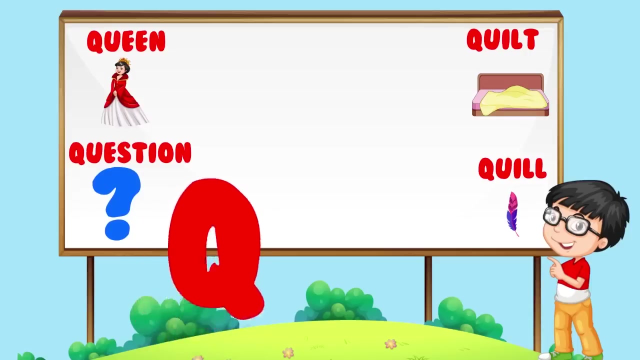 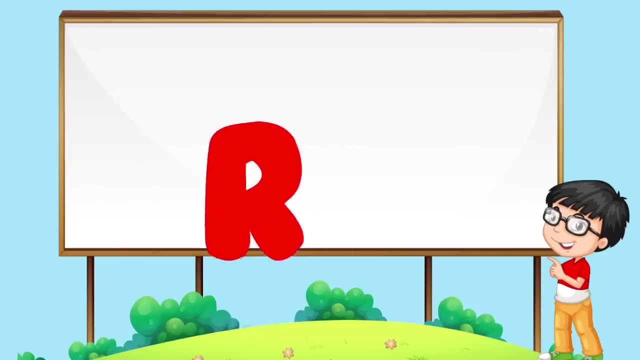 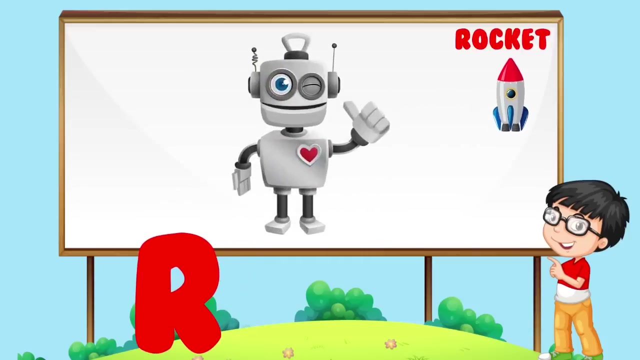 O for Ostrich, O for Oil. O for Octopus, O for Oct. O for Oat. P for Pirate. P for Piano. P for Penguin, P for Pencil. Q for Clip. Q for Queen. Q for Question. R for Rocket. R for Robot. R for Rainbow, R for Rabbit. 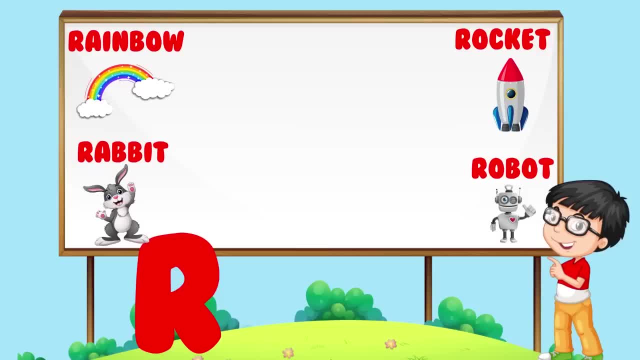 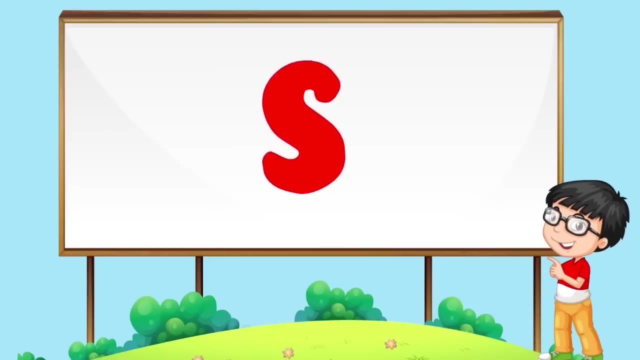 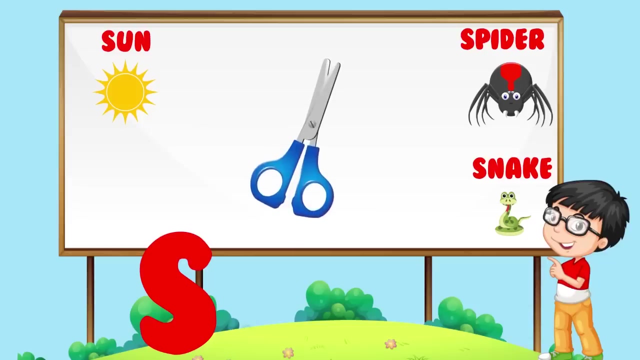 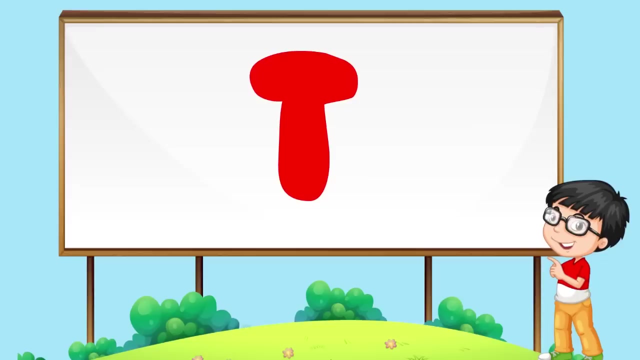 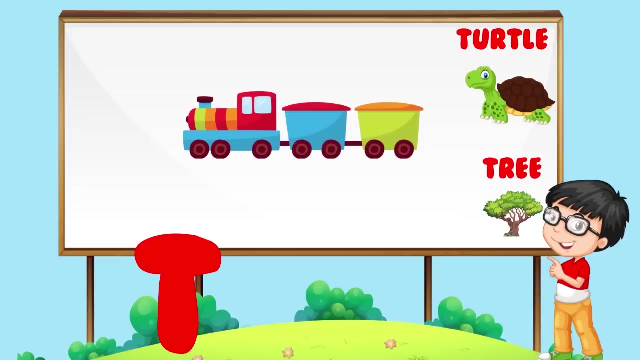 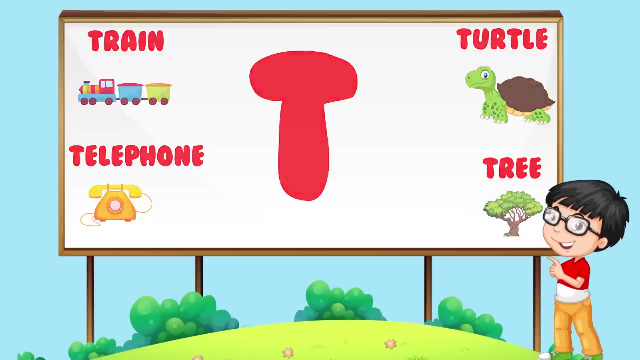 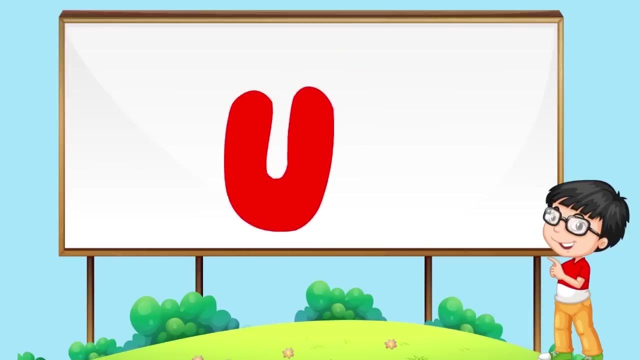 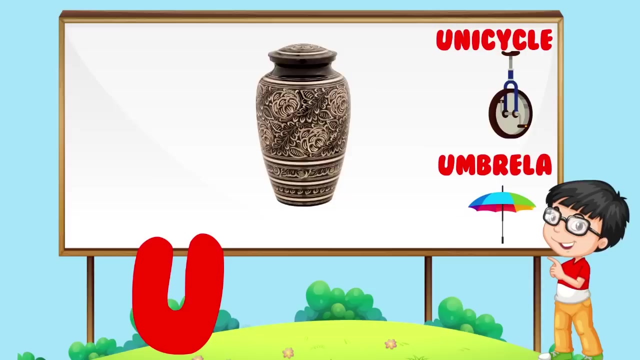 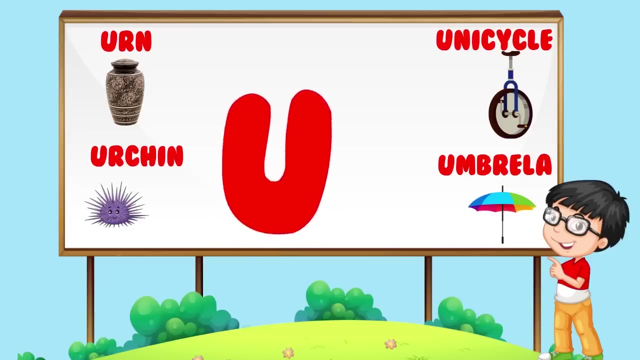 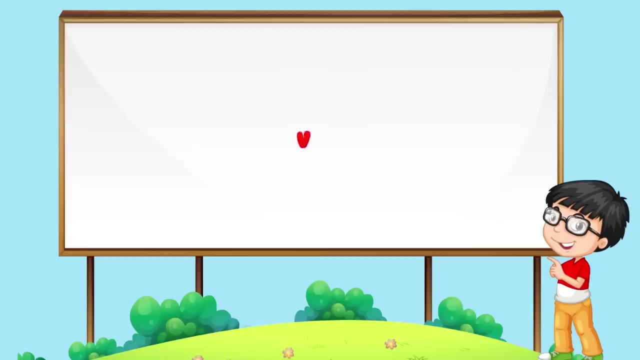 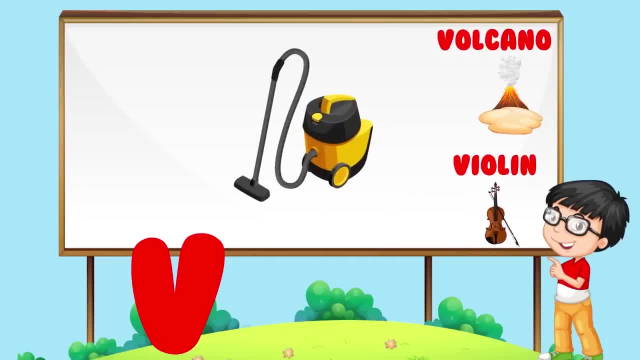 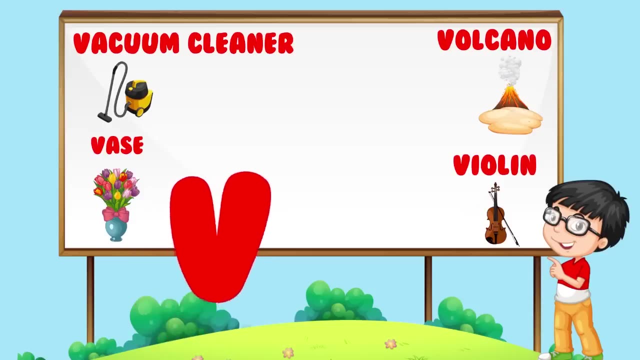 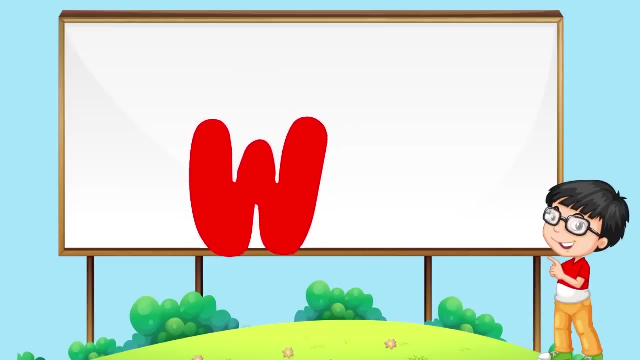 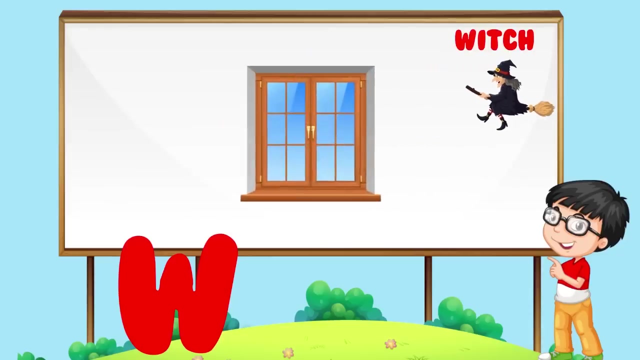 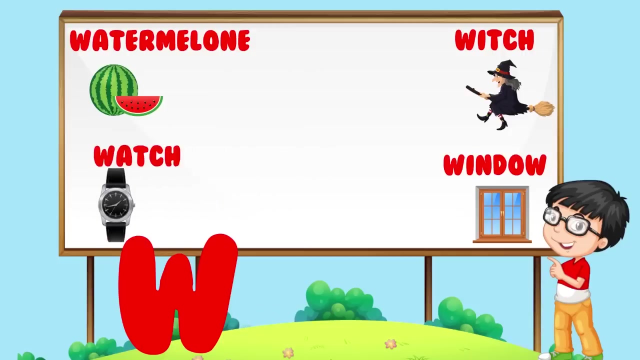 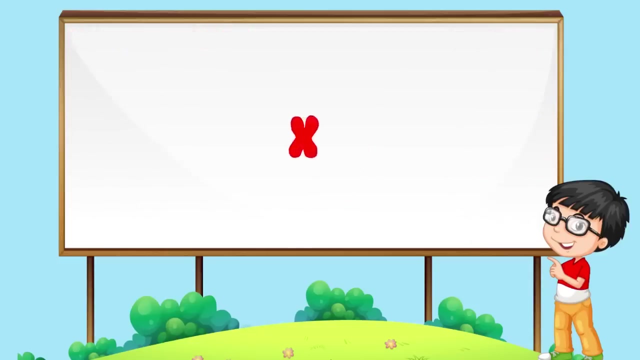 V4 vacuum cleaner, V4 was W4 which W4 window, W4 watermelon, W4 watch, X4 fox, X4 box, X4 box, X4 six, Y4 yo-yo, Y4 yogurt, Y4 play on, Y4 Z4 zipper, Z4 zebra. 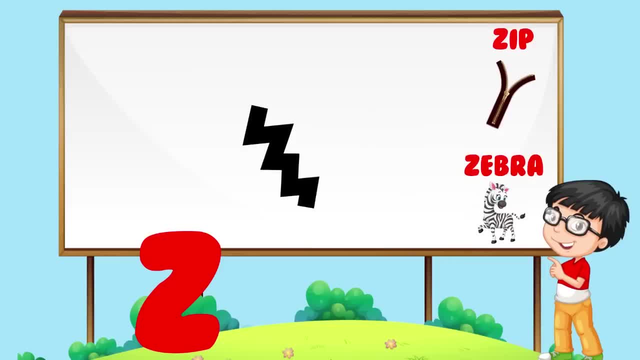 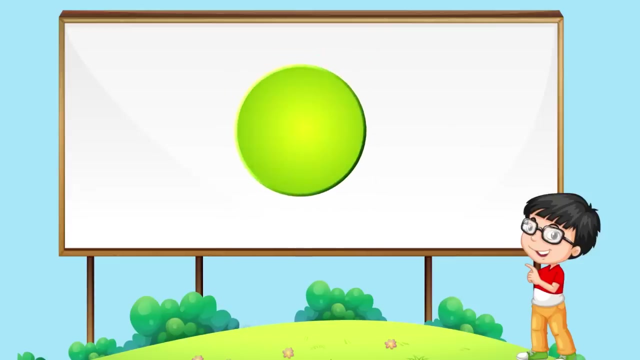 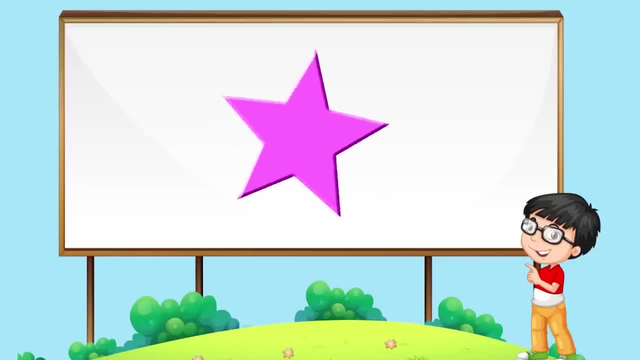 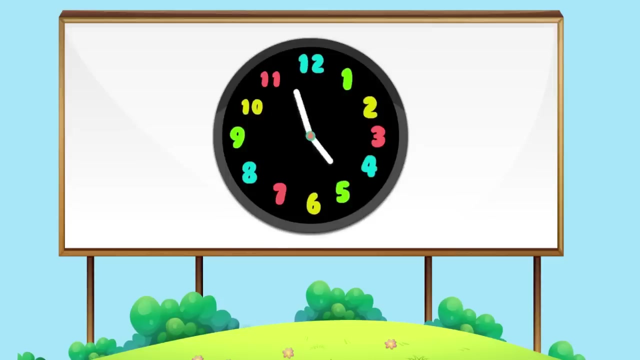 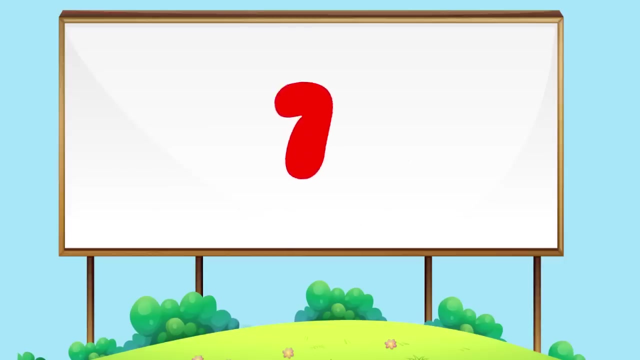 Z4 star, X4 star, Z4 star, Z4 star, Z4 star. A red heart. One, One, Two, Two, Three, Four, Three, Four, Four, Five, Five, Six, Six, Seven, Seven, Eight. 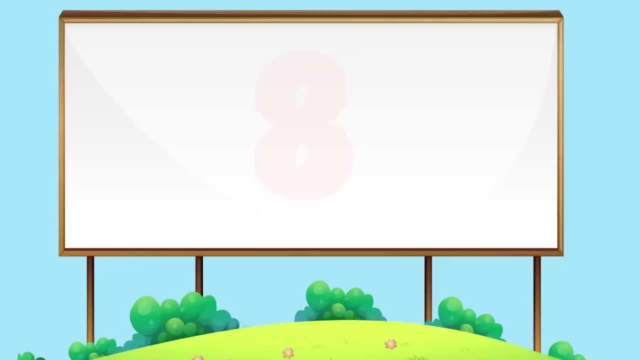 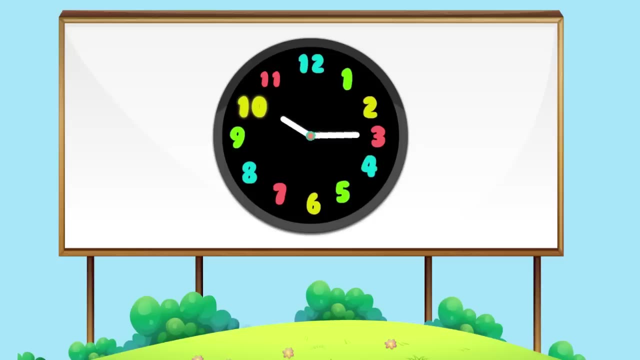 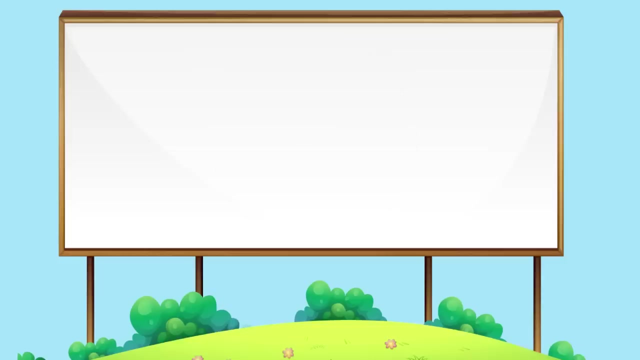 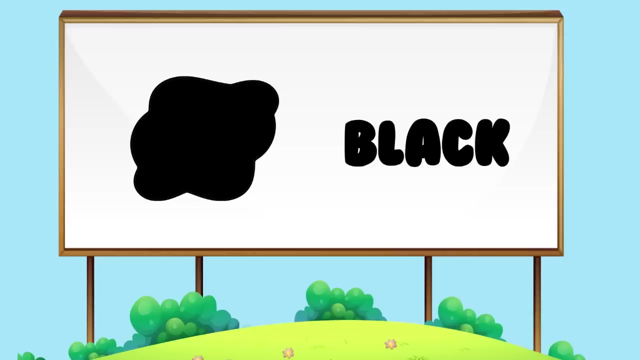 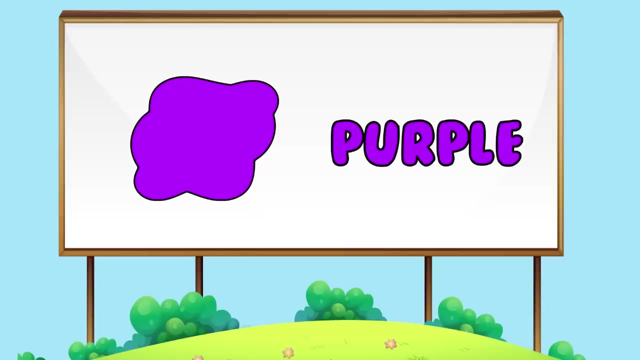 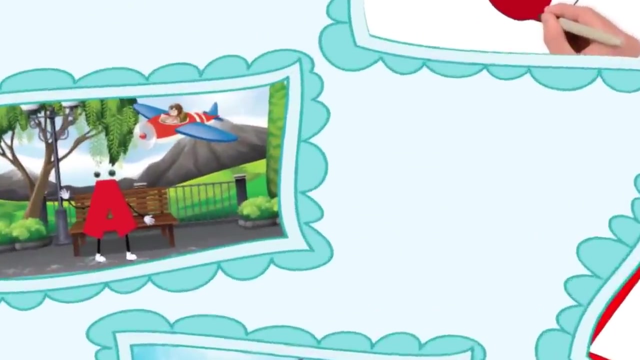 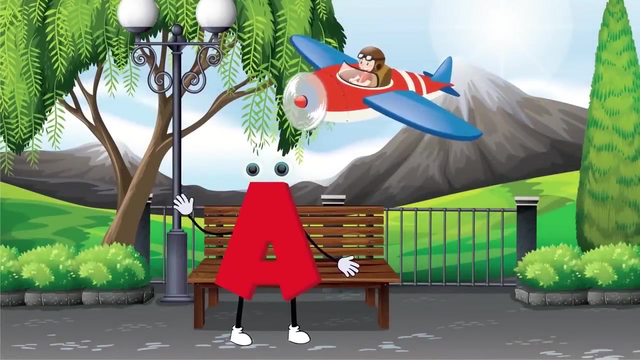 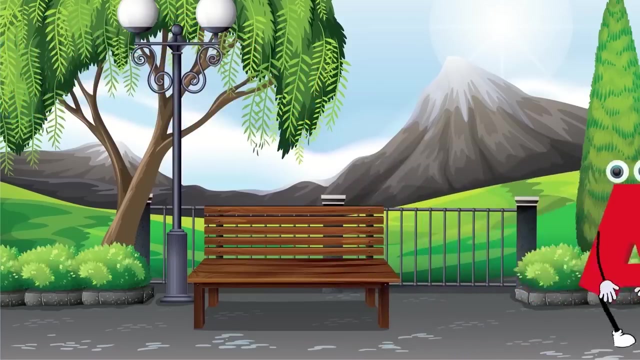 Eight, Nine, Nine, Nine, Ten, Ten, Eleven, Eleven, Twelve, Twelve Red, Green, Green, Blue, Yellow, Pink, Black, Purple, Brown, White, Orange. A for Aeroplane: Off we go B. B for Balls. 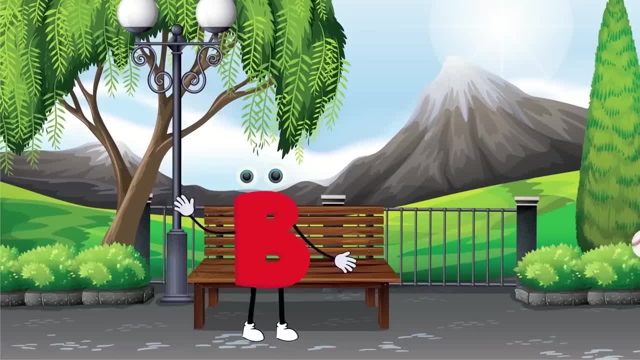 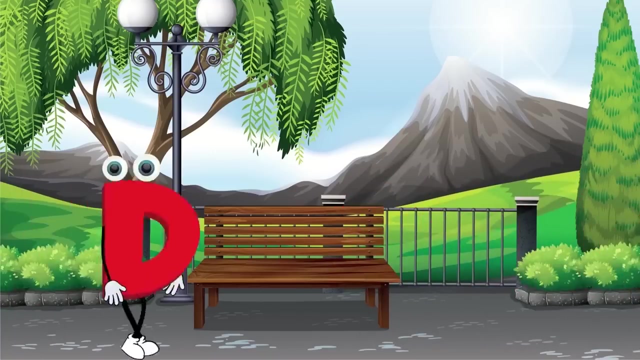 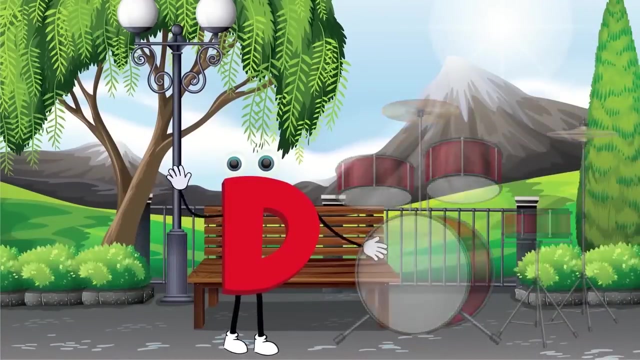 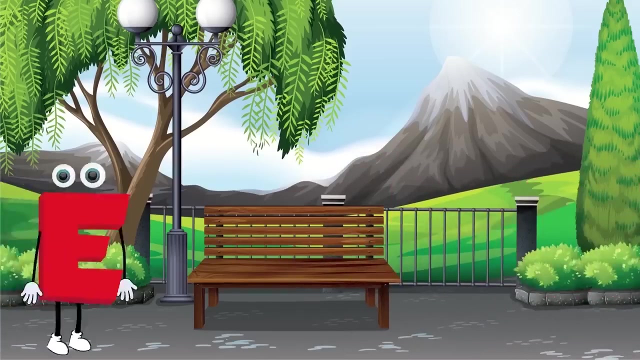 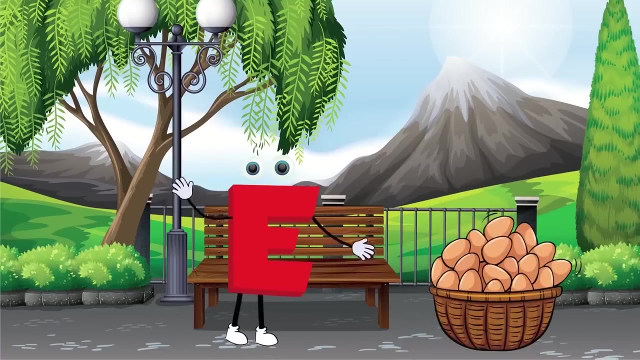 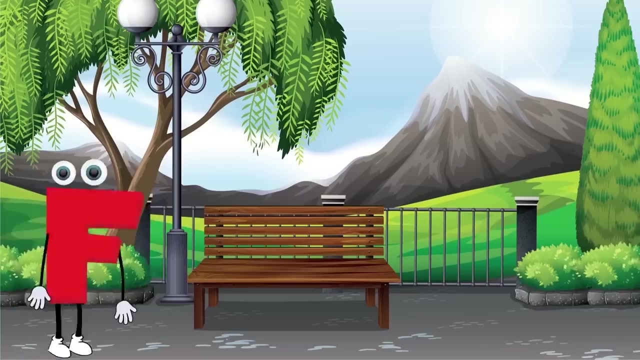 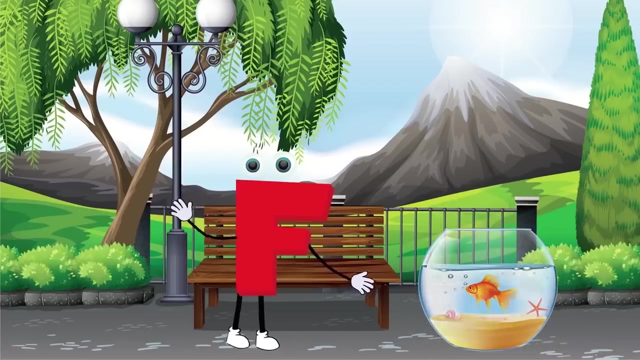 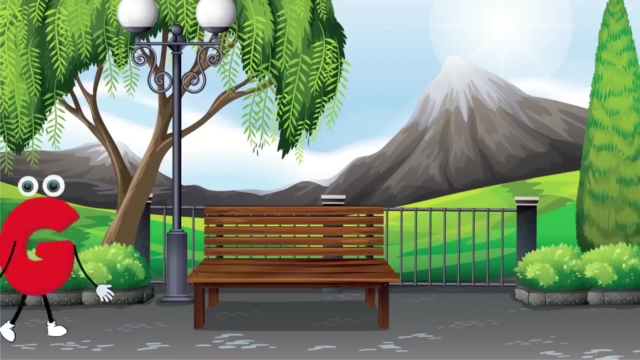 B for Bike. C, C for Car- Wow, look at that. D, D for Drums- Boom, boom, boom. E. E for Eggs- Wow, look at that, a basket full of eggs. F, F for Fish- Wow, look at that fish. G, G for Guitar. 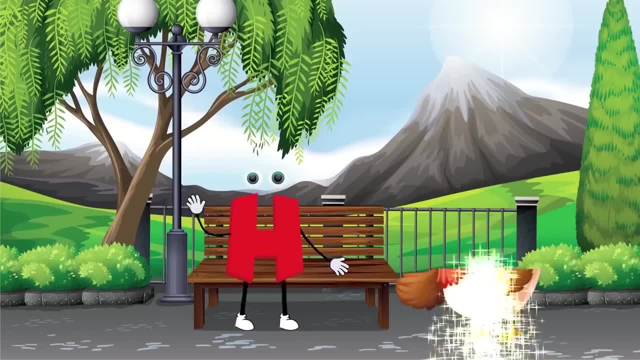 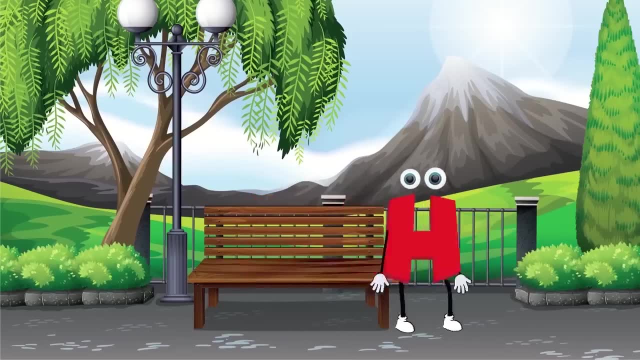 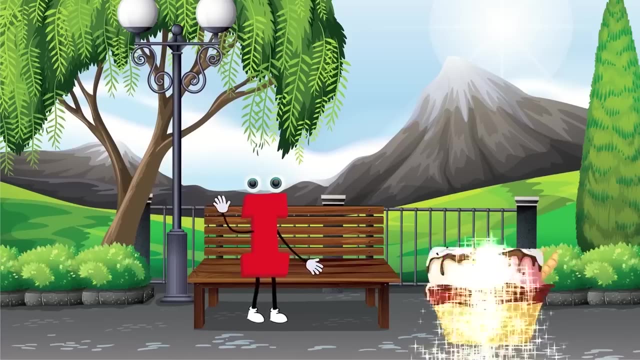 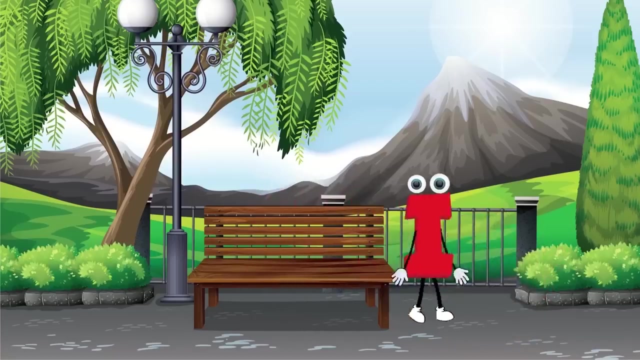 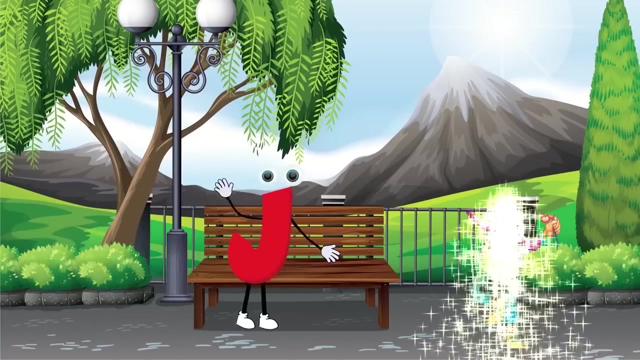 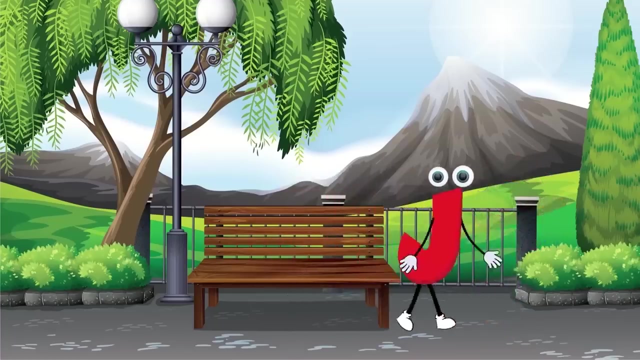 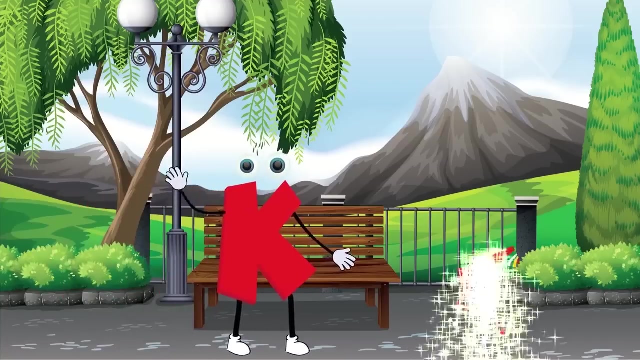 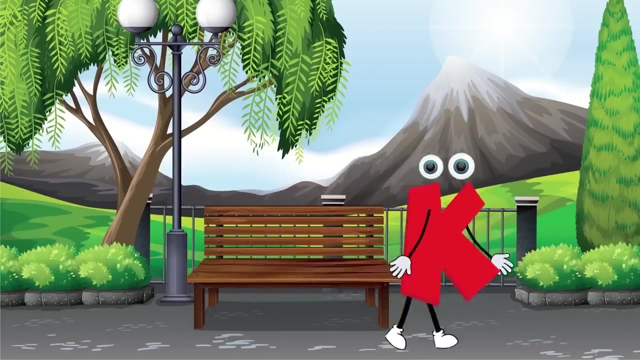 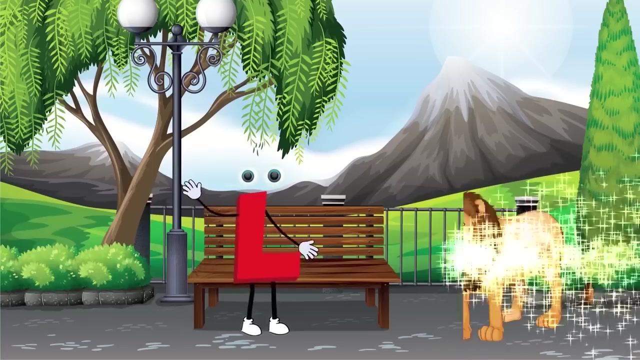 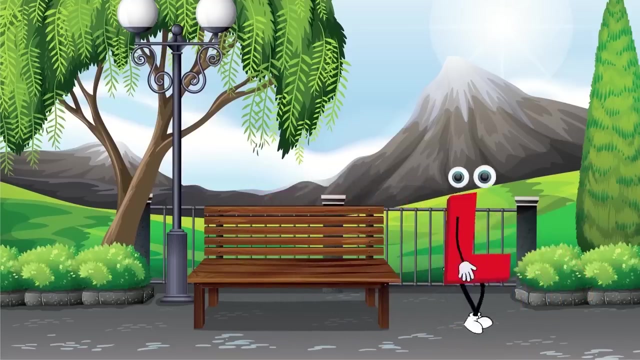 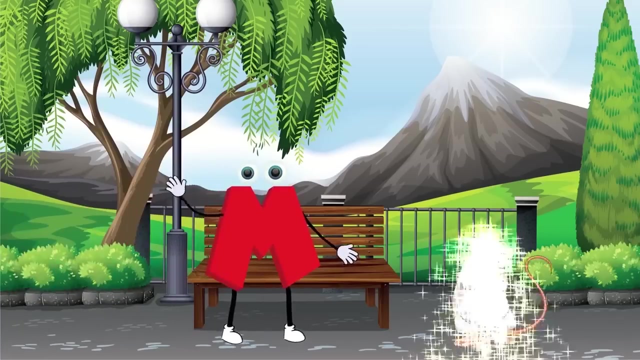 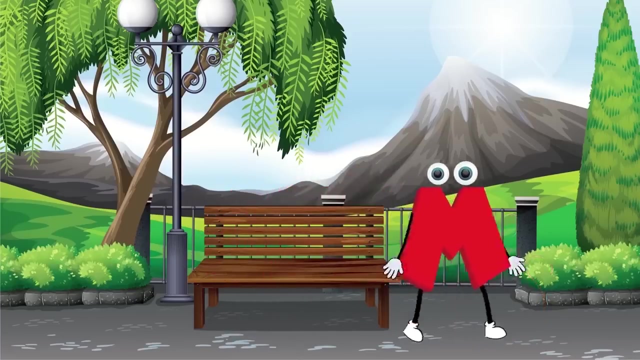 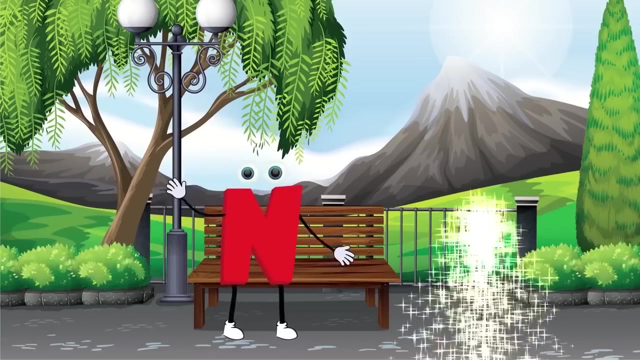 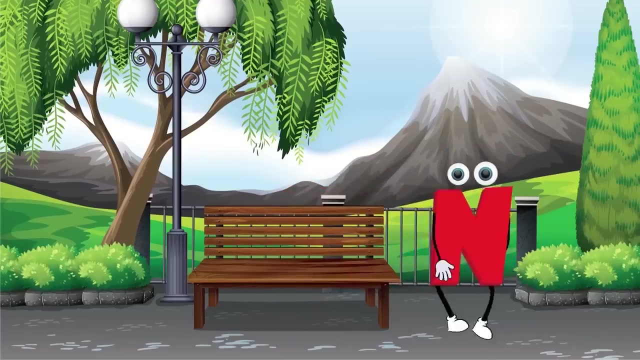 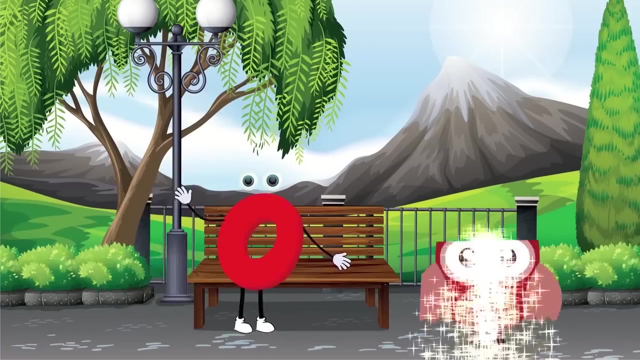 H H for Hen I I for Ice Cream, Mmm, yummy. J J J K K for Kite. Wow, look at that Kite. J J J J L L for Lion, L for Lion, Ro M M for Mouse, N O O for Owl. 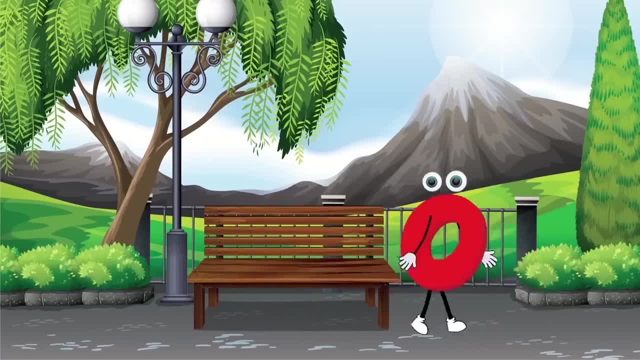 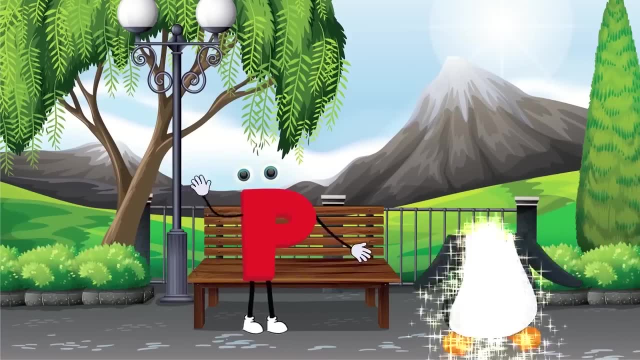 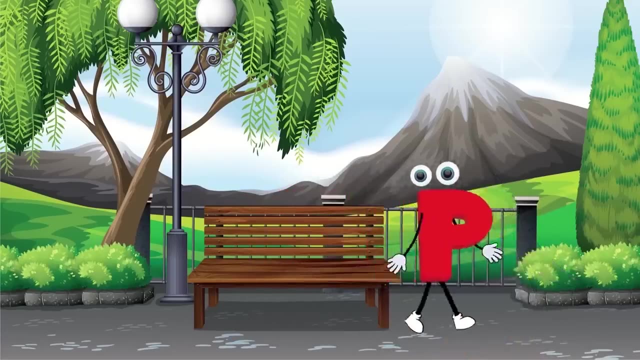 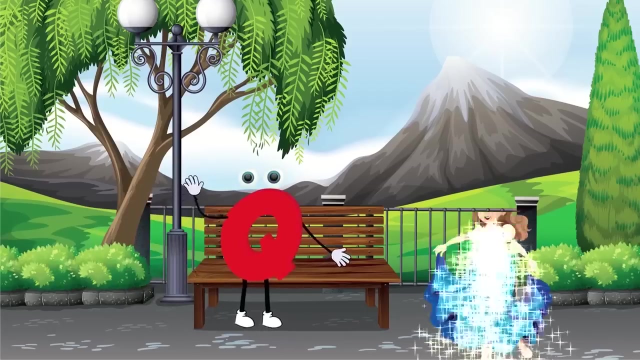 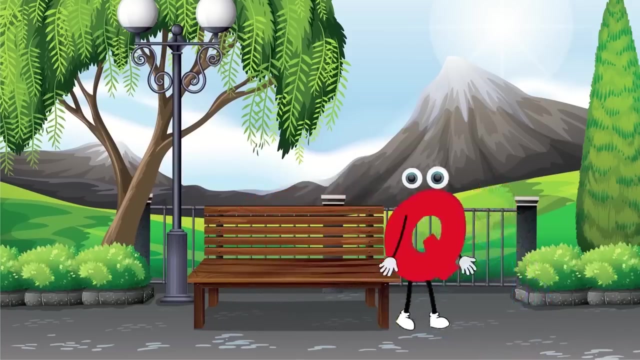 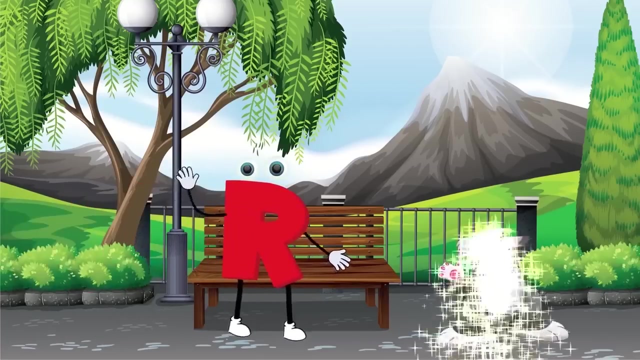 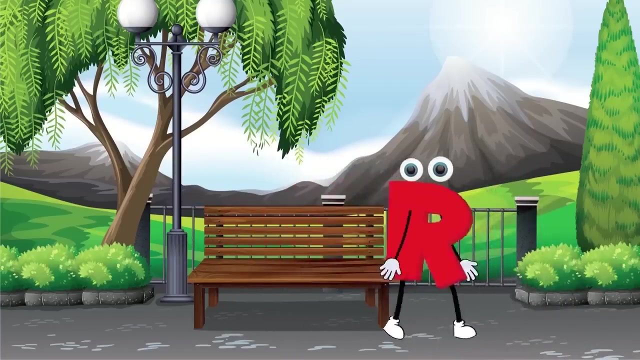 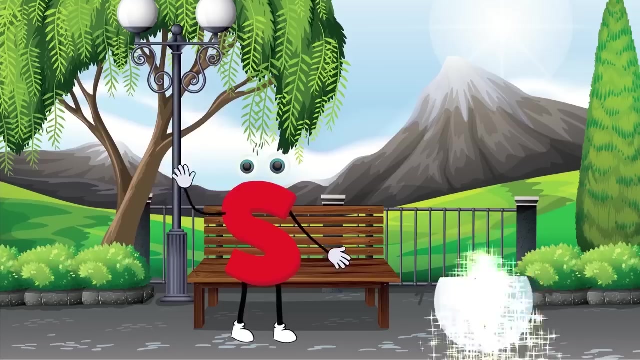 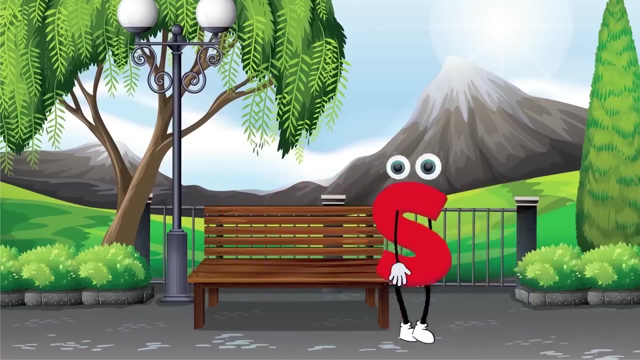 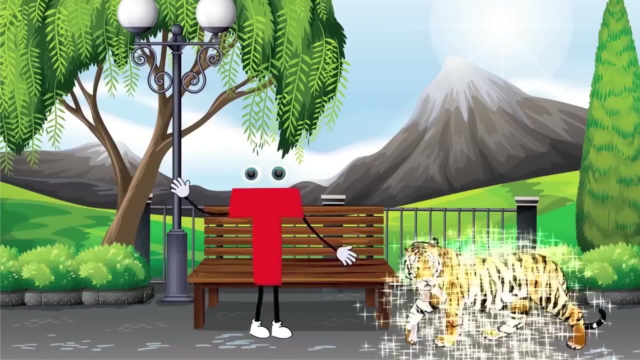 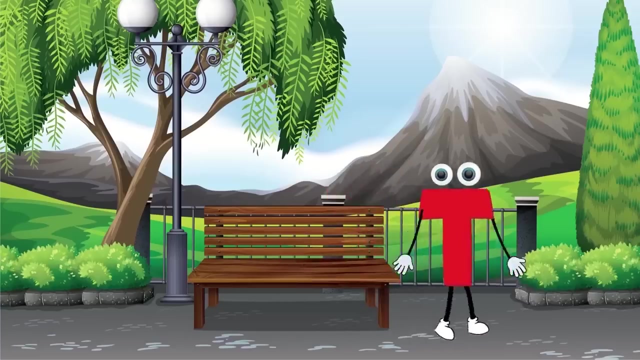 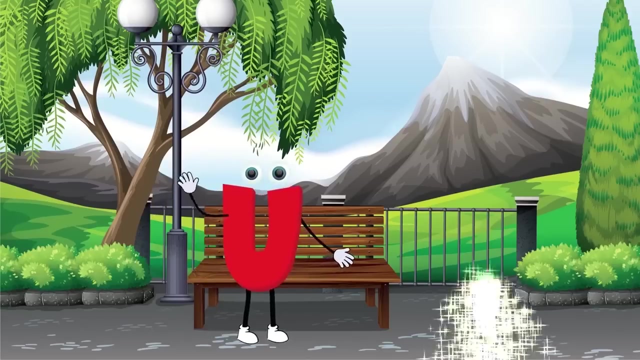 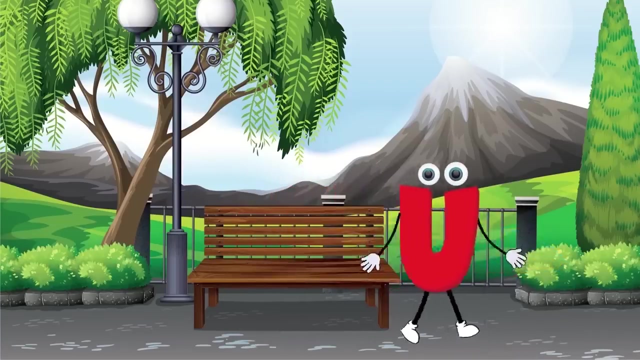 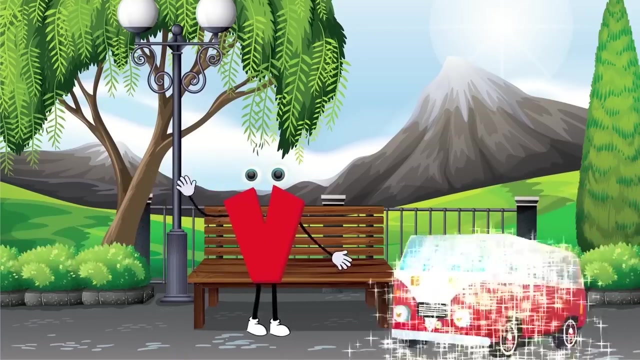 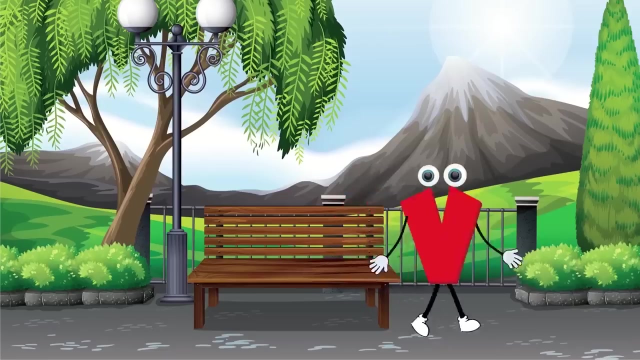 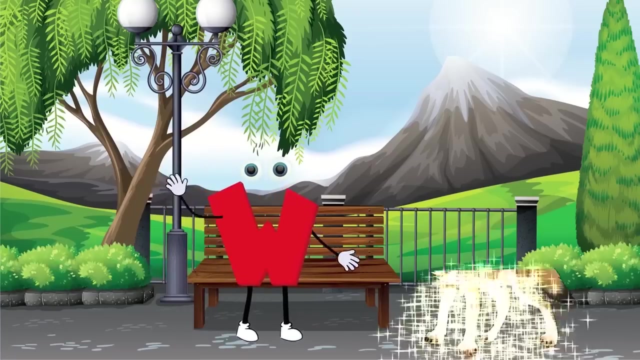 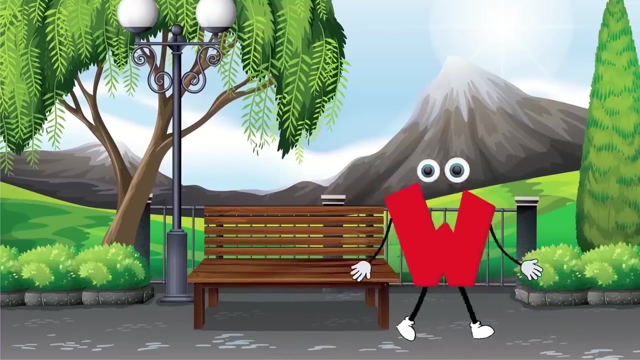 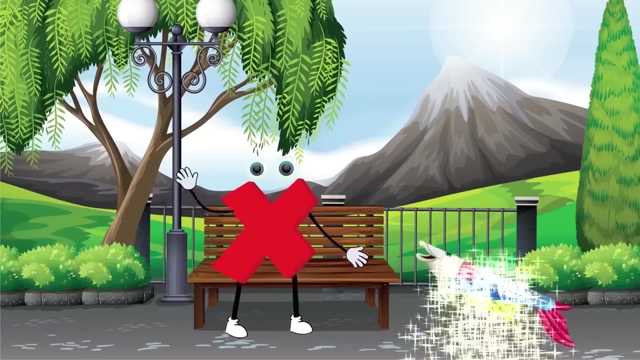 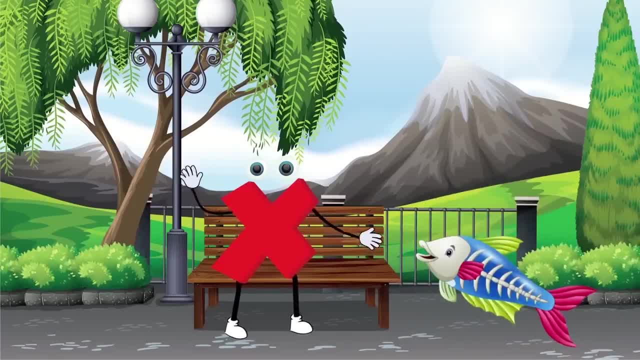 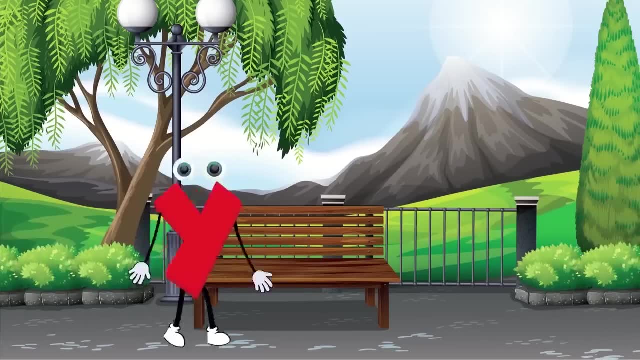 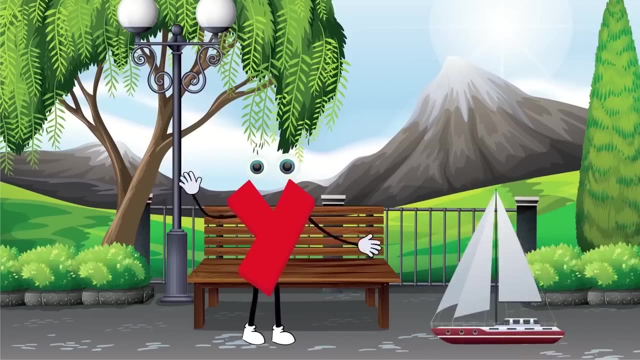 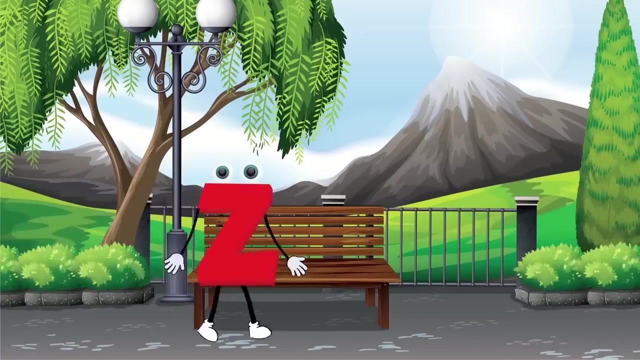 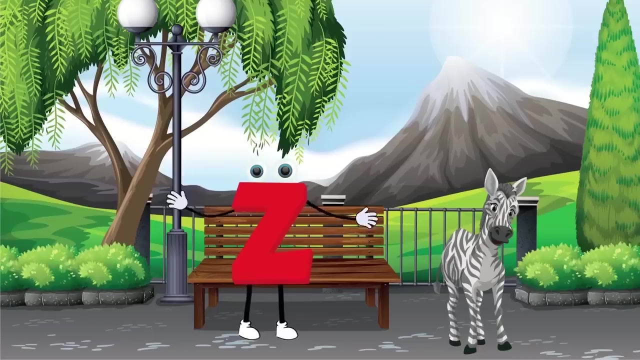 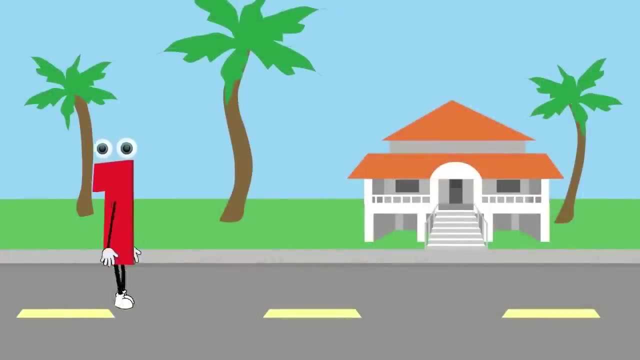 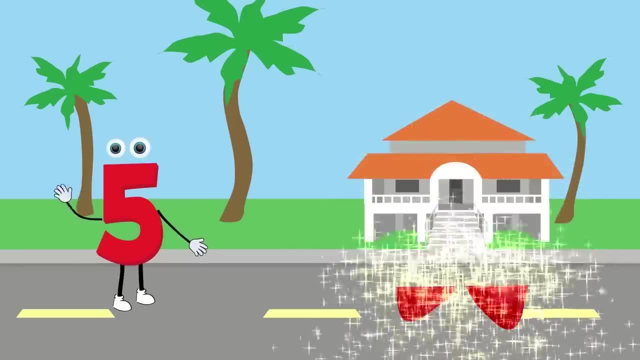 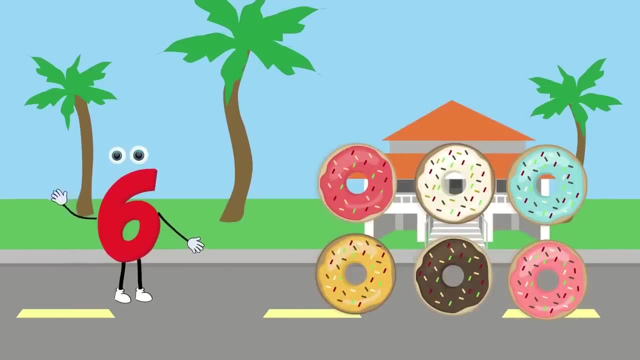 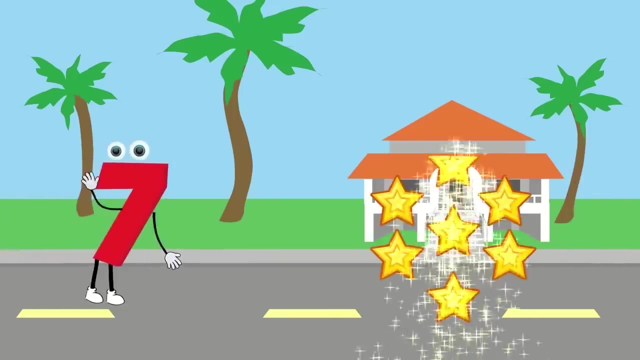 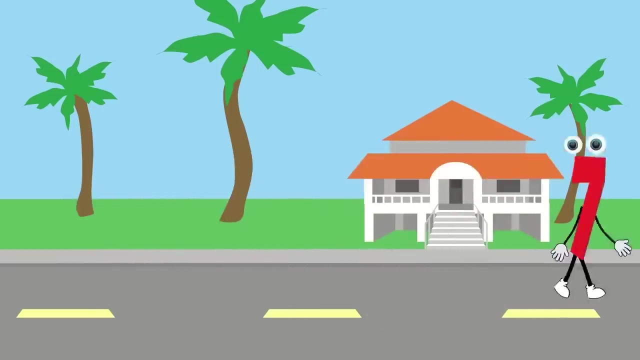 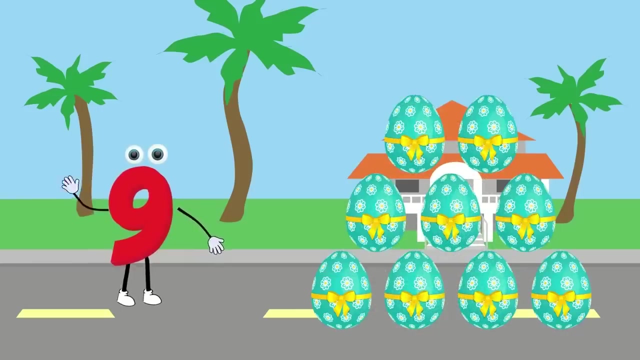 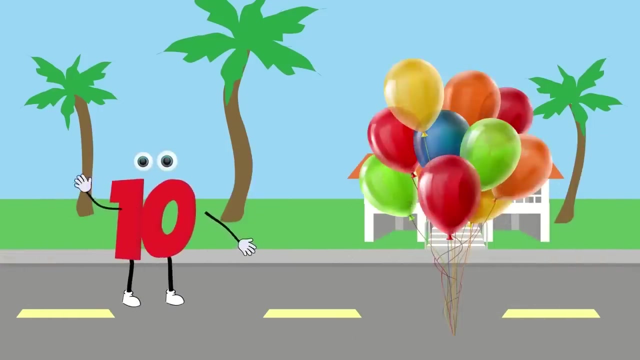 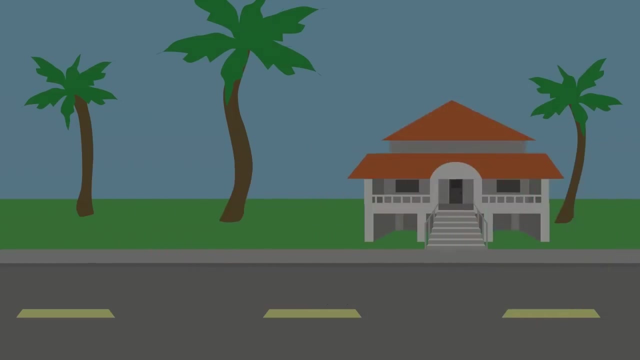 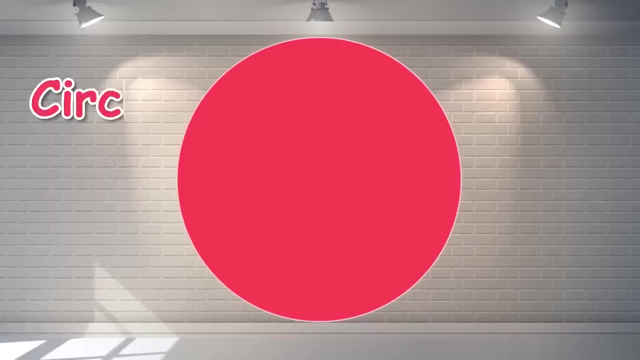 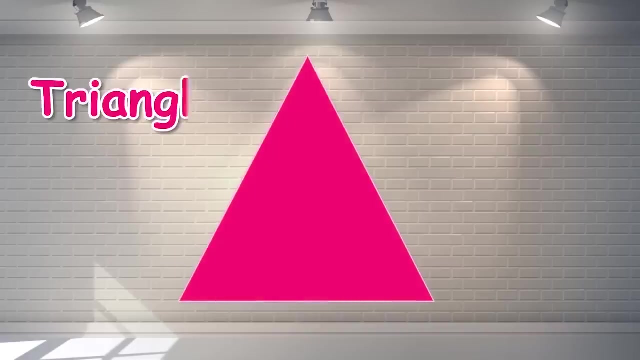 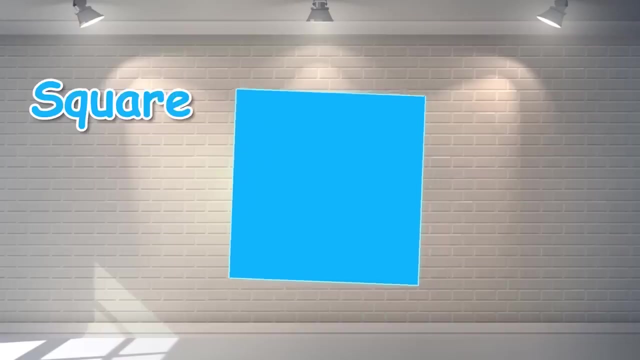 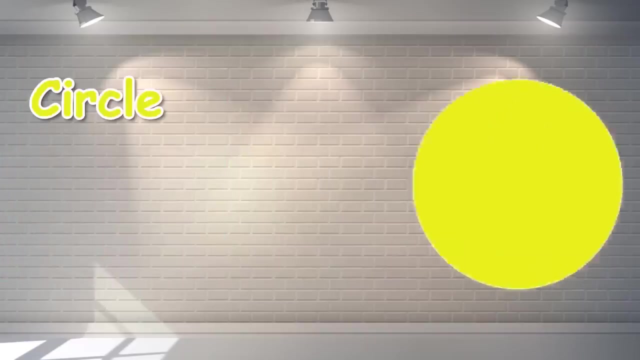 Five, five strawberries. Six, six donuts. Seven, seven stars. Eight eight candles. Nine, nine eggs. Ten, ten balloons, Ten, ten stars. Wow, look at that Circle, A red circle. Wow, A pink triangle, A blue square. Wow, look at that, A yellow circle. 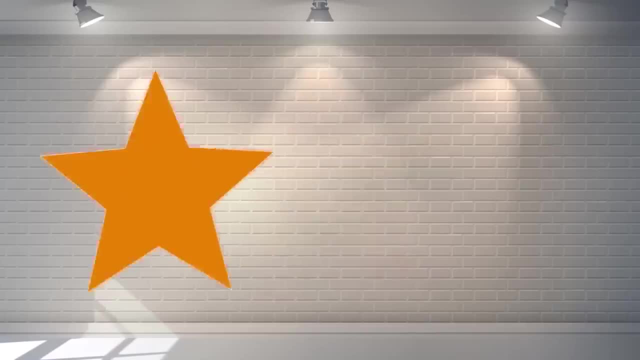 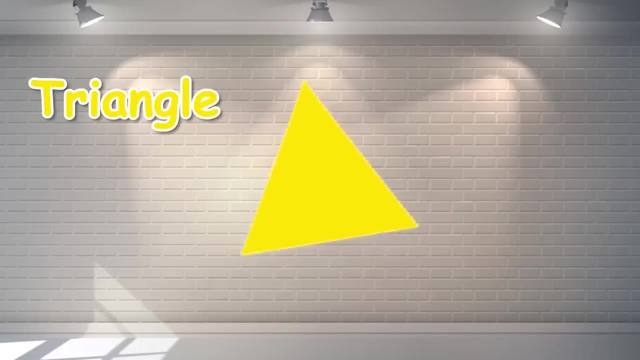 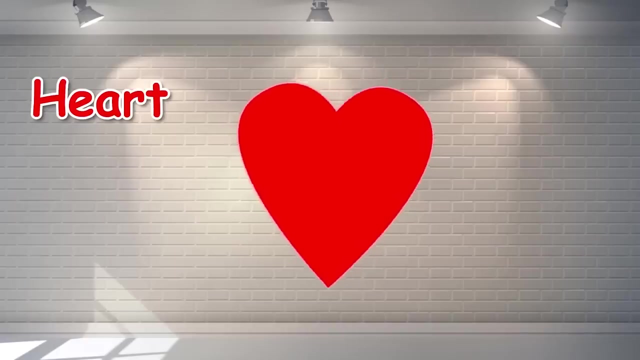 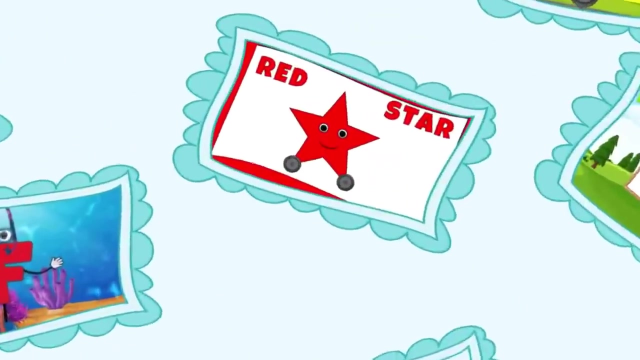 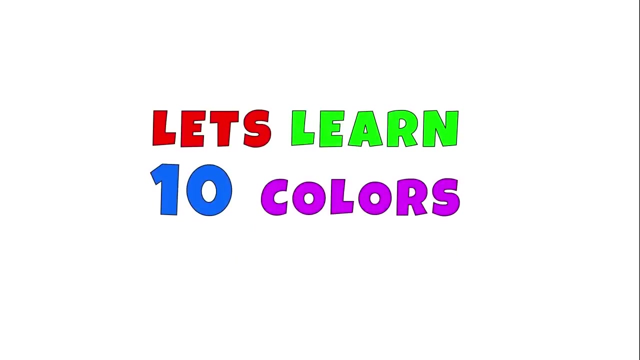 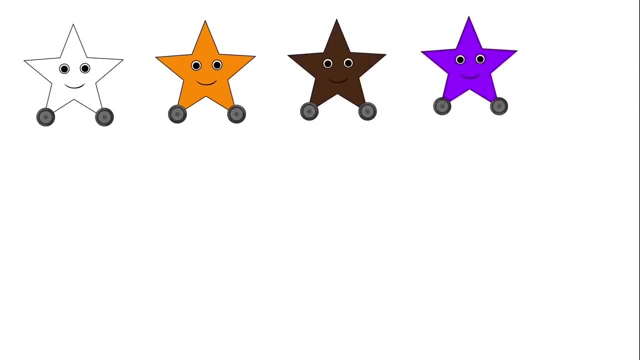 An orange star. Wow, look at that. A yellow triangle. Wow, look at that. A red heart. Red Heart, White, White, Orange, Brown, Brown, Purple, Pink, Green, Black, Yellow, Blue, Red. Now let's try it backward: Red, Blue, Yellow. 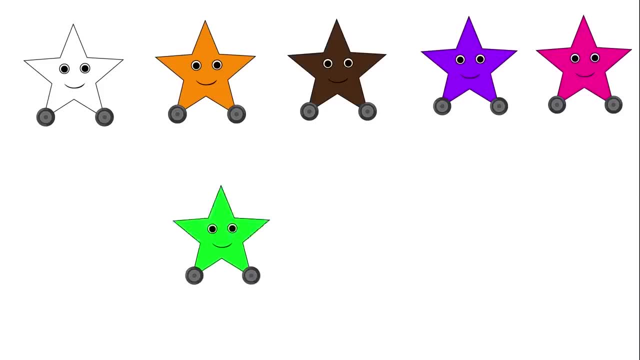 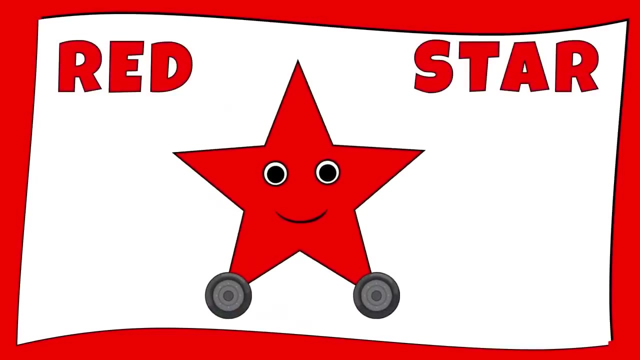 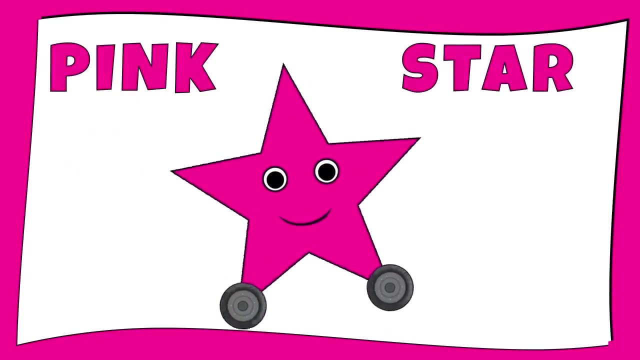 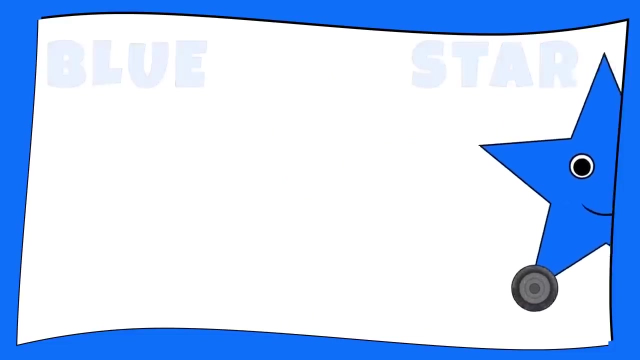 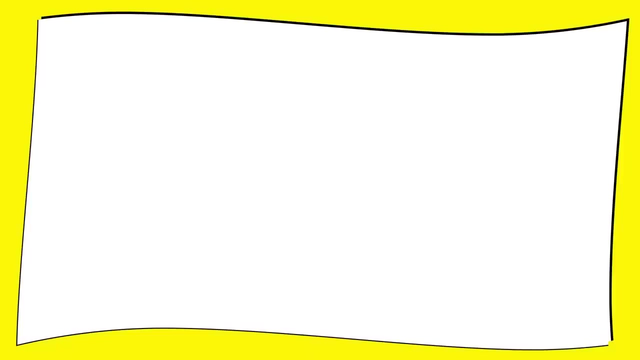 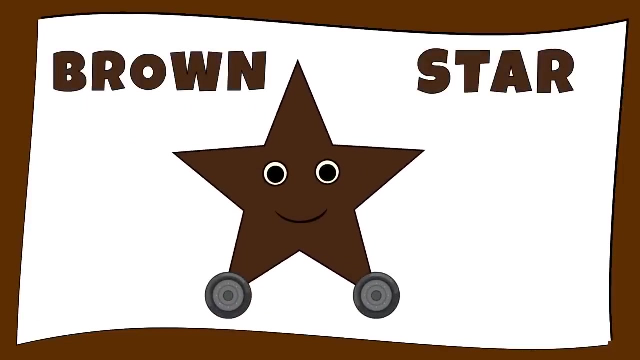 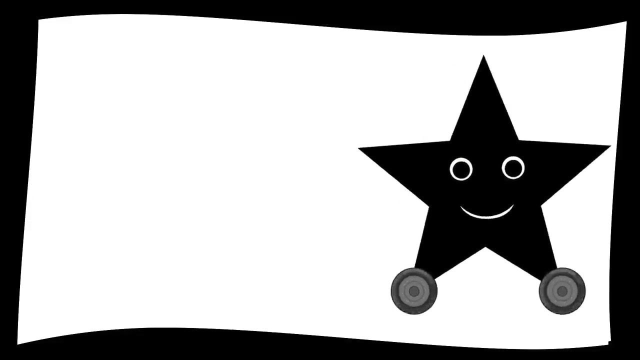 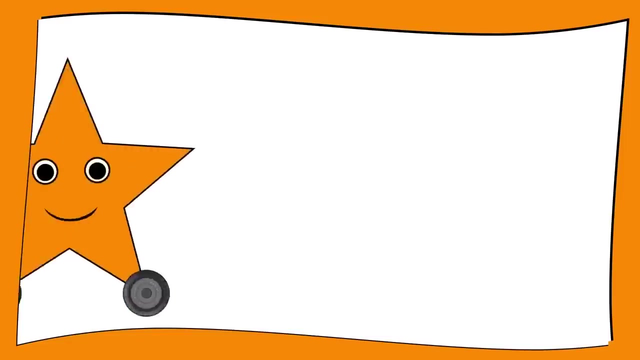 Black, Green, Pink, Purple, Brown, Orange, White, Red, Red, Pink, Pink, Blue, Blue, Green, Green, Green, Yellow, Yellow, White, White, Brown, Brown, Black, Black, Blue, Purple, Purple, Orange, Orange. 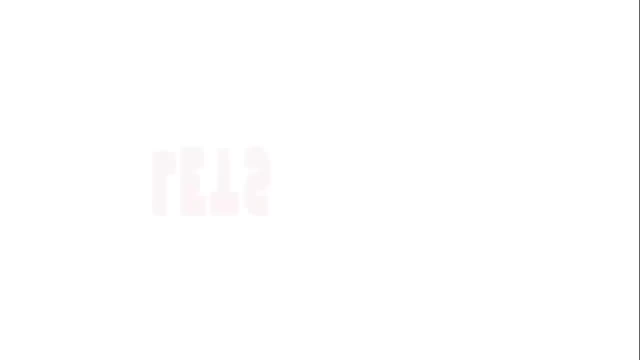 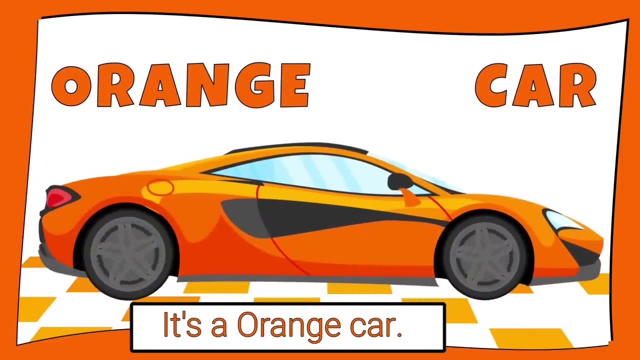 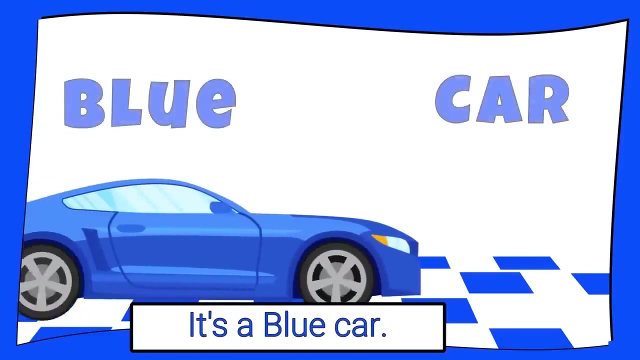 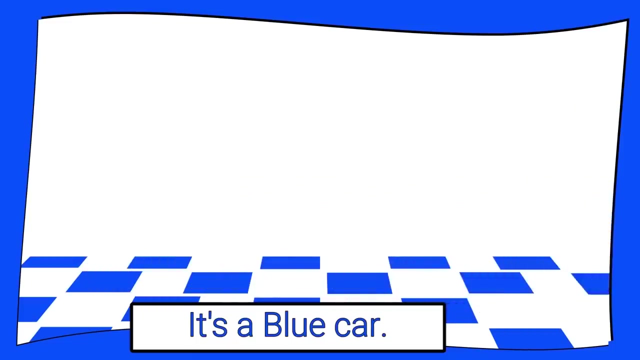 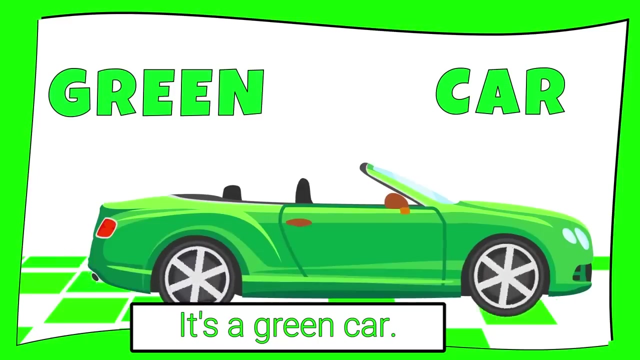 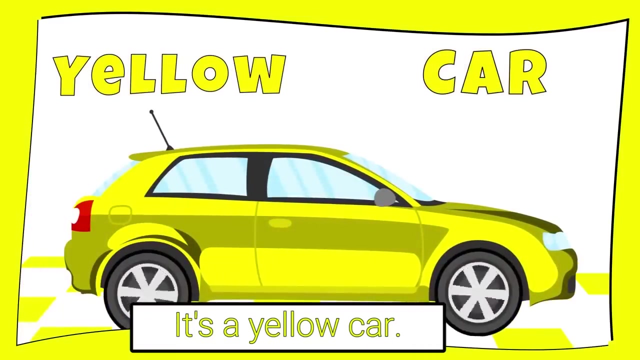 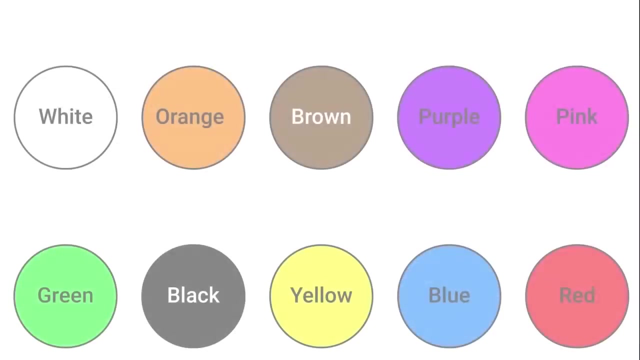 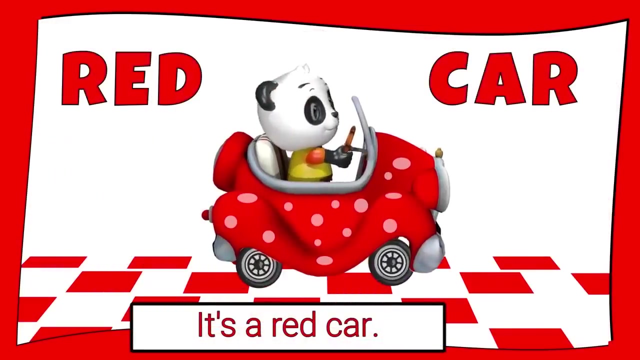 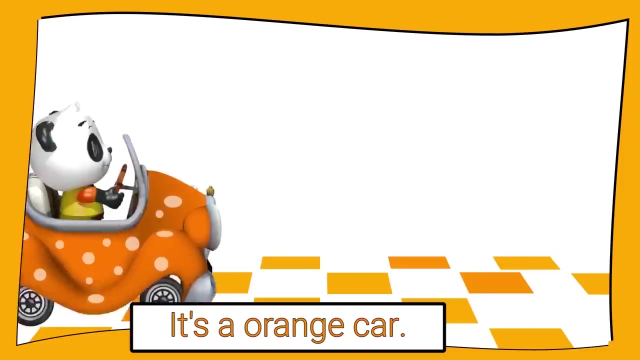 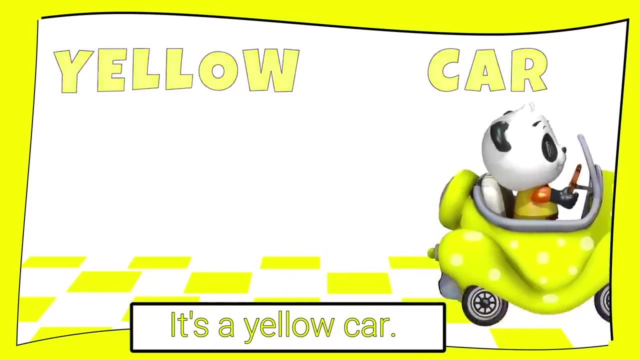 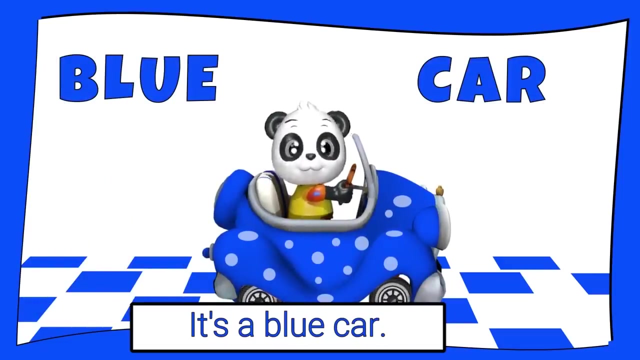 It's an orange car, It's a blue car, It's a green car, It's a yellow car, It's a red car, It's a orange car, It's a yellow car, It's a blue car, It's a blue car. 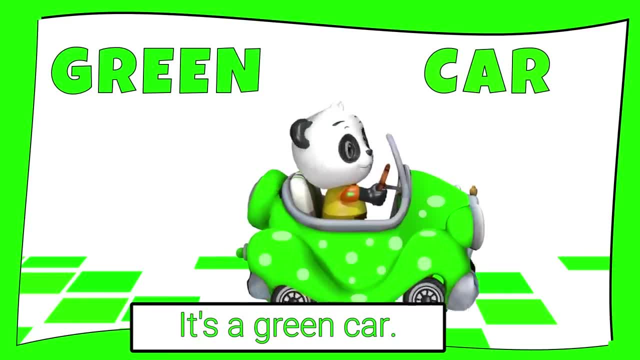 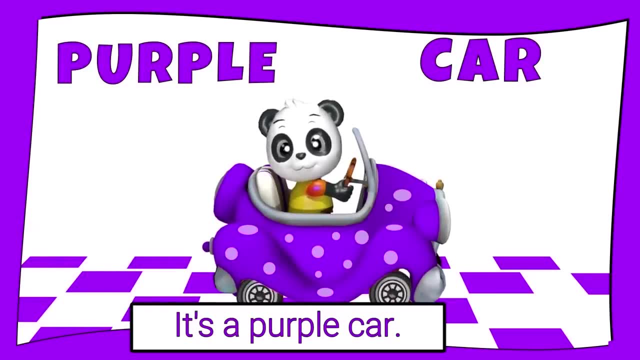 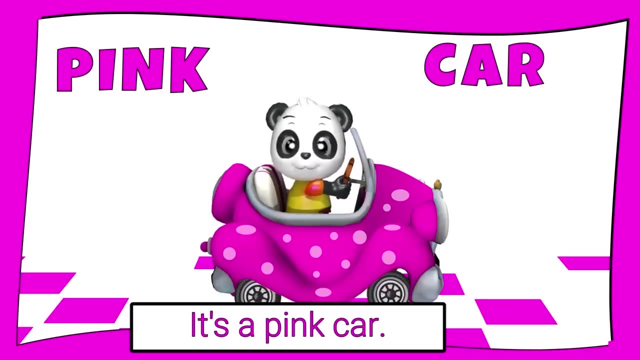 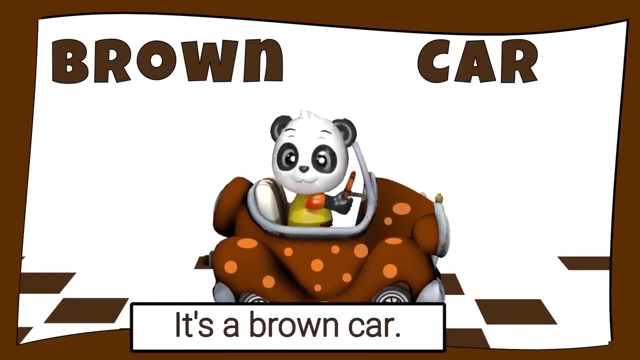 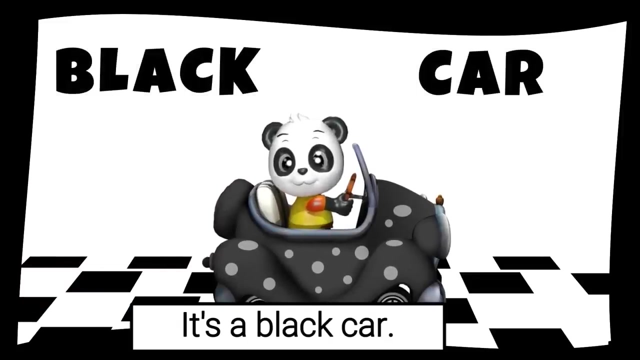 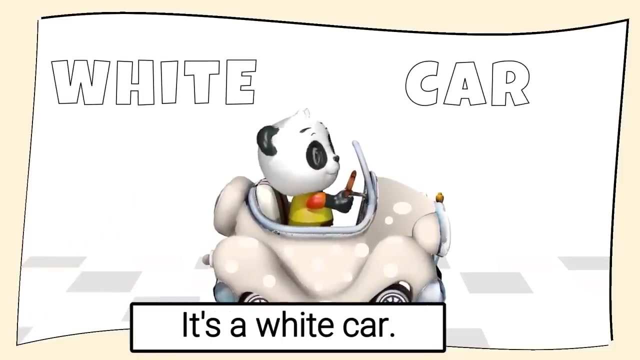 It's a blue car, It's a green car, It's a purple car, It's a pink car, It's a yellow car, It's a blue car, It's a brown car, It's a black car, It's a white car. 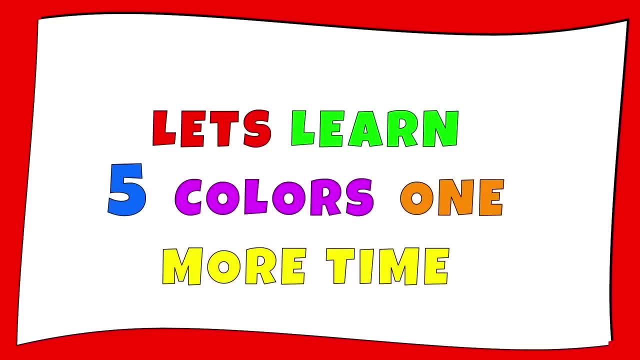 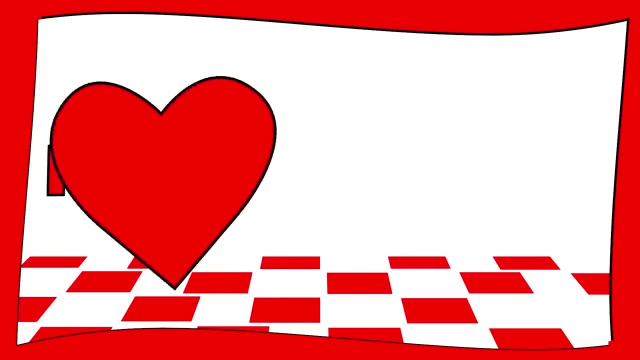 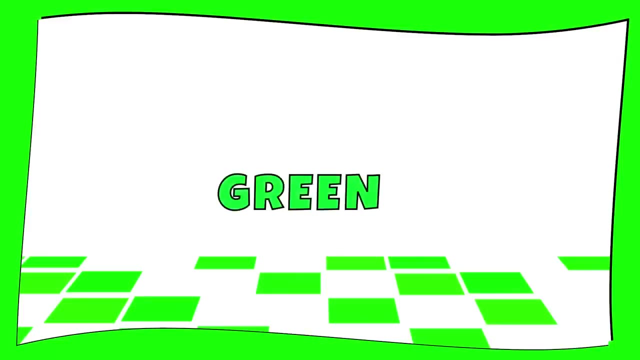 Red, red. the heart is red, Red red: the heart is red, red, red. Green, green. the pear is green, Green, green: the pear is green, green, green, Blue, blue. the balloon is blue. 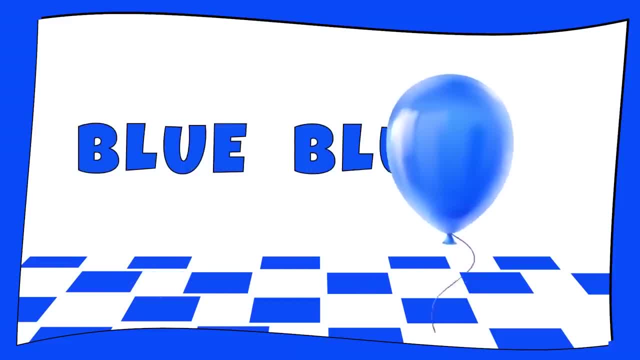 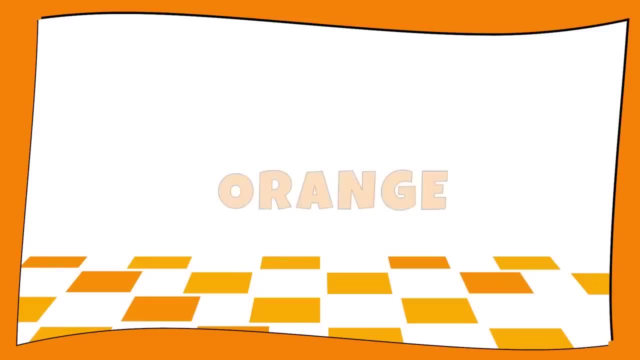 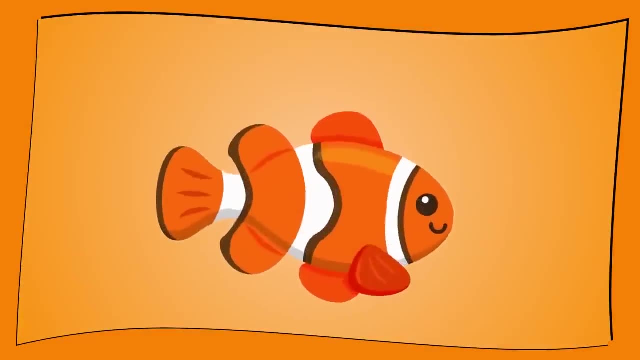 Blue blue. the balloon is blue, Blue blue: the balloon is blue, blue, blue. Orange, orange, orange. the fish is orange, Orange, orange. the fish is orange, orange, orange, Black, black. the cat is black. 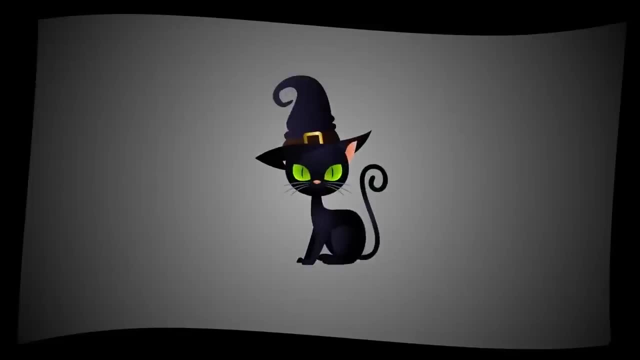 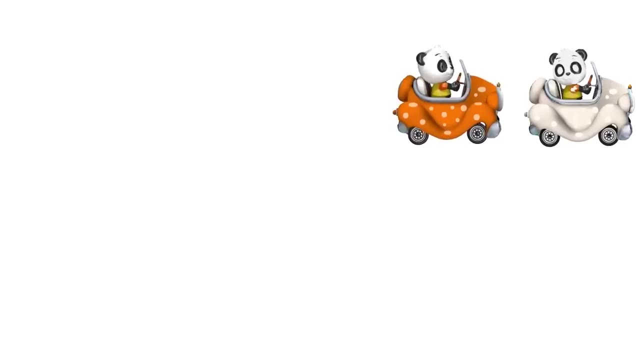 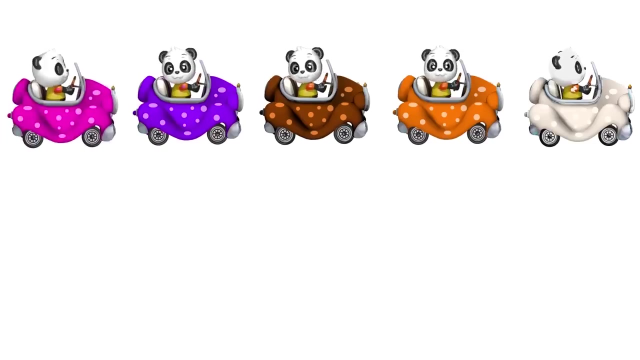 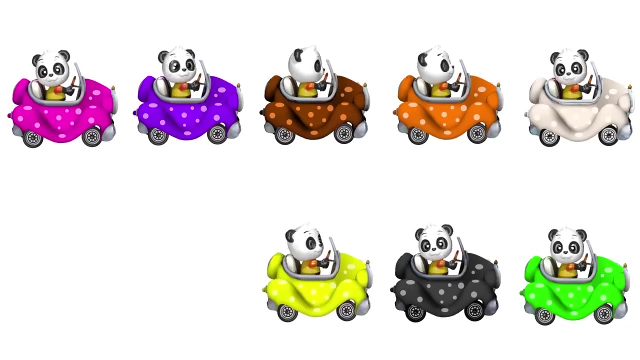 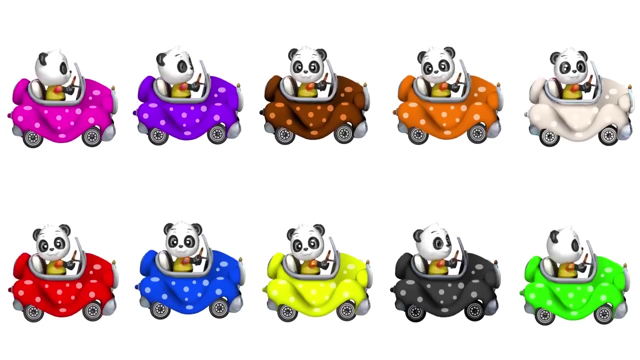 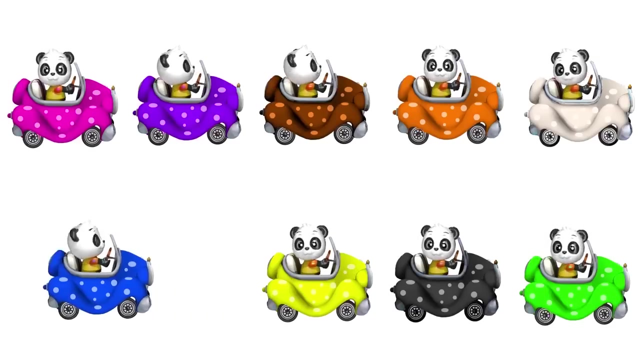 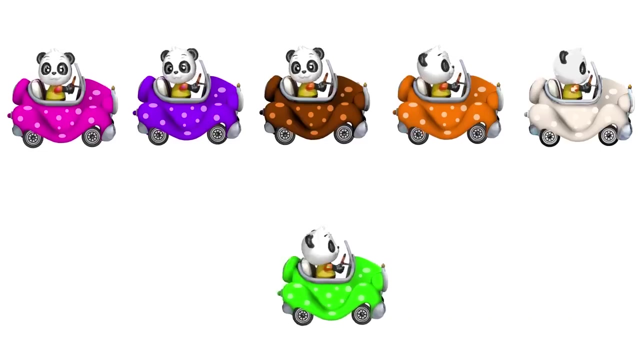 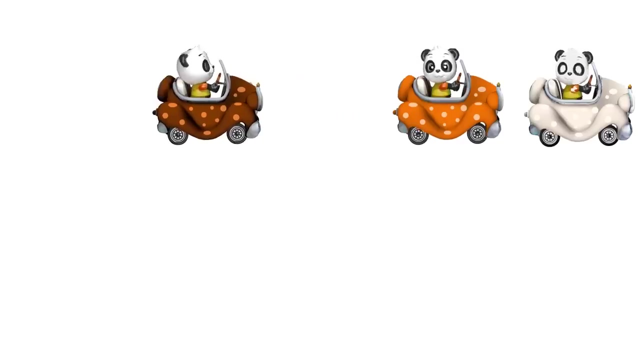 Black black. the cat is black. black. black, White, orange, brown, purple, pink, Green, black, yellow, blue, red. Now let's try it backwards: Blue, blue, yellow, black, green, pink, purple, brown, orange. 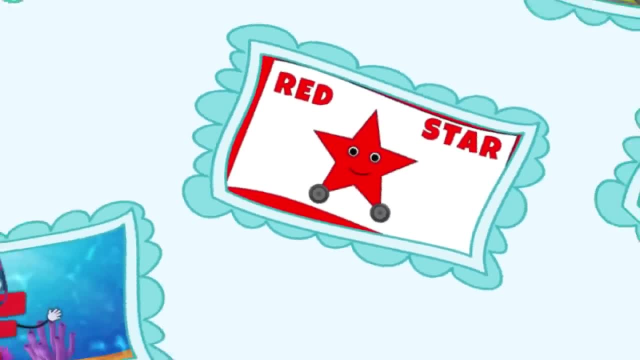 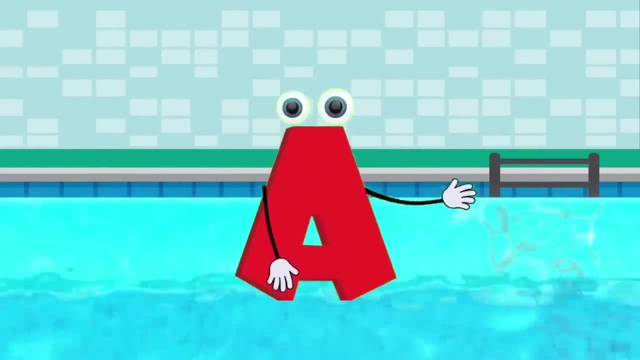 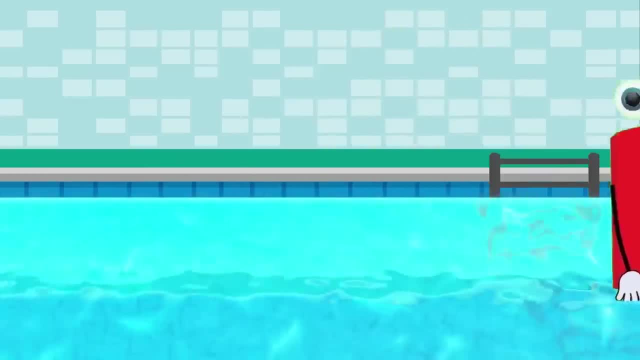 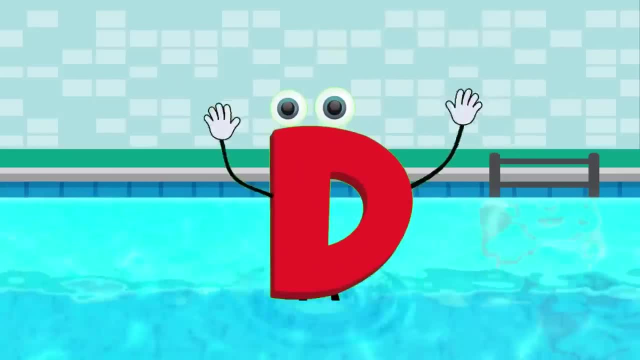 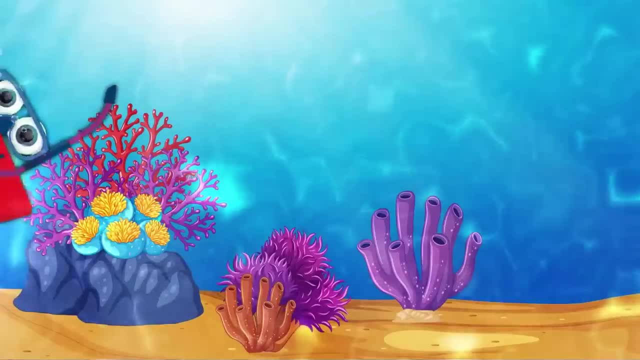 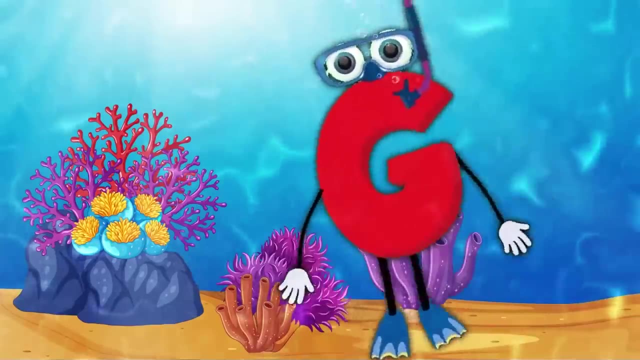 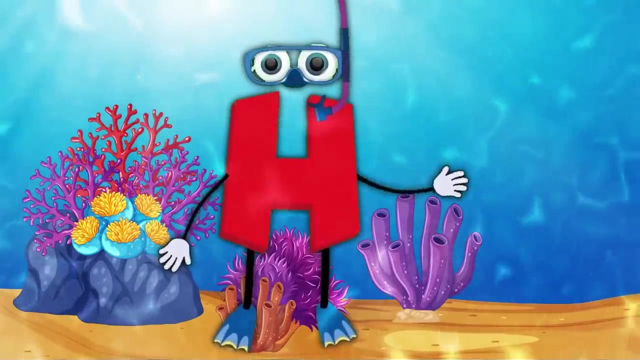 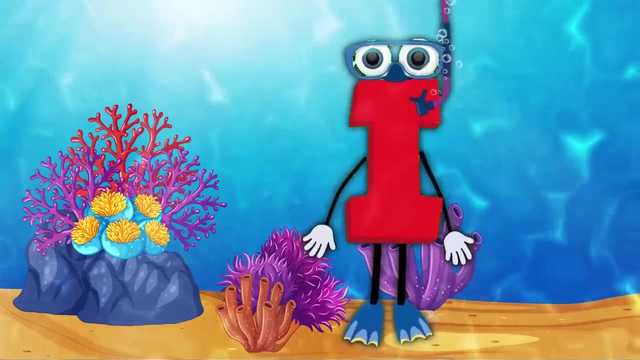 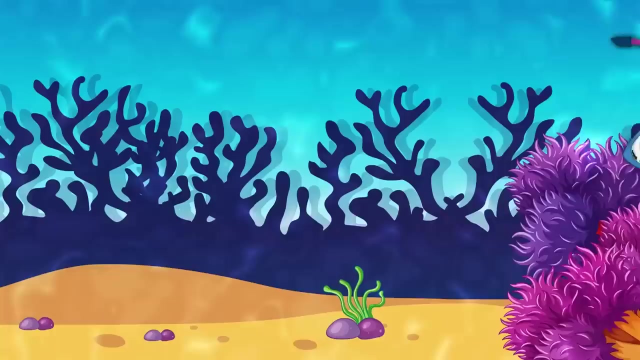 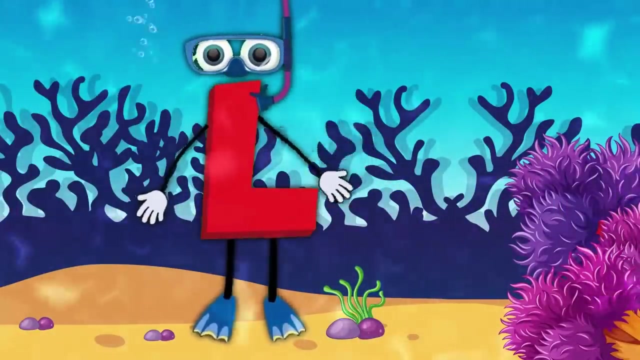 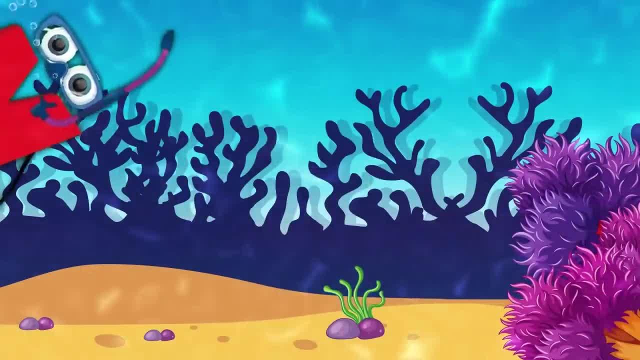 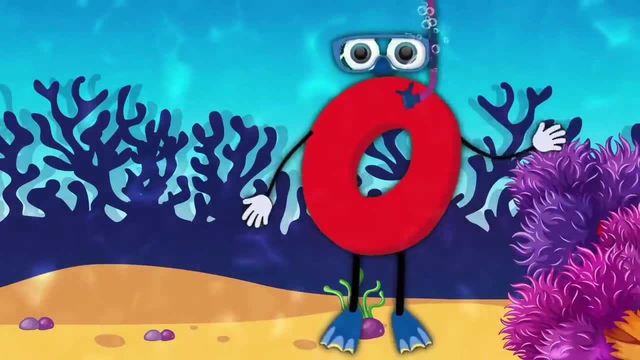 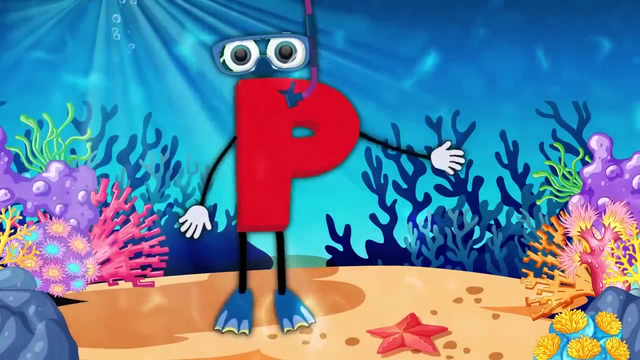 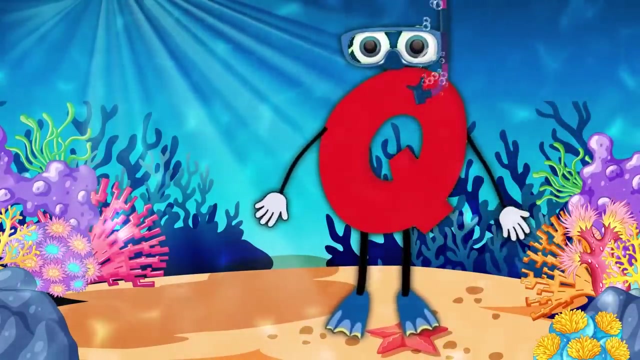 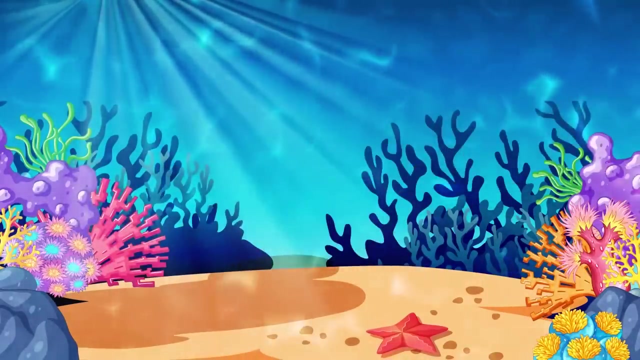 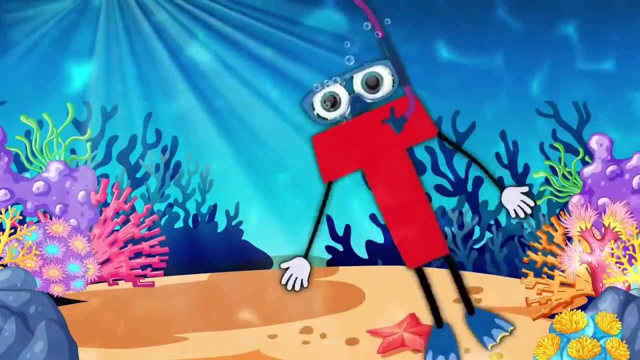 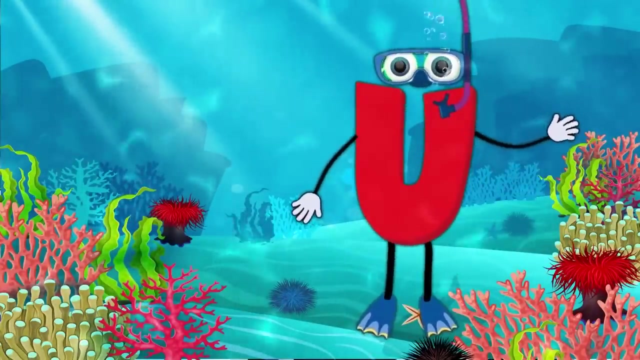 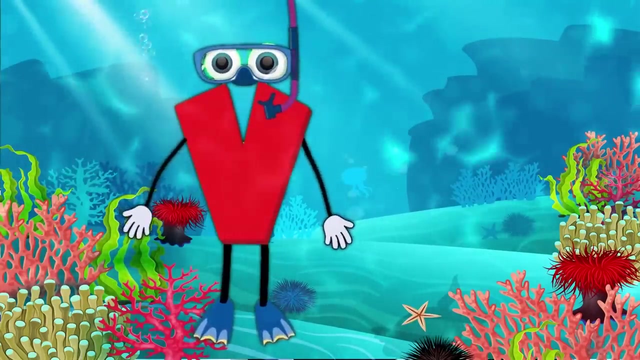 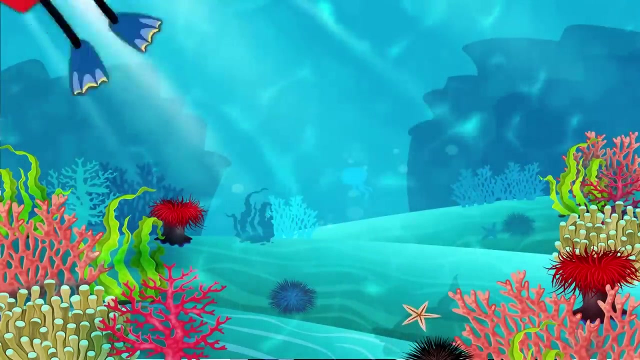 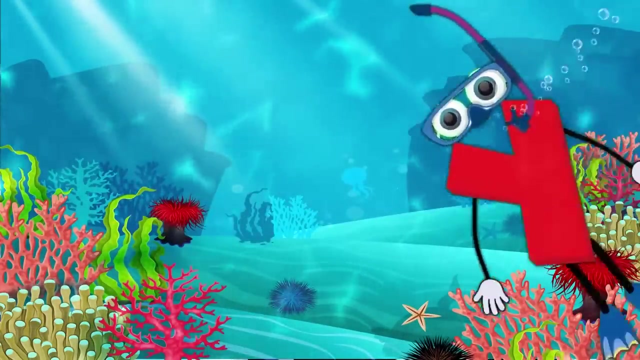 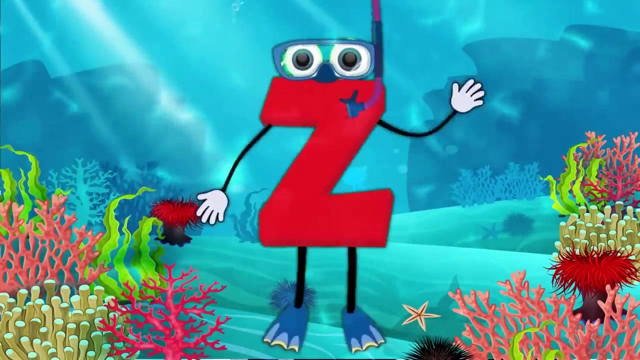 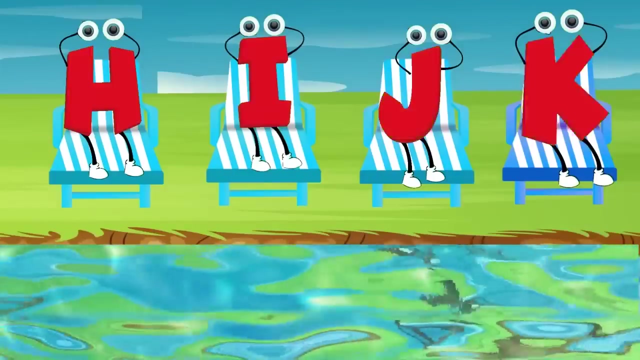 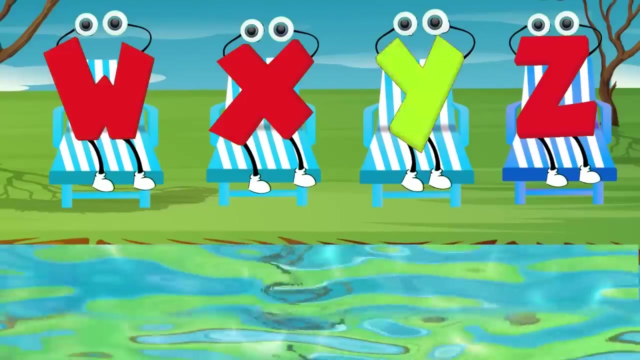 N O P Q R S T U V, W, X, Y and Z. A, B, C, D, E, F, G, H, I, J, K, L, M N O P Q R S T U V, W, X, Y and Z. 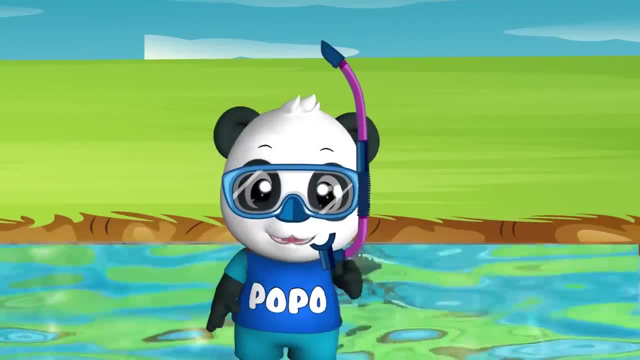 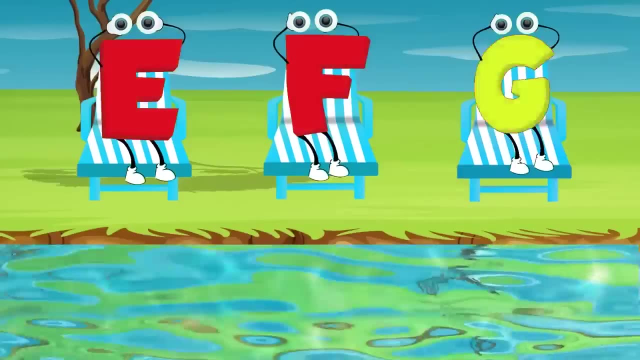 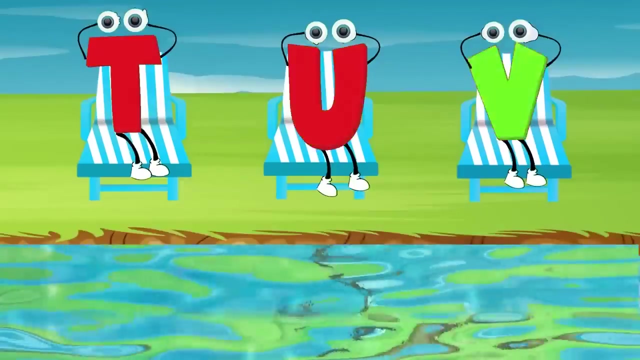 Now I know my A, B, C's. next time won't you sing with me? A, B, C, D, E, F, G, H, I, J, K, L, M, N, O, P, Q, R, S, T, U, V, W, X, Y and Z. 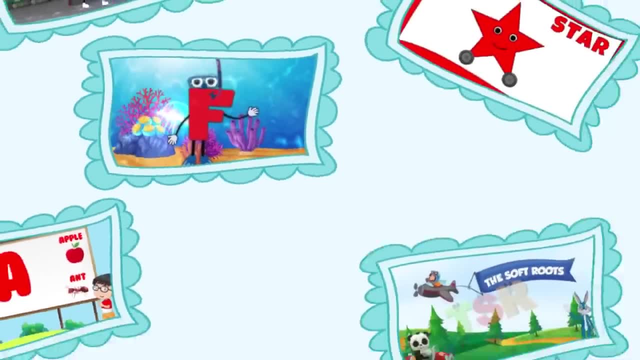 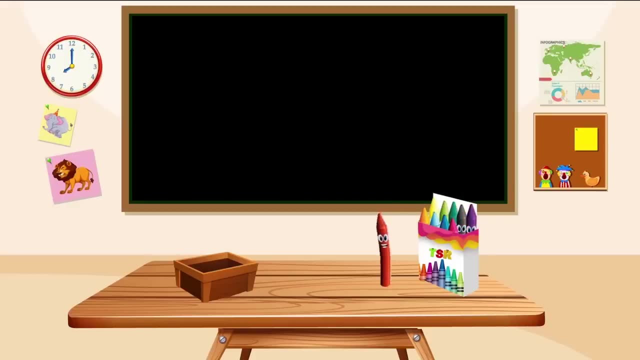 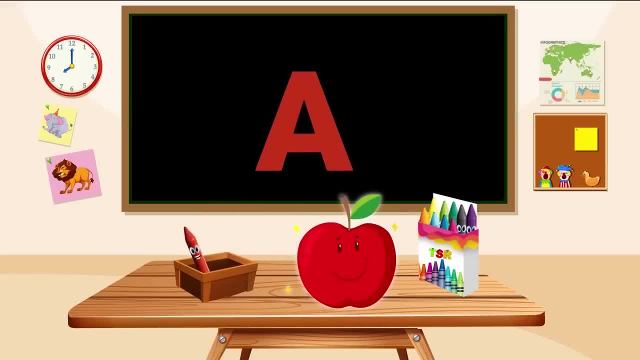 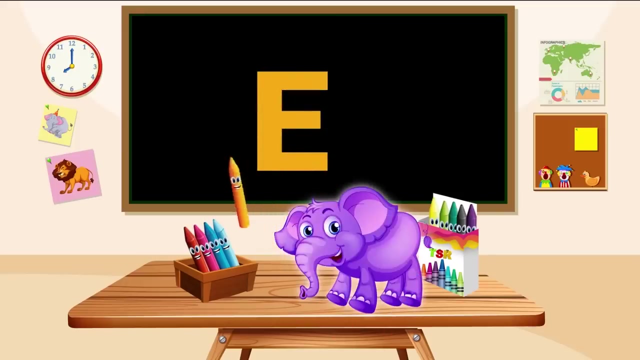 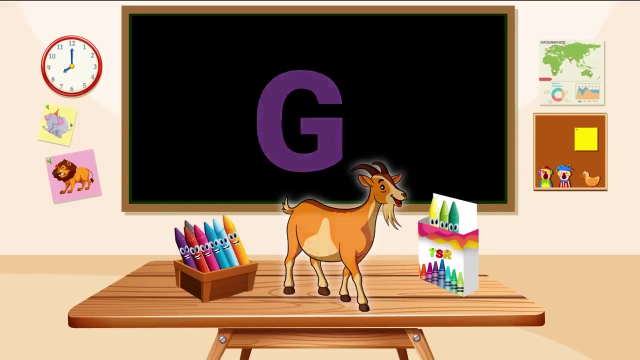 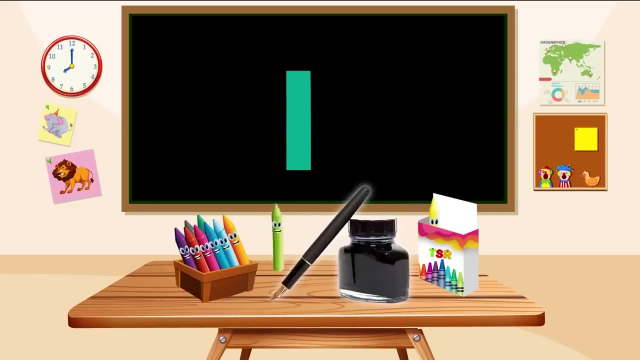 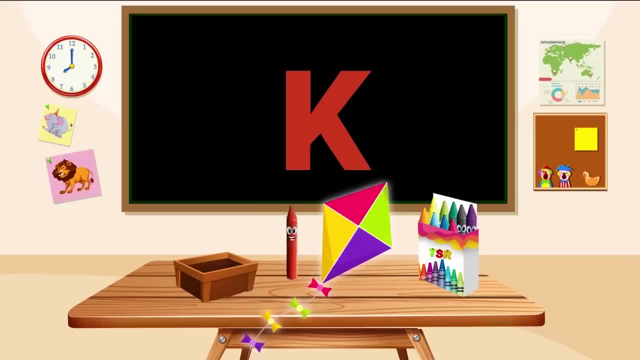 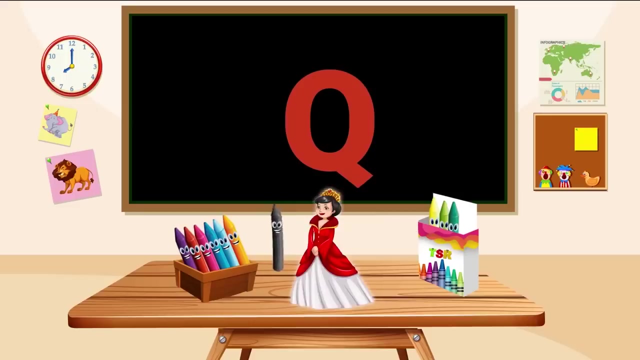 K for Kite L for Leaf M, for Monkey N for Net O for Owl P for Pencil Q for Queen Q for Queen R for Robot S, for Shoe S for Sleeve S, for Shoes S for Boots. 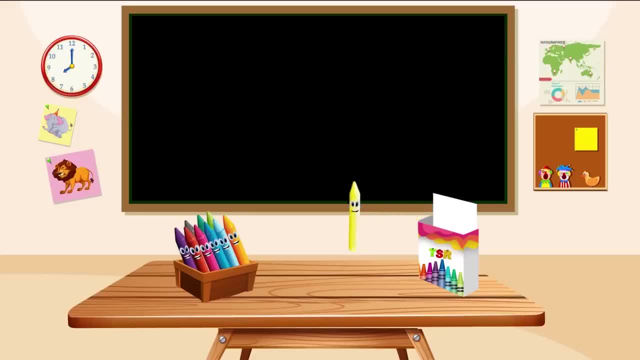 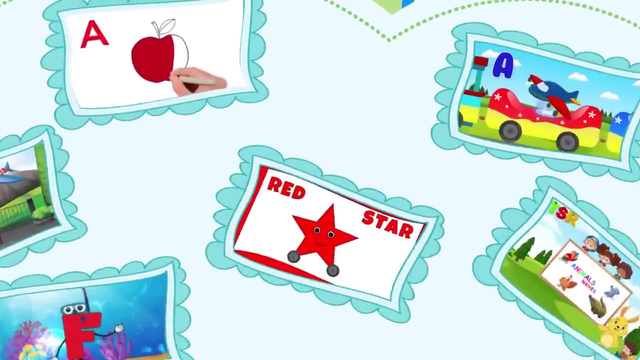 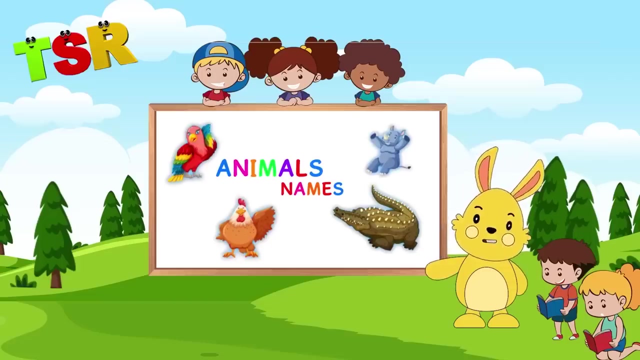 S for Shoes, R for Shoes, T for Train, U for Umbrella, V for Van, W for Watch, X for Christmas Tree, Y for York, Z for Zip, Z for Zip. Let us learn the alphabets along with the animal names: A, A, Alligator. 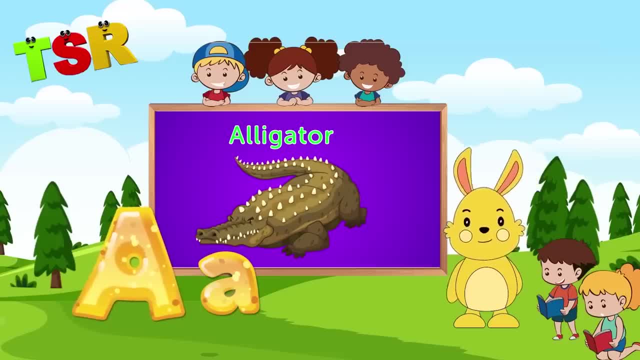 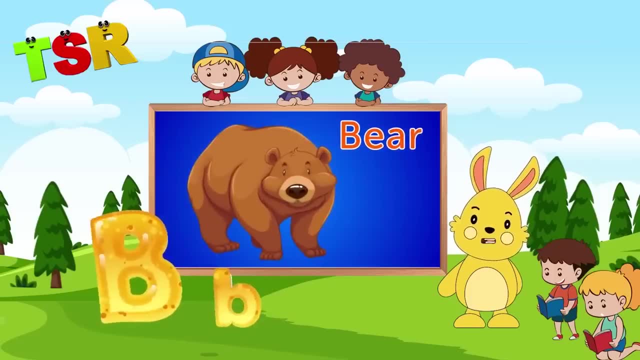 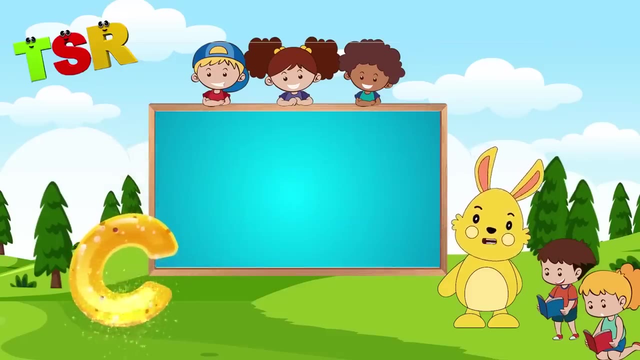 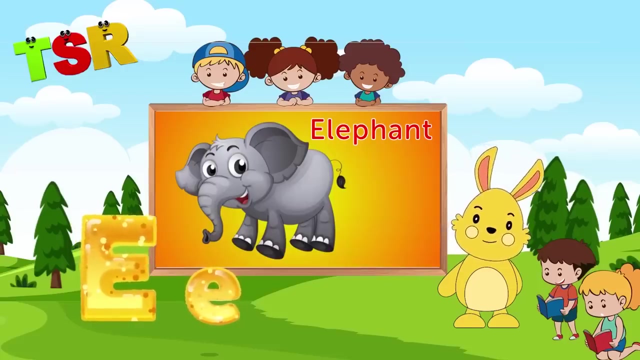 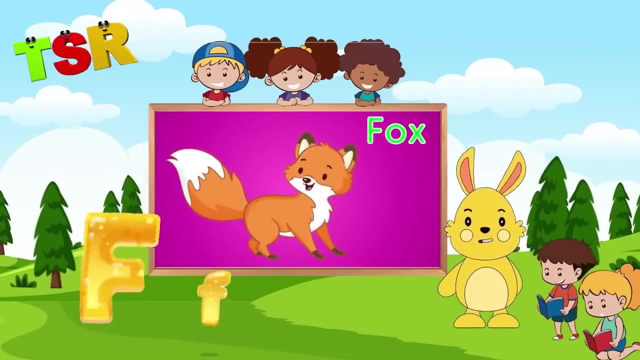 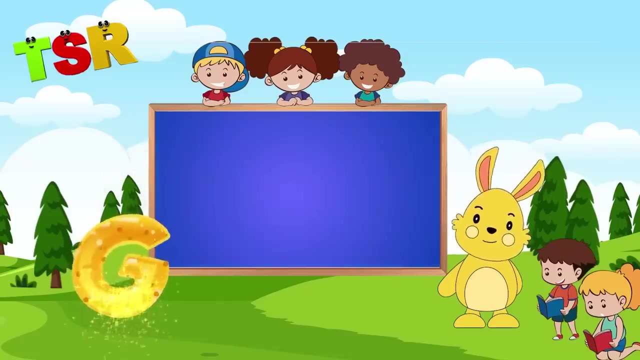 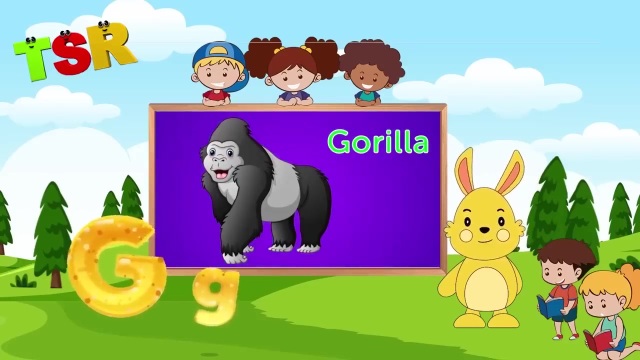 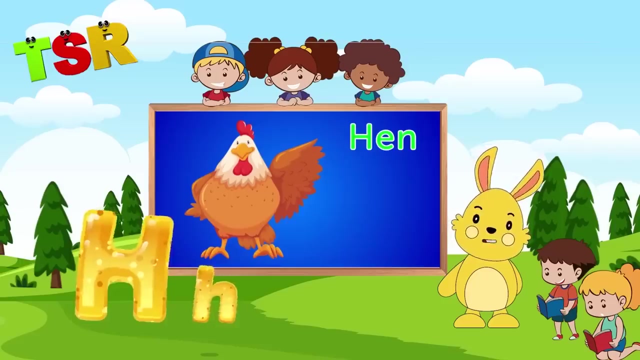 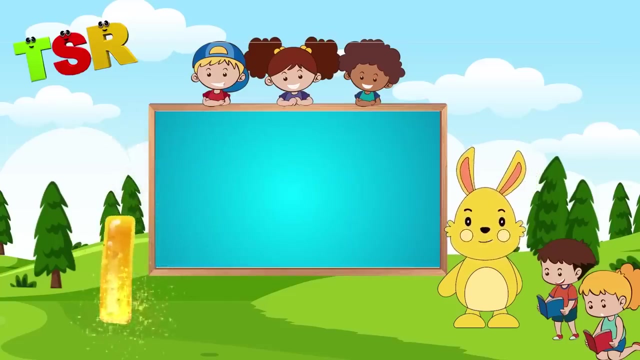 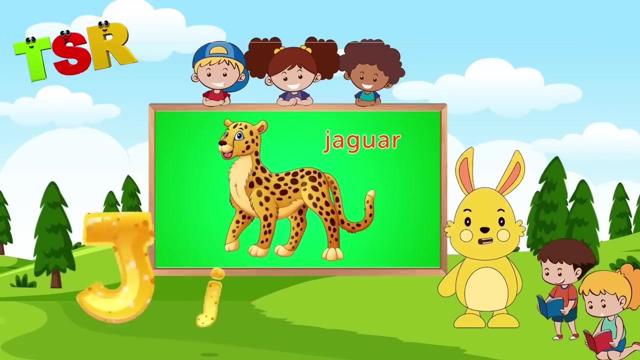 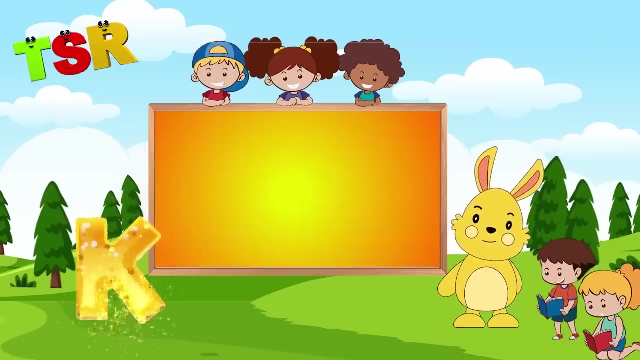 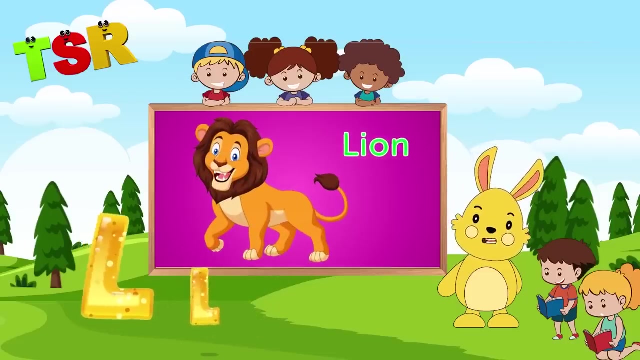 Alligator B, B, Bear Bear C, C, Cat D, D, Dog E, E E. Elephant F, F, F, Fox G, G, G G, gorilla, gorilla, H, H, hen, hen, I, I, guana, guana, J, J, jaguar, jaguar, K, K, kangaroo, kangaroo, L, L, lion, lion. 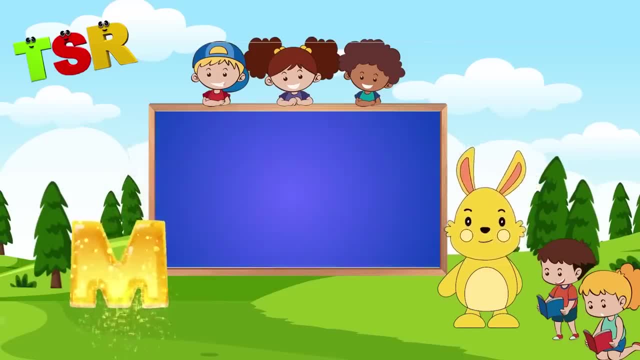 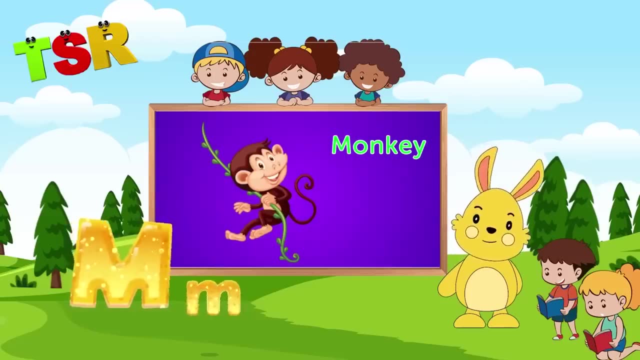 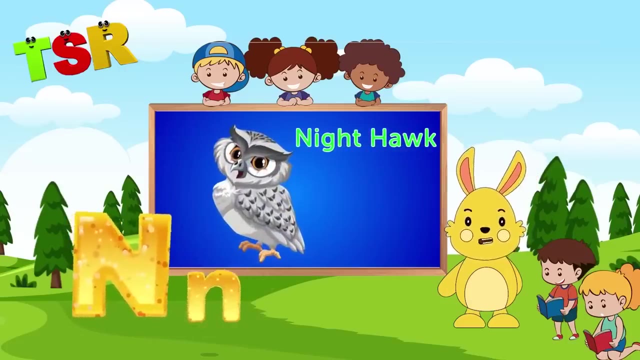 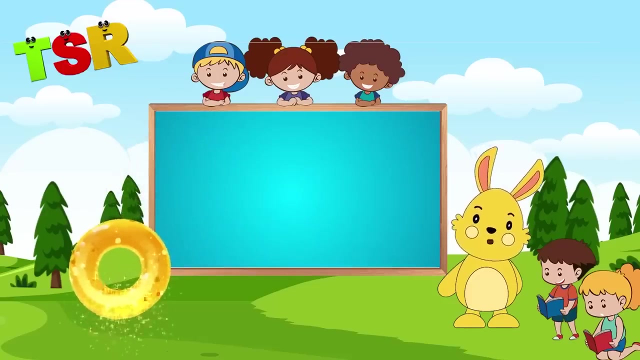 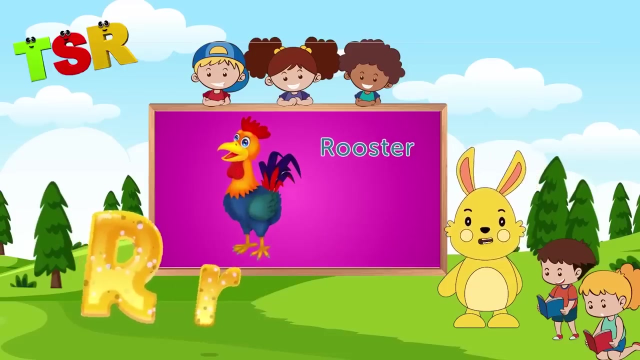 M M monkey N N, nighthawk, nighthawk, O O, ostrich, ostrich, P P, penguin, penguin, Q, Q, quail, quail, R R rooster. 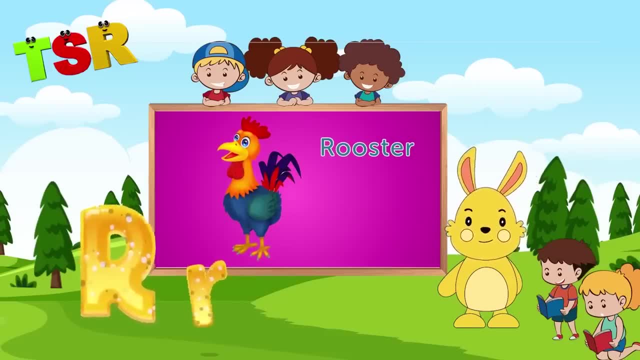 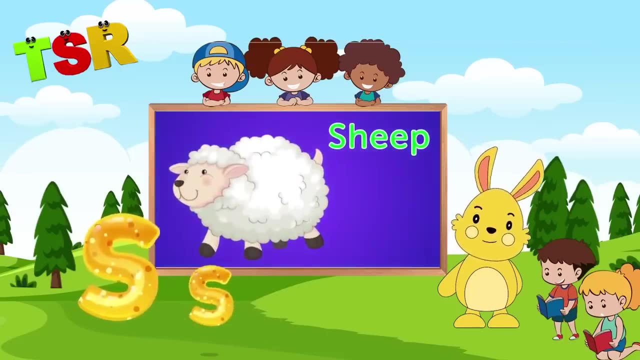 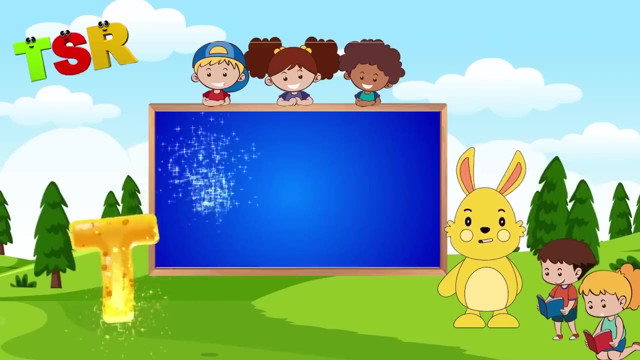 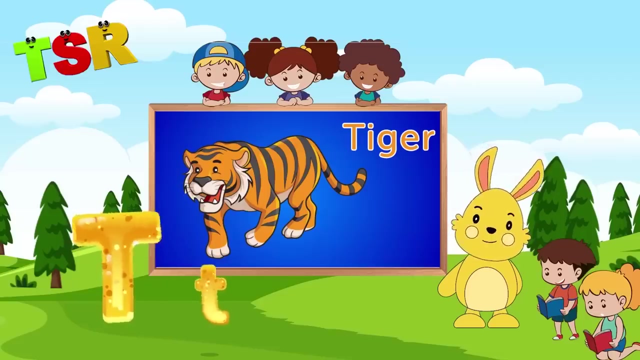 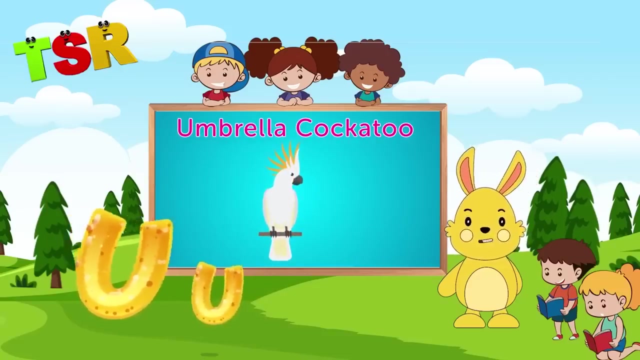 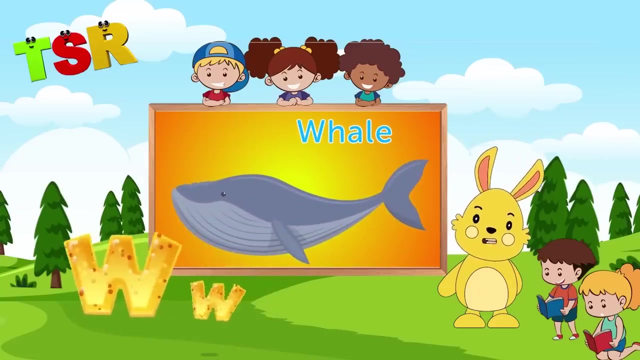 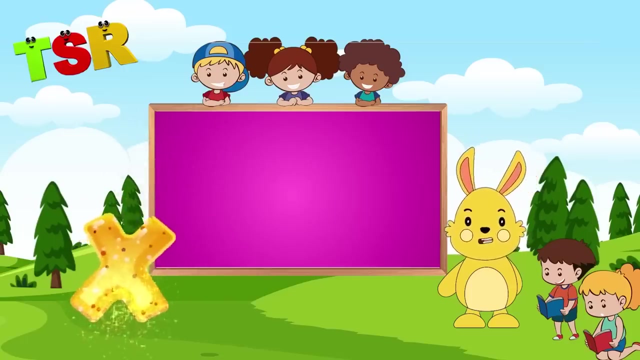 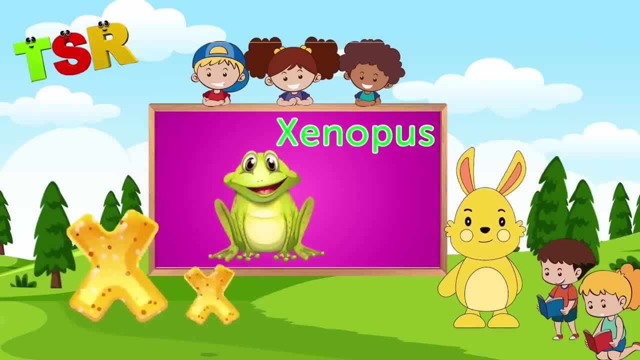 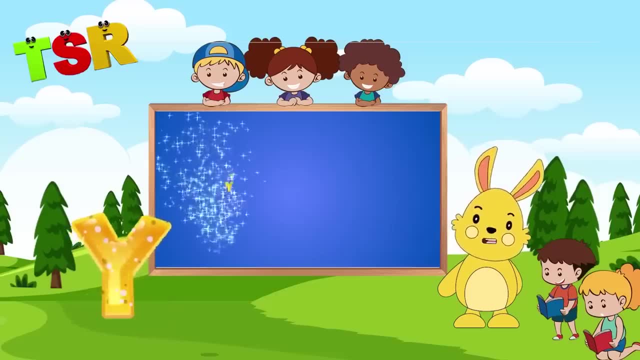 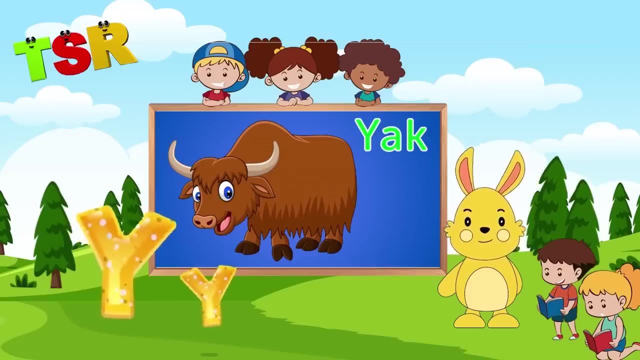 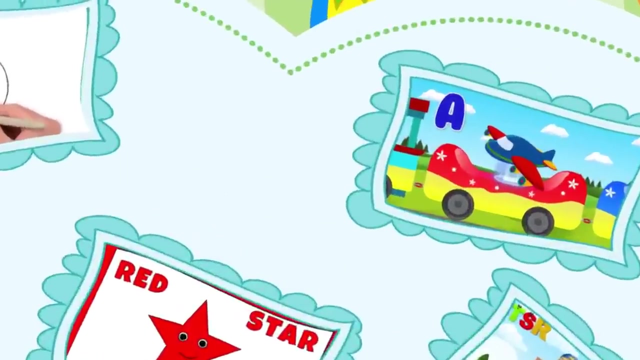 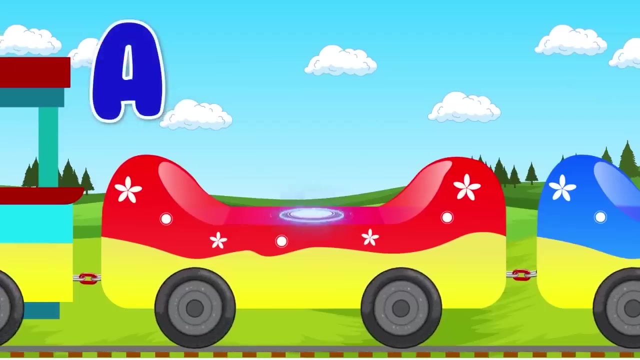 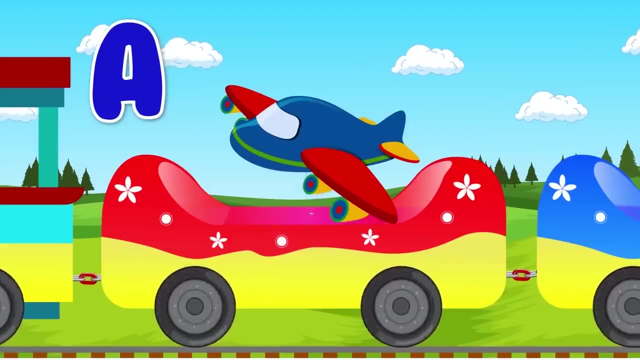 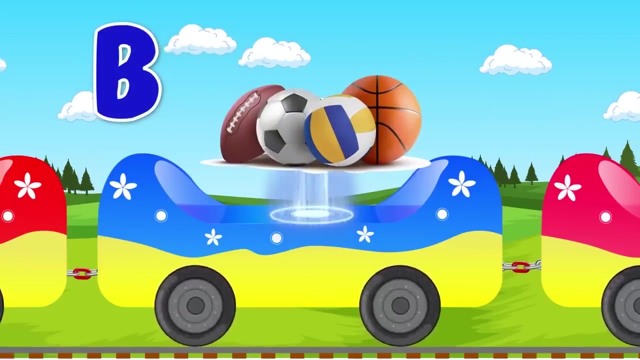 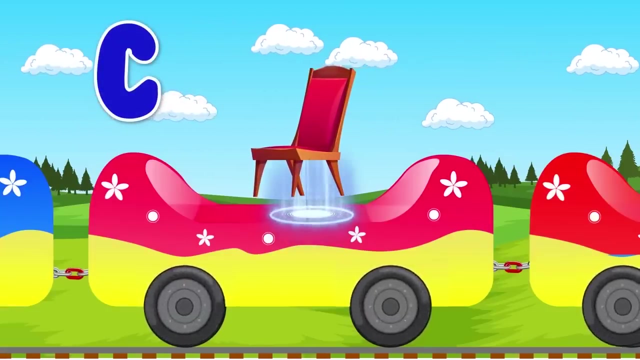 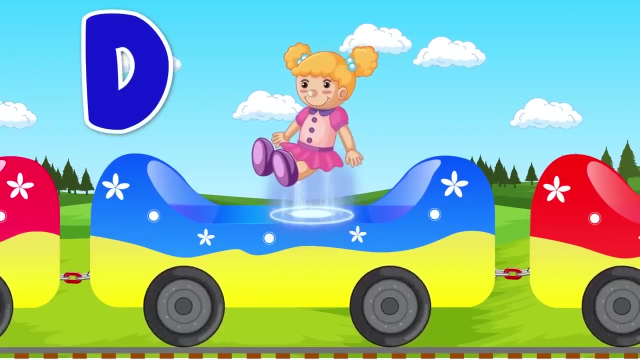 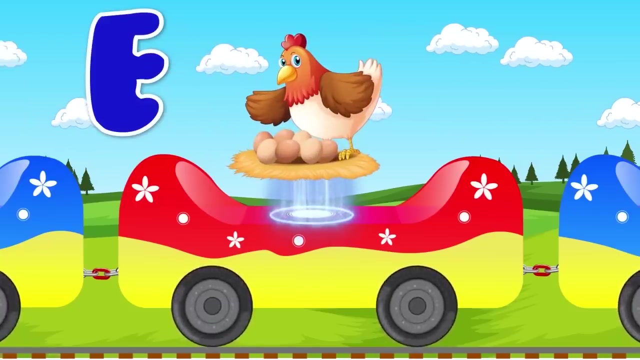 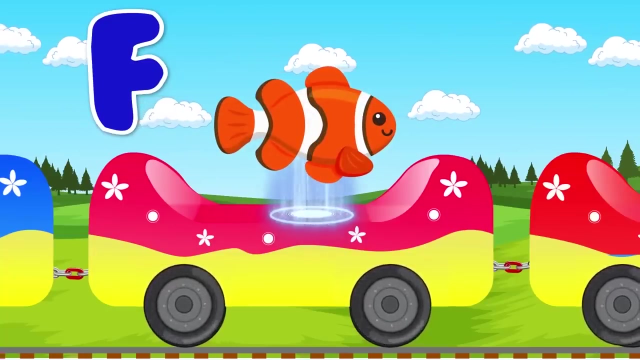 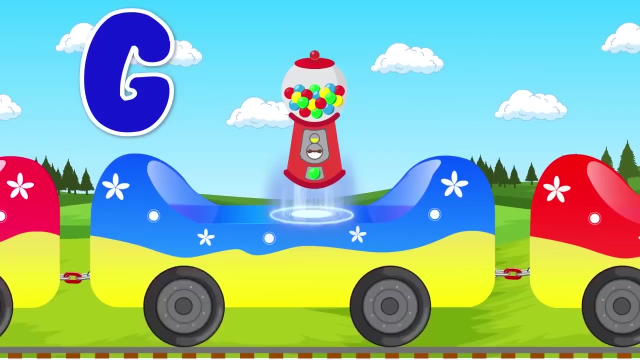 X, X-O-P-U-S. Y Y, YAK, YAK, Z Z. ZEB-RA A, AEROPLANE B, BOB C, CHAIR D, DOLL E, EGG, F, FISH, G, GUMBALLS. 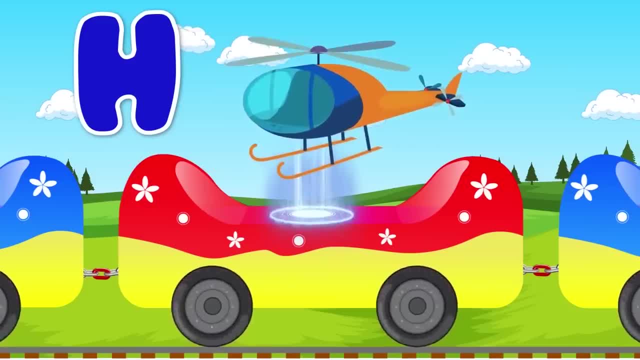 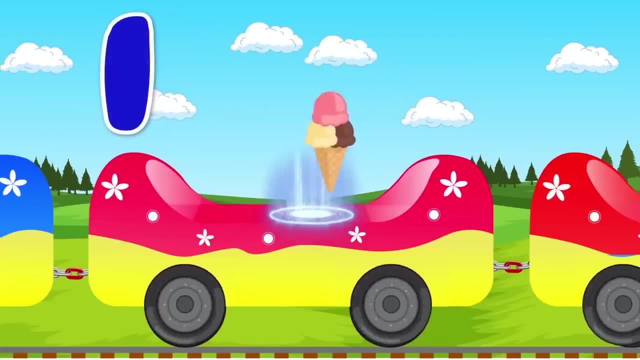 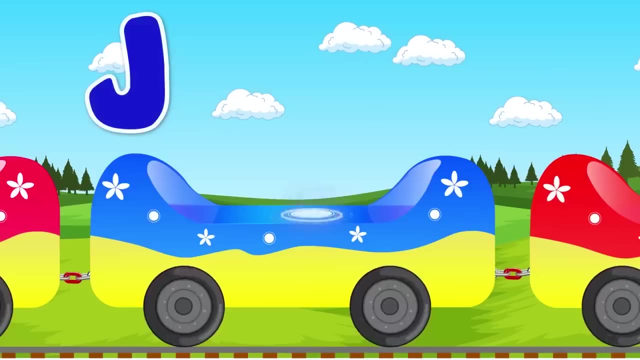 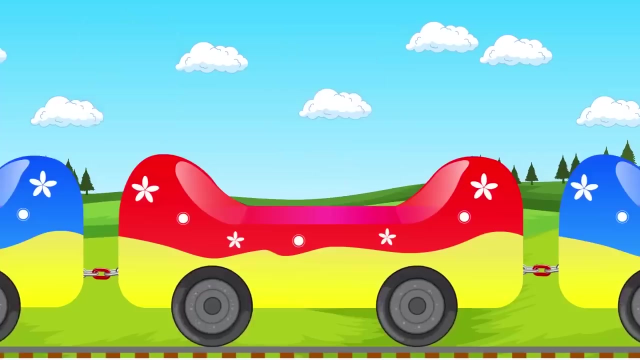 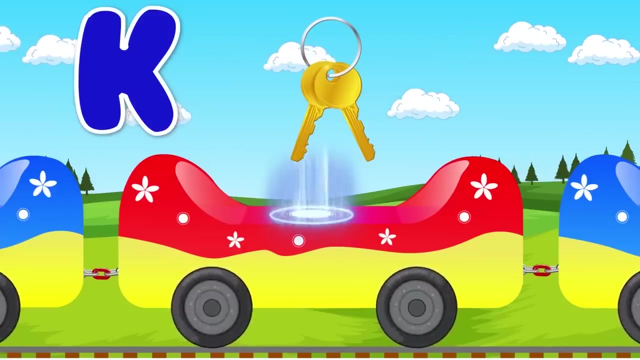 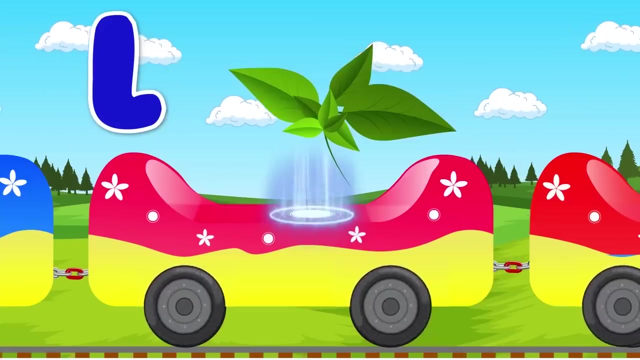 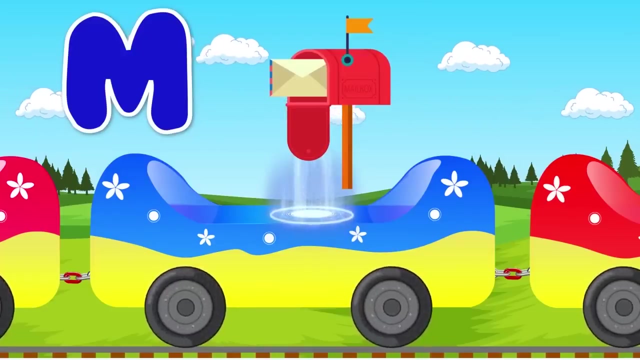 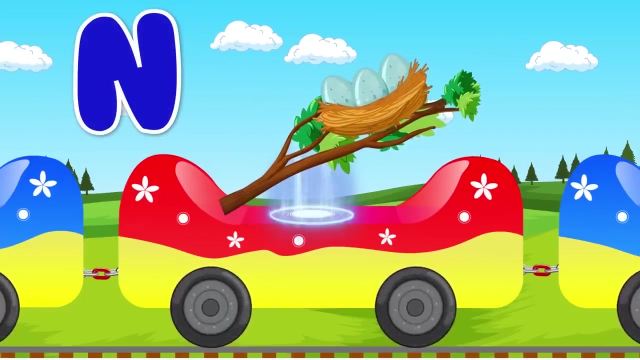 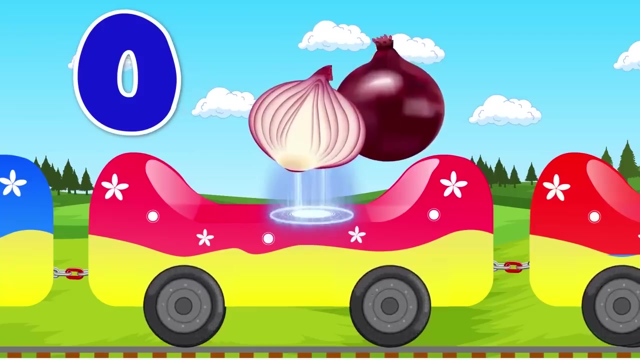 H HELICOPTER, I ICE CREAM, J JAM K KEYS K KEYS N LEAVES M MAILBOX N. NEST N NEST O ONION. O ONION, NEST NEST. 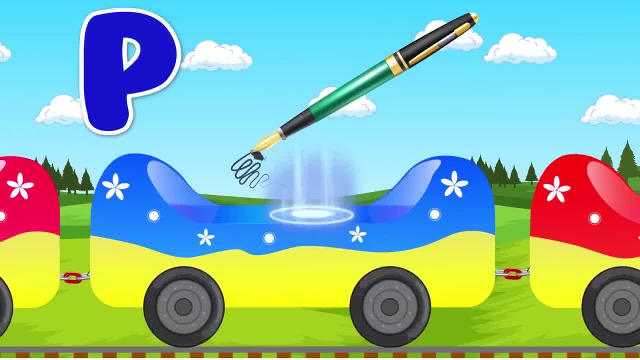 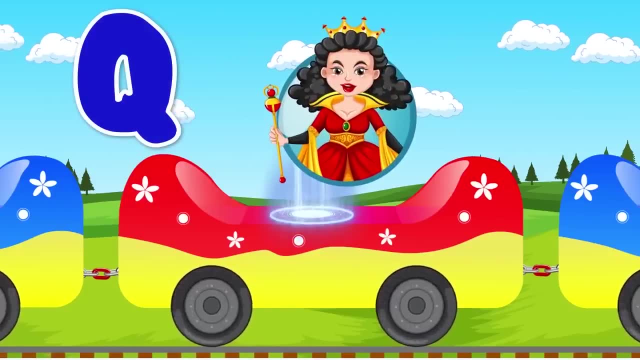 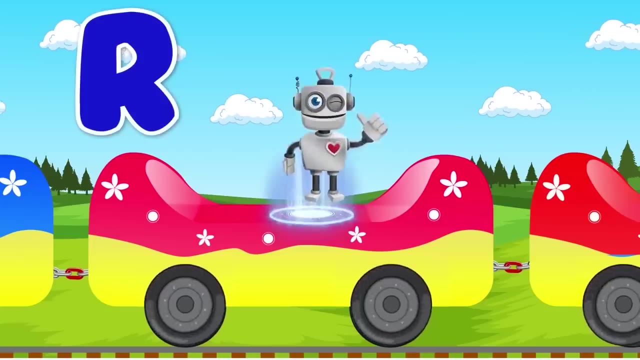 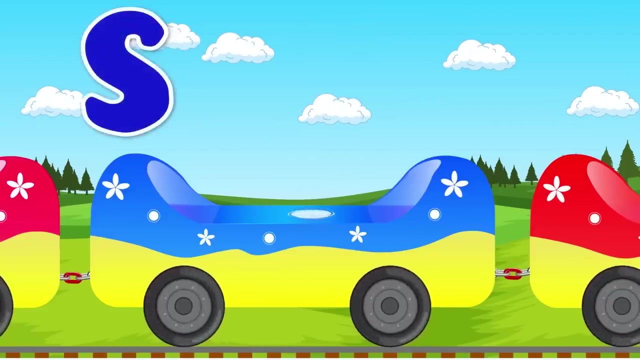 P PEN. P PEN. NEST NEST NEST NEST NEST NEST Q QUEEN Q QUEEN. NEST NEST NEST NEST NEST NEST R ROBOTS, R ROBOTS, NEST S Ship. 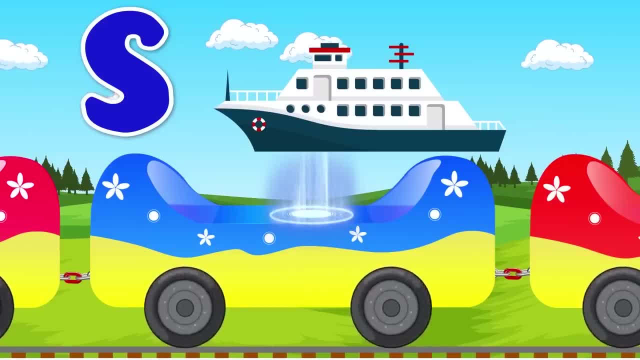 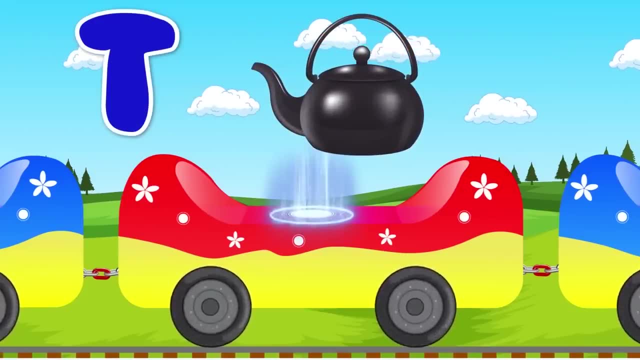 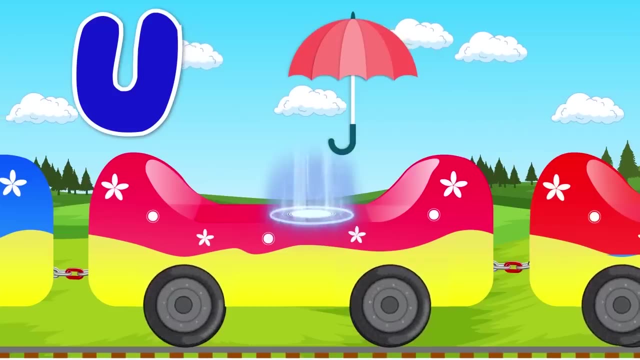 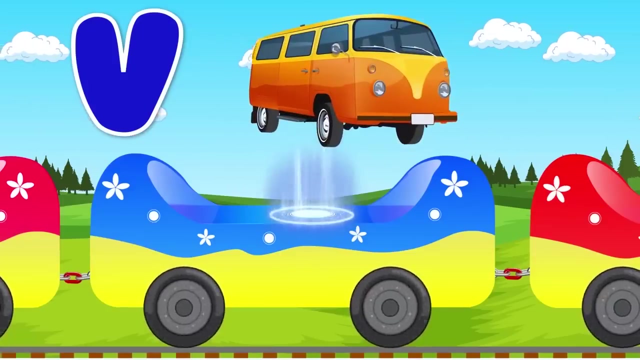 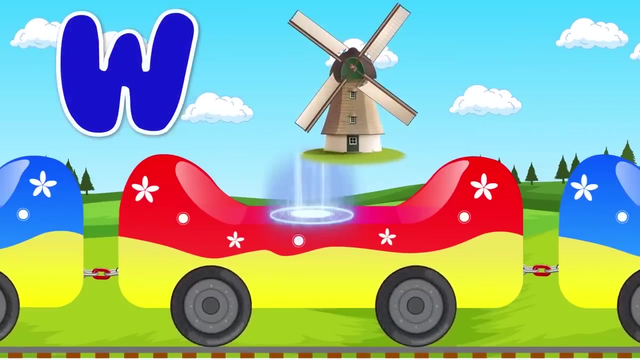 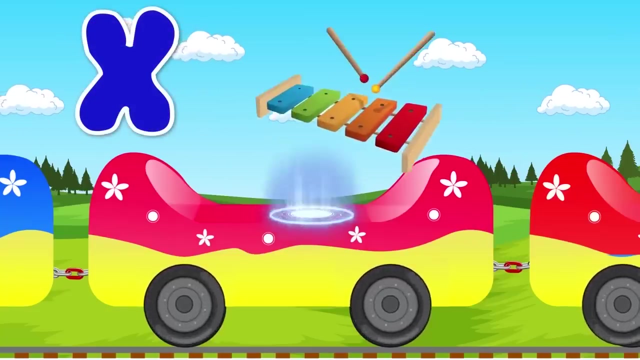 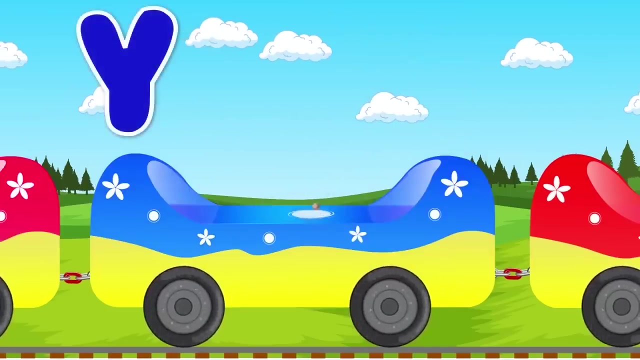 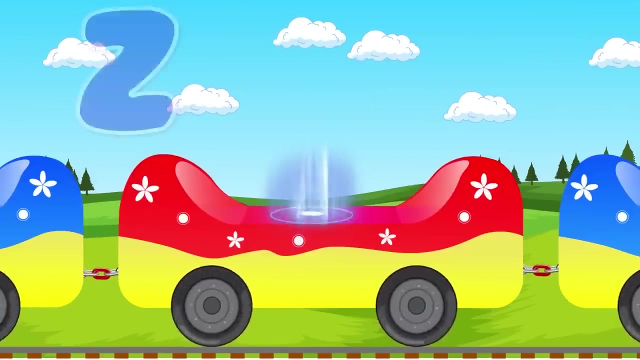 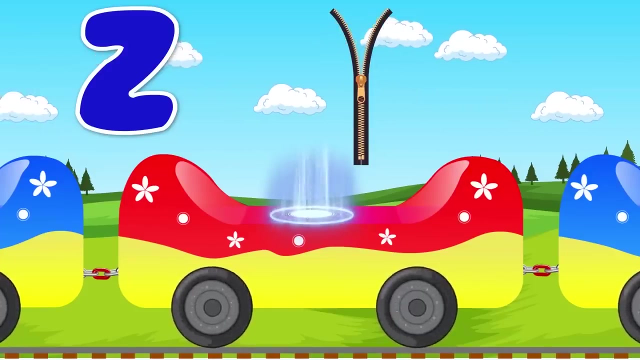 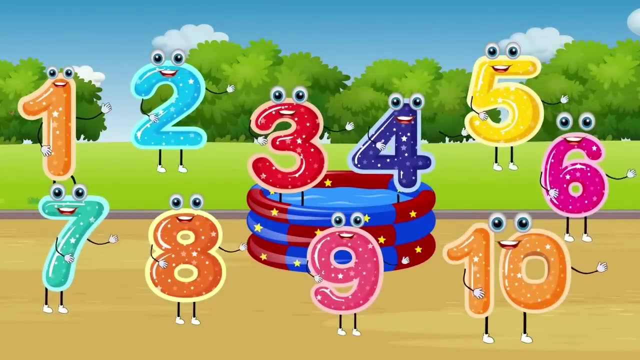 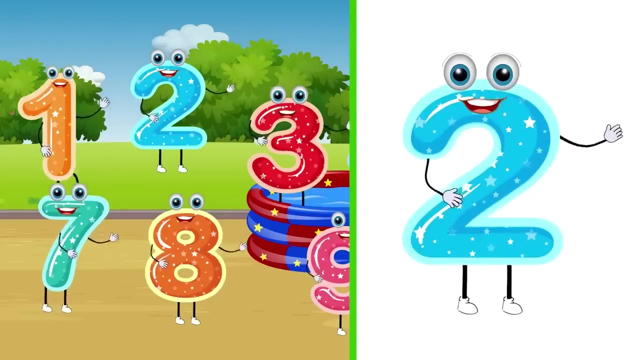 T Teapot U Umbrella V Van W Windmill X. Xylophone Z Windmill Z Windmill Y Yarn Z Zipper. 1. 1, 2. 2, 3. 3. 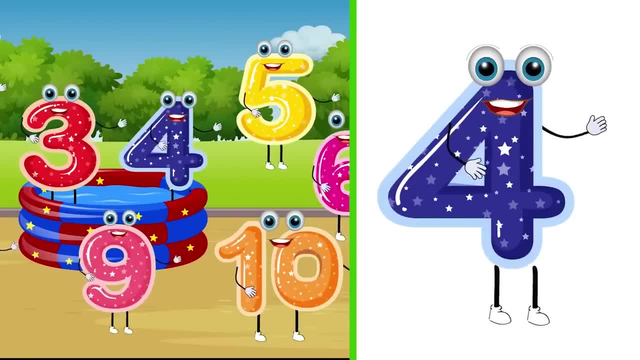 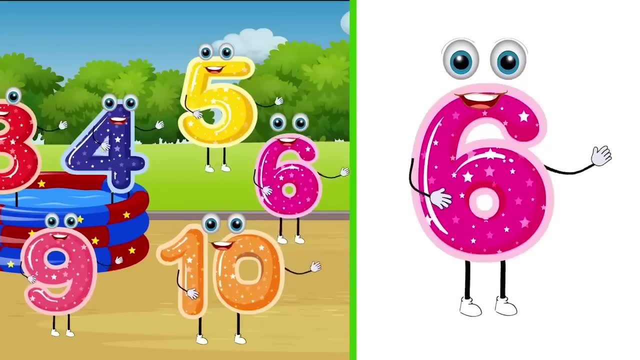 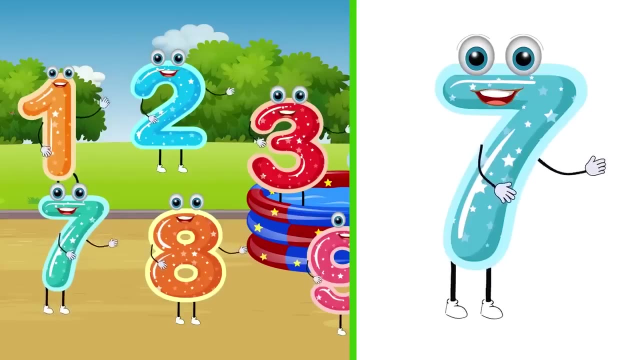 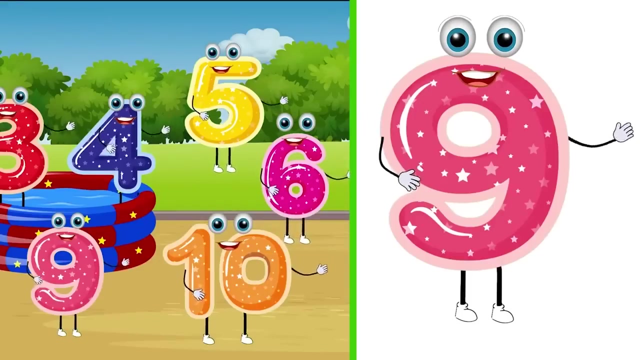 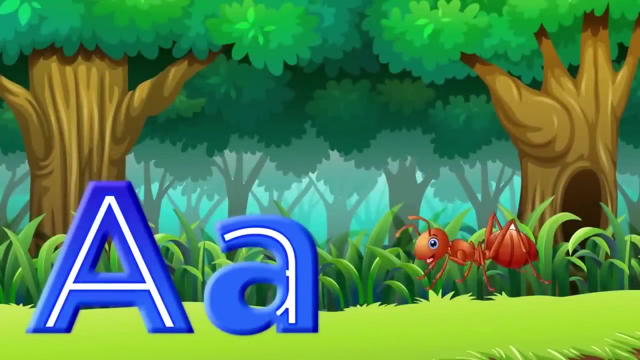 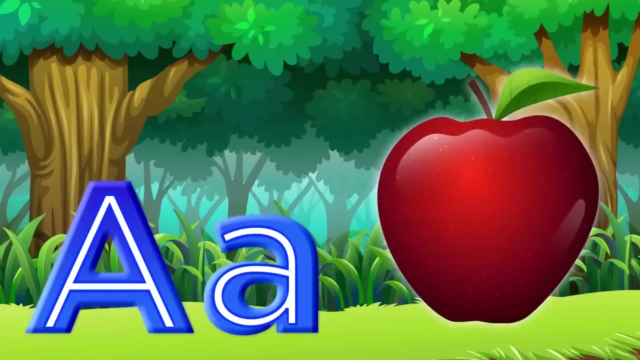 4. 4, 5. 5, 6. 6, 7. 7, 8. 8, 9. 9, 10. 10, 10. 10. A for Ant A- a. ant. A for Apple A- a apple. 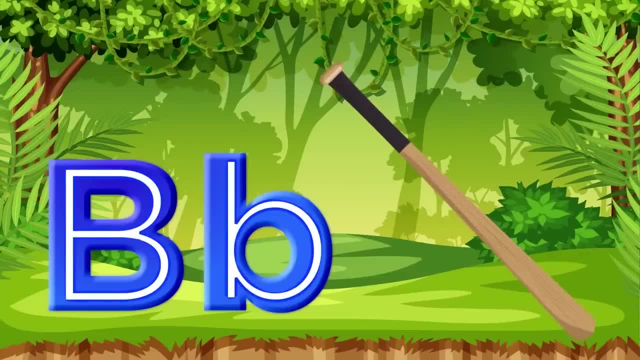 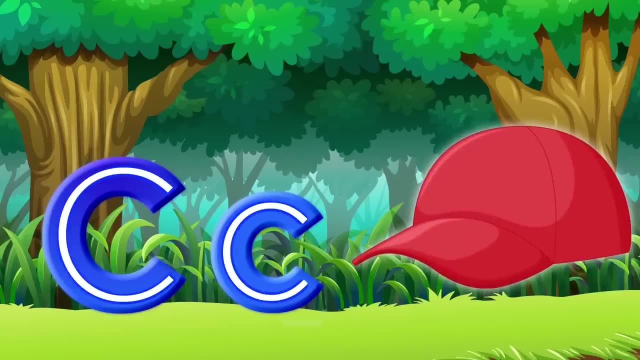 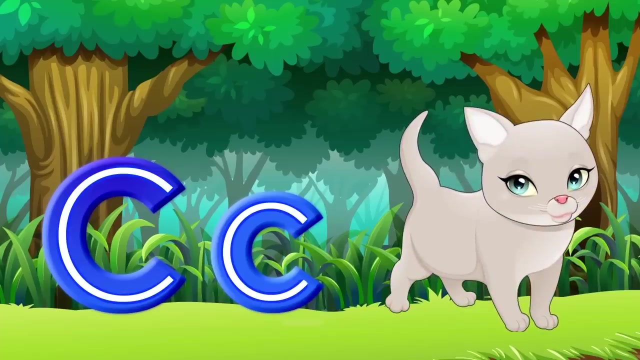 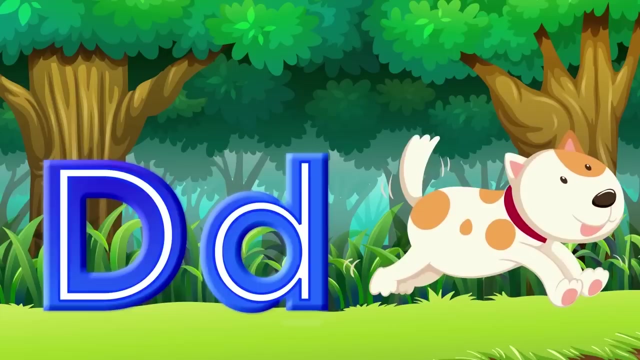 B for Bat B- B-. Bat B for Ball B- B- Ball Z. Ball C for cap c-c-cap C for cat c-c-cat. D for dog d-d-dog. D for dots d-d-dots. 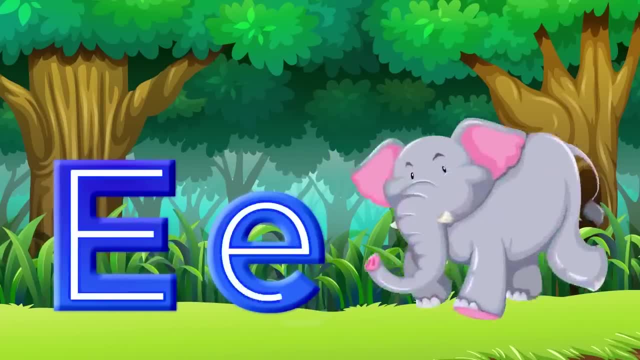 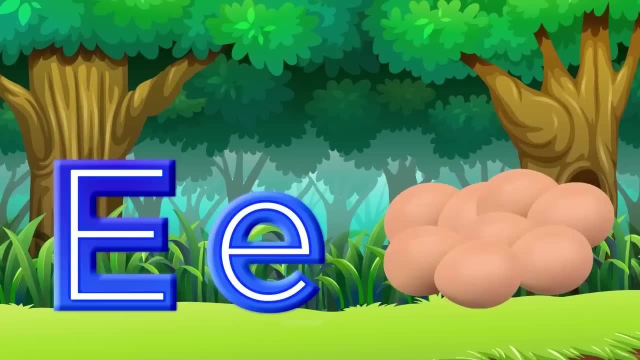 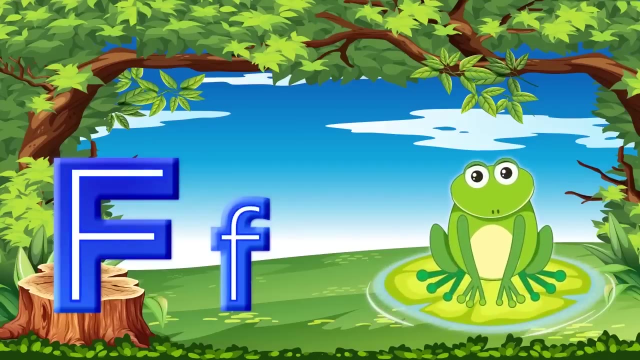 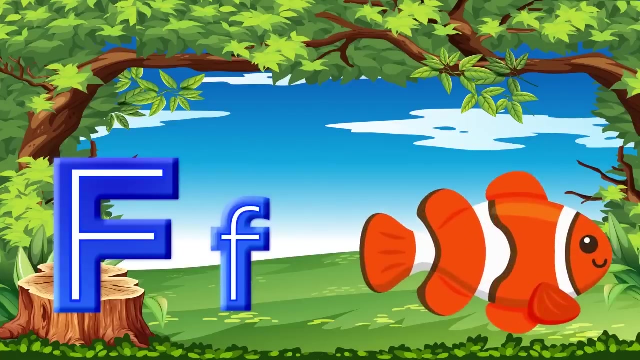 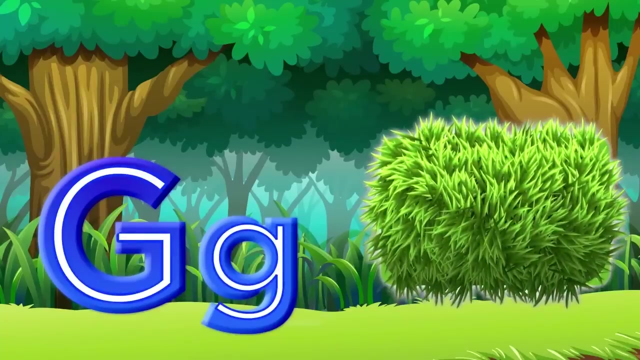 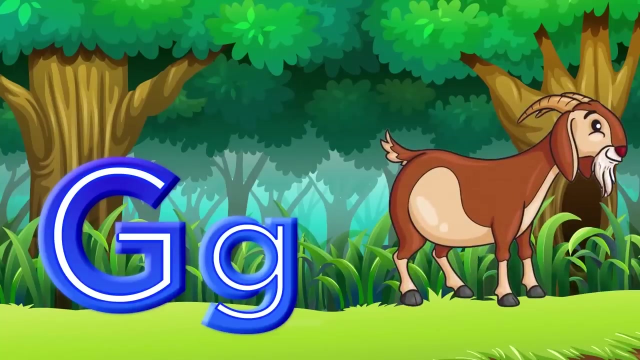 E for elephant: e-e-elephant. E for egg: e-e-egg. F for frog: f-f-frog. F for fish: f-f-fish. G for grass: G-g-grass. G for goat: g-g-goat. 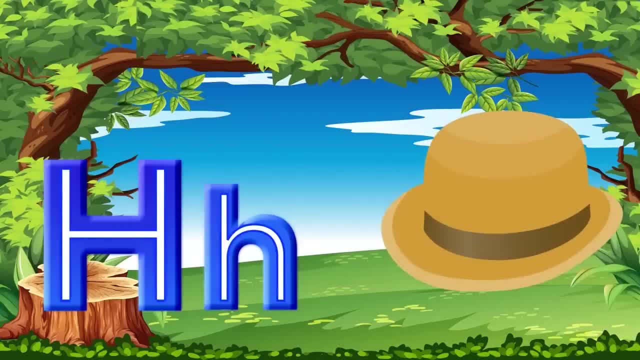 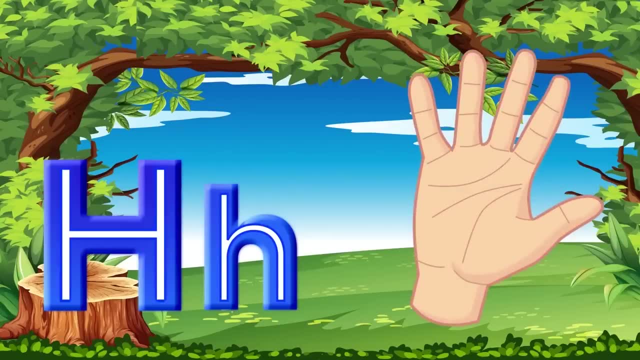 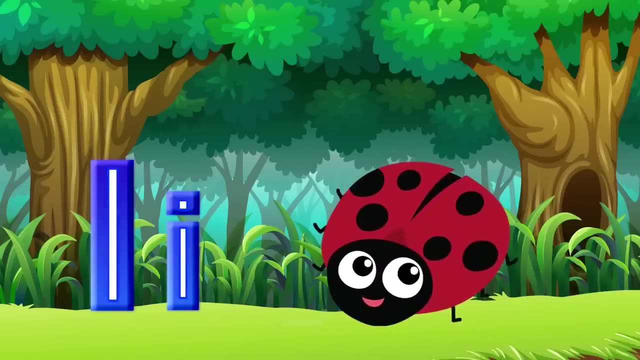 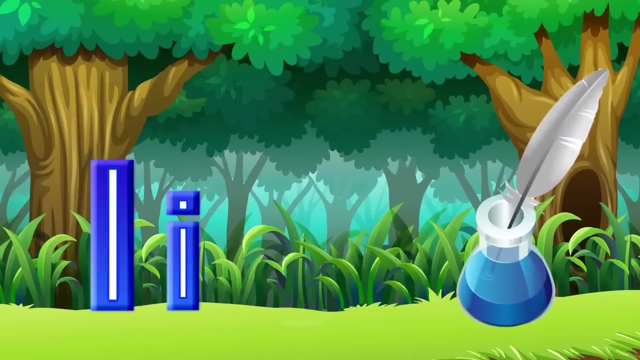 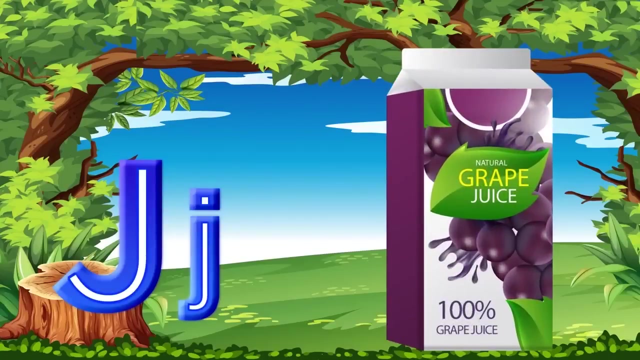 H for hat: h-h-hat. H for hand: h-h-hand. I for insect: p-p-insect. I for ink: i-i-ink. J for juice: j-j-juice. J for jar: j-j-jar. 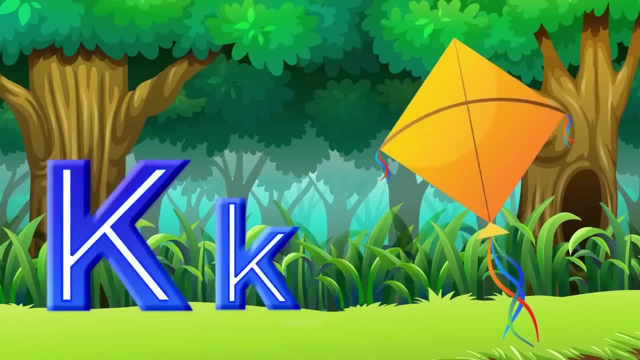 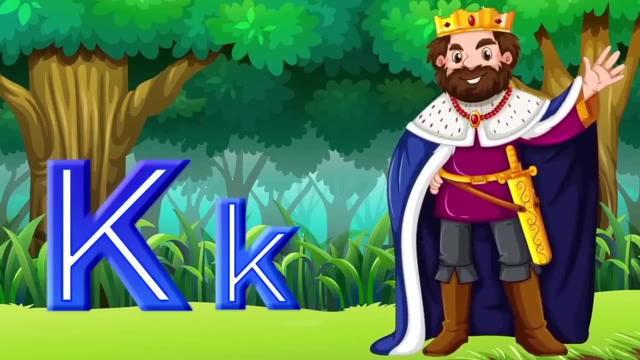 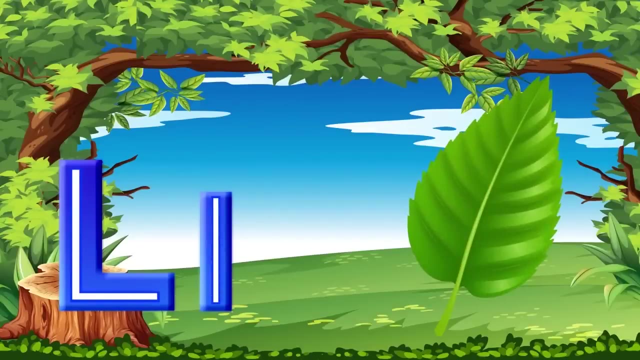 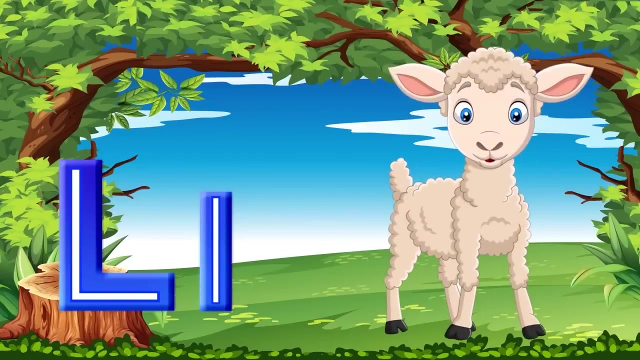 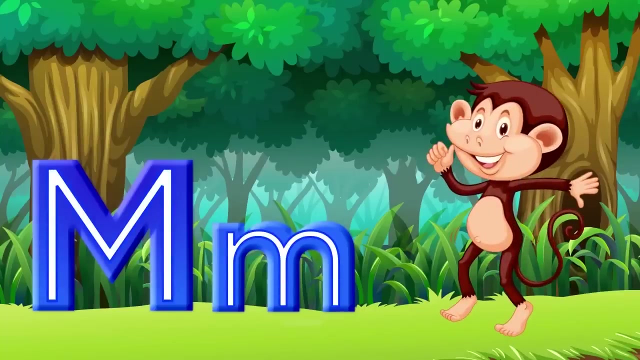 K for kite: k-k-kite. K for king- k-k-kite. K for bag: k-k-king L for leaf: l-l-leaf. L for lamb: l-l-lamb. M for monkey: m-m-monkey. 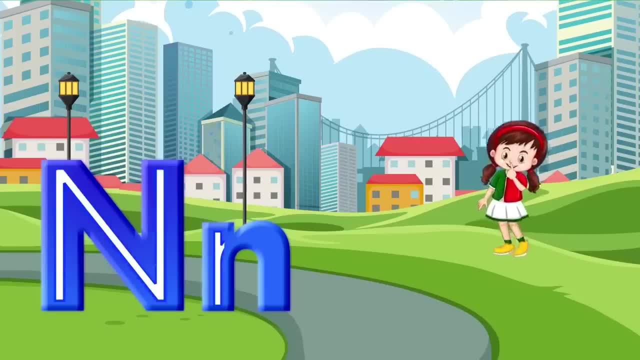 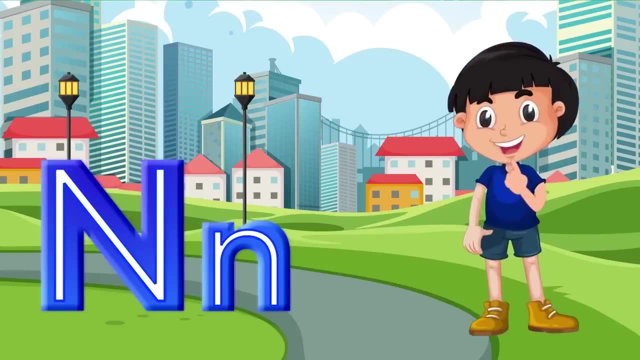 M for man: m-m-man. C for rope: j-j-j-j. C. for frog: j-j-j-j. T for approached: n-w-c-c. N for nose: n-n-nose. N for neck: n-n-neck. 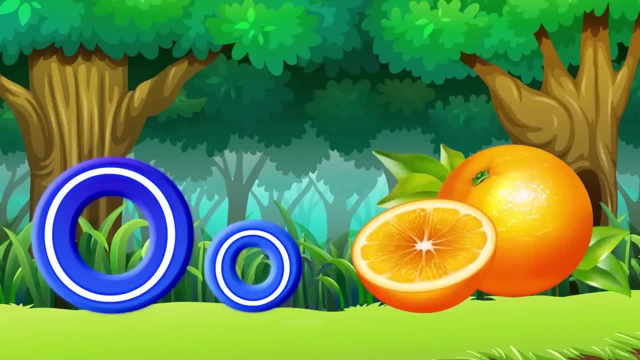 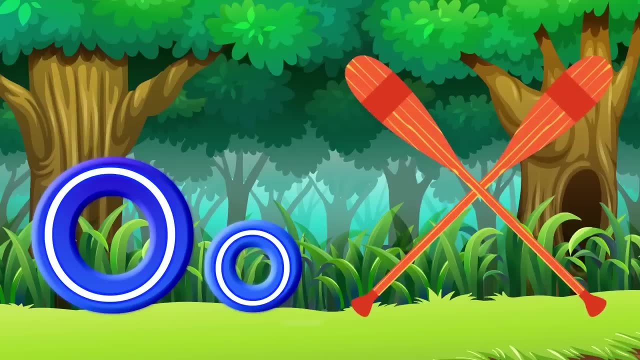 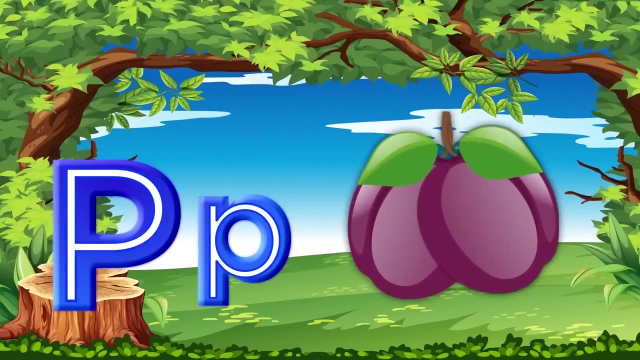 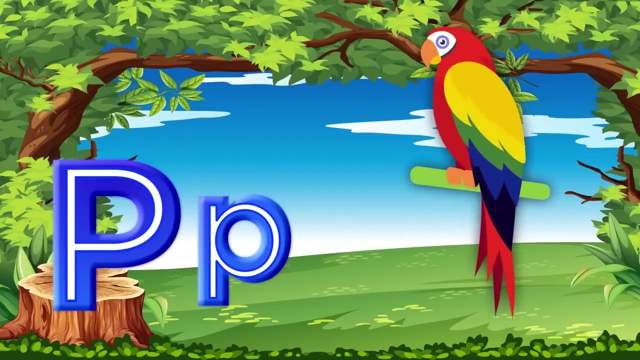 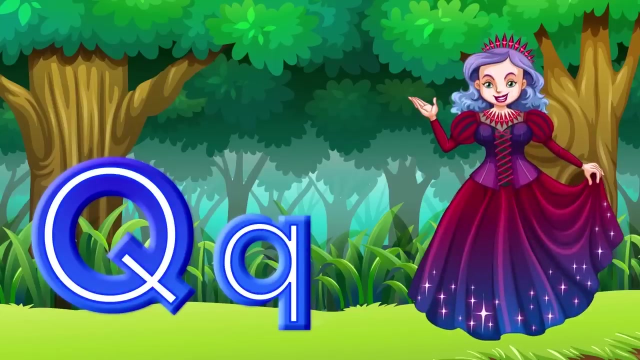 O for orange. O for ore o-o-ore. P for plum: P-p-plum. P for parrot: p-p-parrot. Q for queen: q-q-queen. Q for quail: q-q-quail. 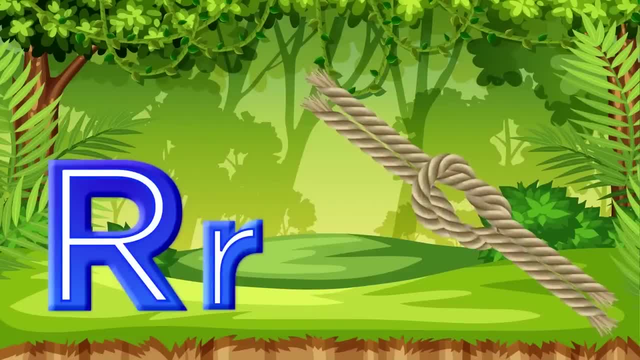 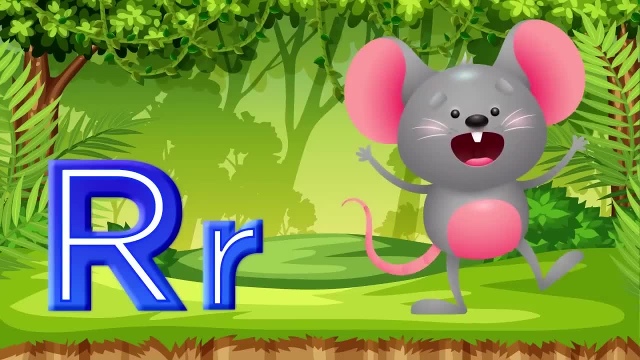 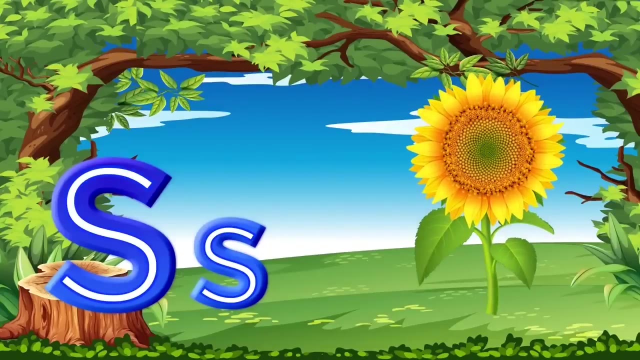 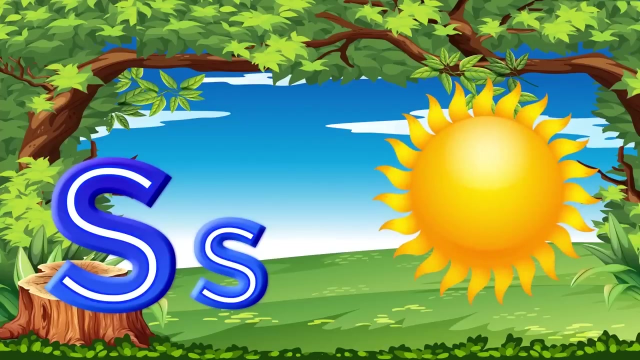 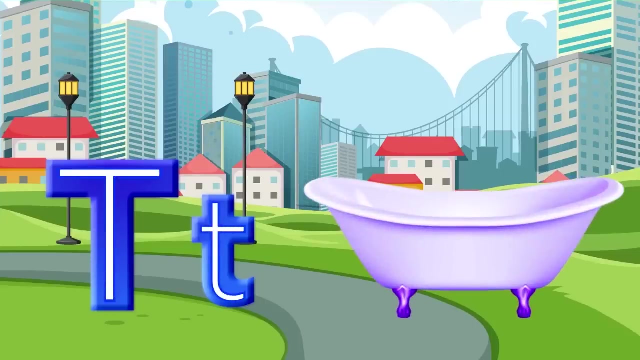 R for rope: r-r-rope. R for rat: r-r-rat S for sunflower s-s-sunflower, S for sun s-s-sun. T for tub: t-t-tub. T for tap: t-t-tap. 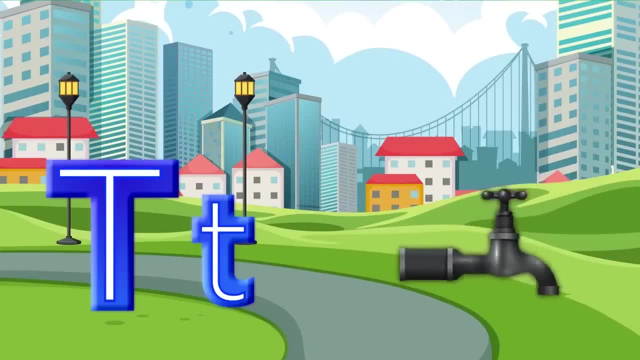 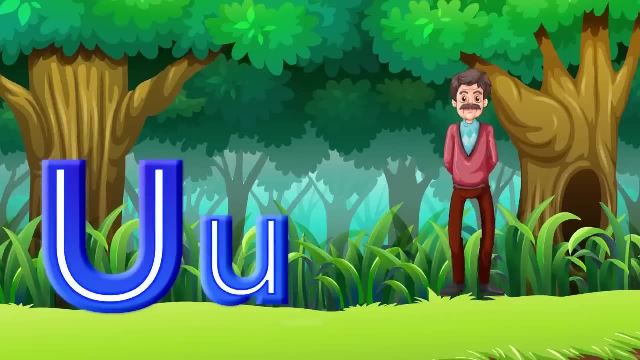 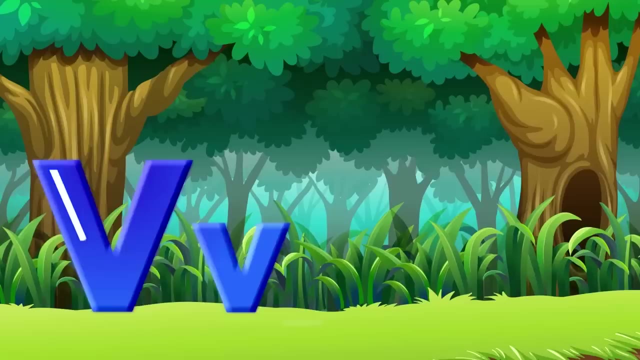 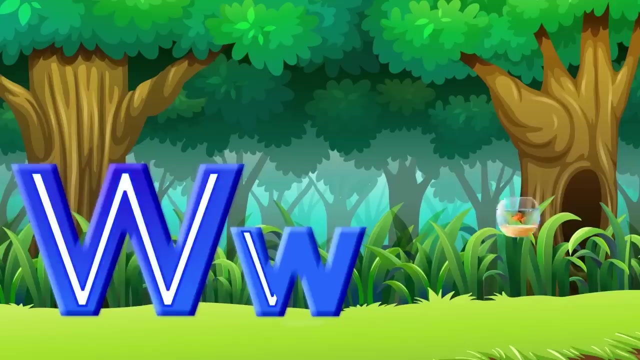 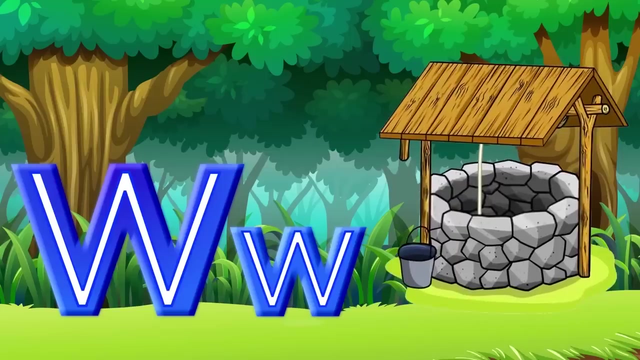 U for uncle, u-u-uncle. U for umbrella: u-u-umbrella. V for violet: v-v-voilet. V for violin: v-v-voilin'. W for water: v-v-water. W for will: v-v-will. 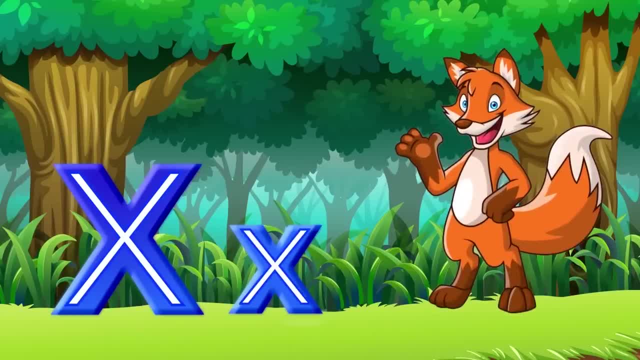 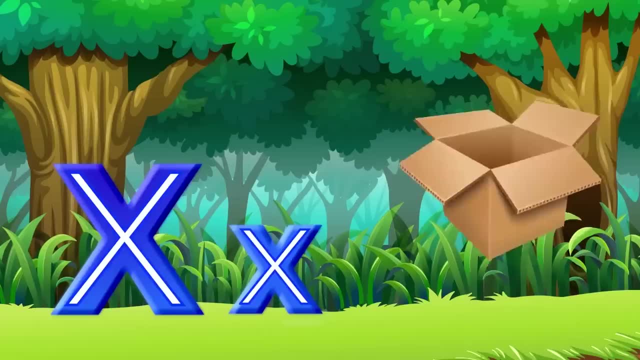 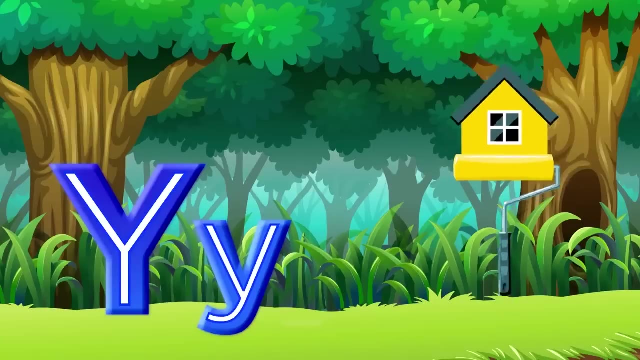 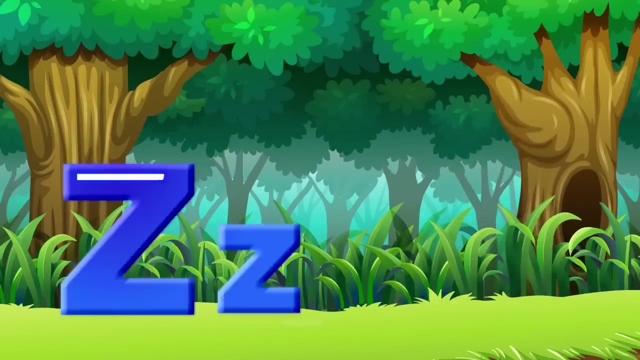 X for fox s-s-fox, X for box s-s-box, Y for yellow yellow. Y for yellow y-y-yellow, Y for yacht y-y-yacht, Z for zoo- z-z-zoo, Z for zebra z-z-zebra. 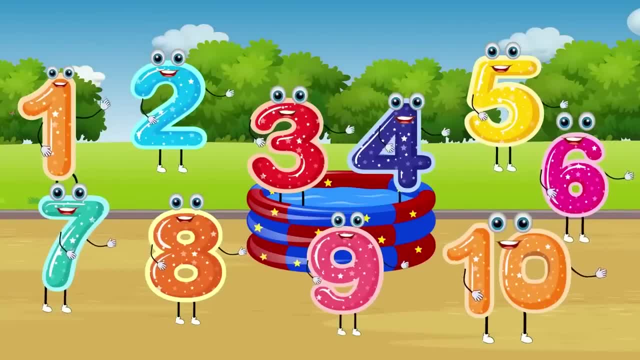 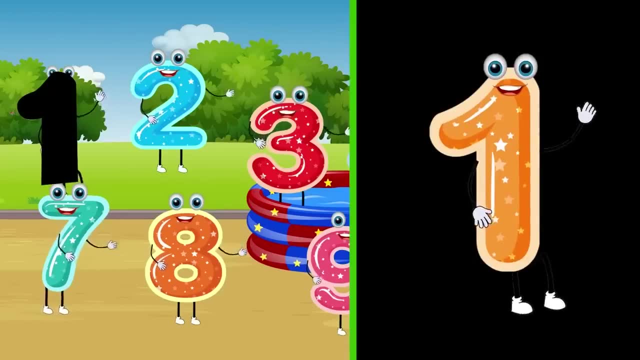 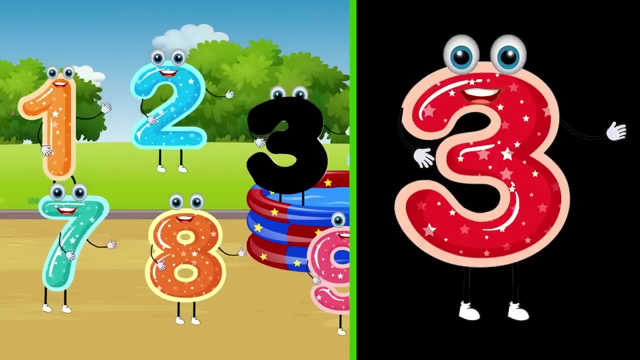 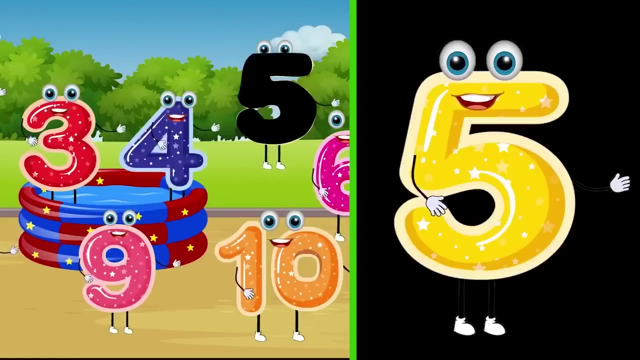 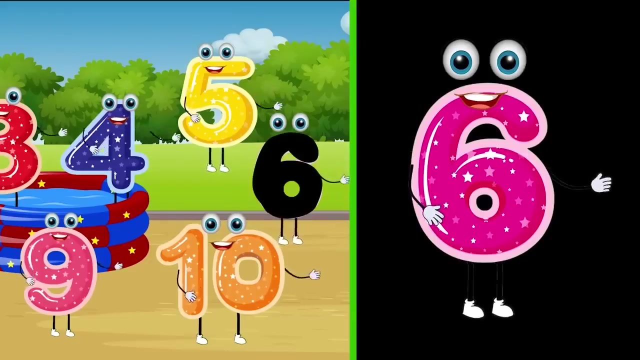 One, two, three, four, One, two, three, four, One, two, three, four. One, one, two, two, three, three, four, four, five, five, six, six, seven, seven, eight. 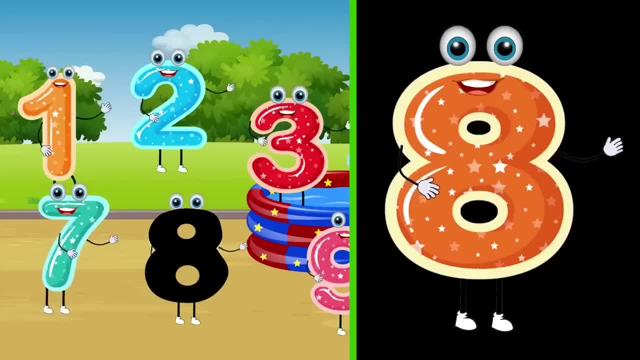 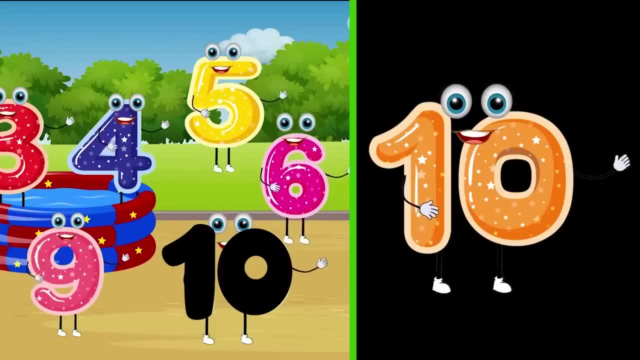 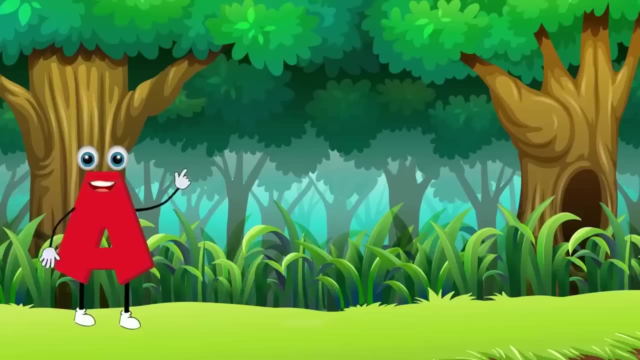 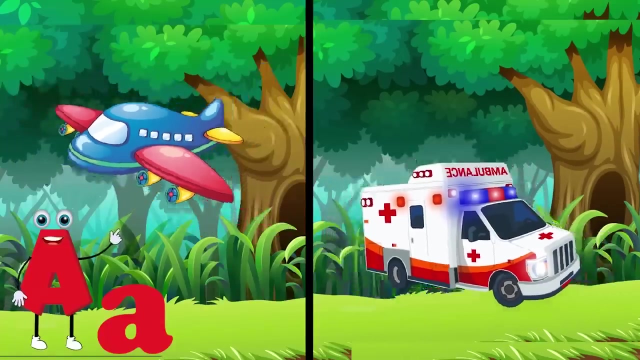 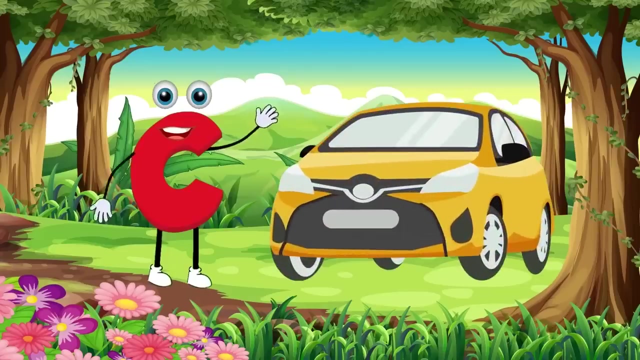 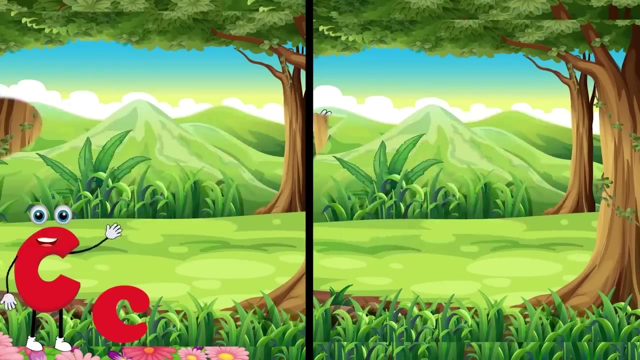 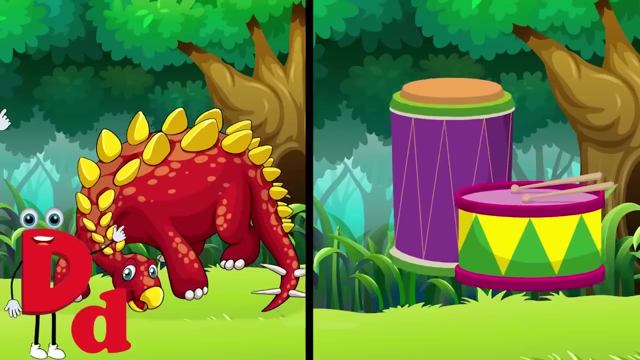 eight, eight, nine, nine, ten ten: A for Airplane, A for Ambulance: A, A, A, B for Bus, B for Boy, B, B, B, C for Car, C for Cow, C, C, C, D for Drum, D for Dinosaur, D, D, D, E for Angel. 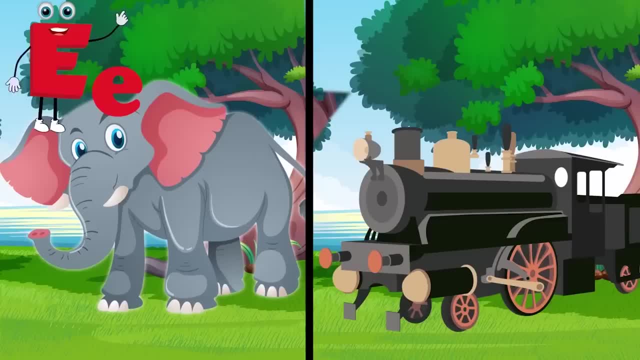 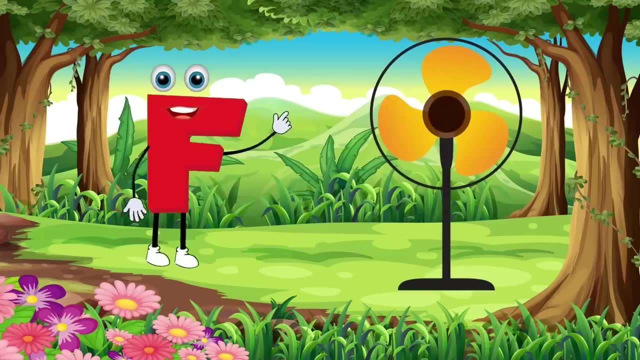 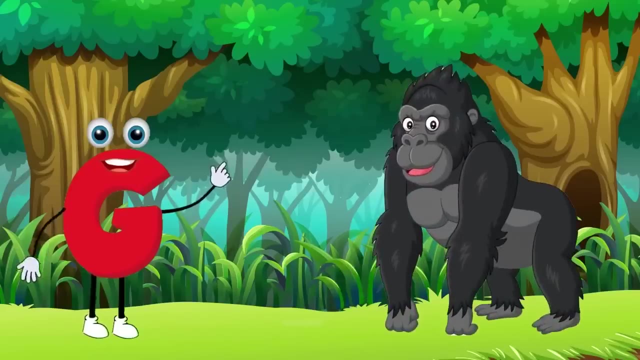 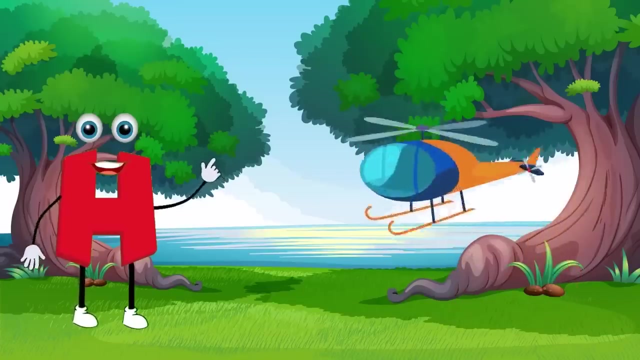 E for Elephant: E, E, E. F for Fox, F for Fan, F, F. G for Guitar. G for Gorilla, G, G, G, H for Horse. H for Helicopter: H, H, H, I for. 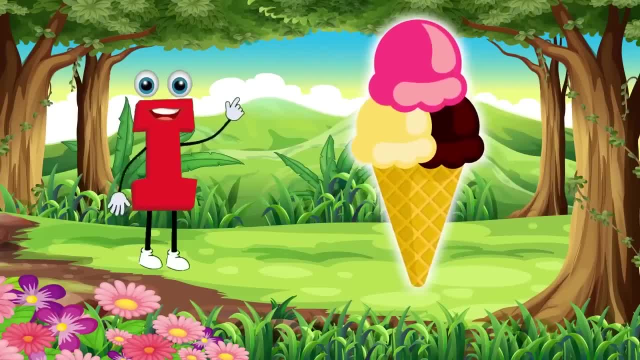 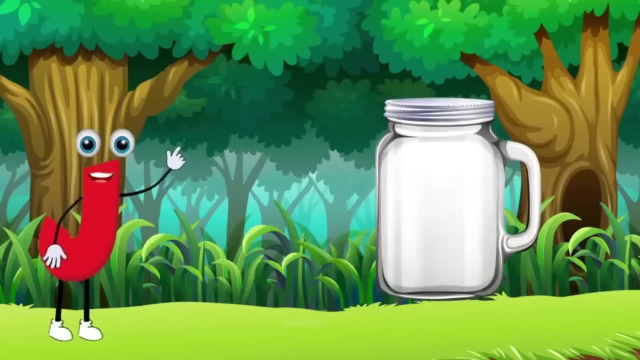 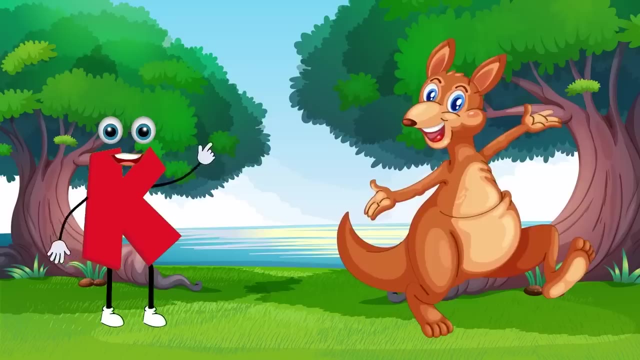 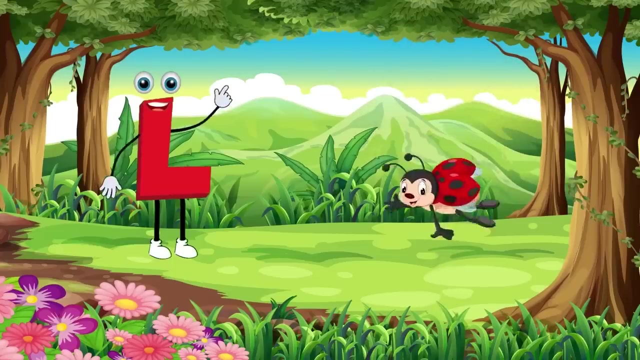 Idea: I for Ice Cream: A A A J for Jam. J for Jar Jar, Jar Jar J for Jam. A A A J. K for Koala, K for Kangaroo, K K K. L for Lollipop. L for Ladybug, L, L, L, M for Mother. 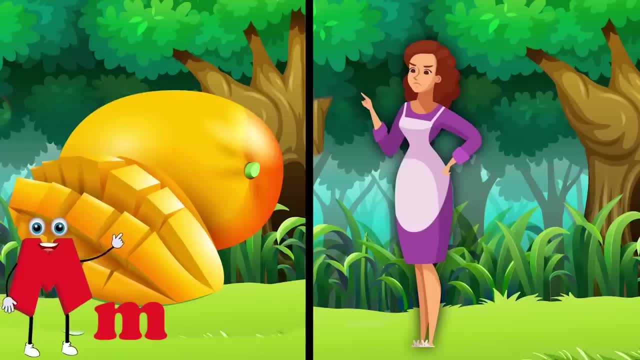 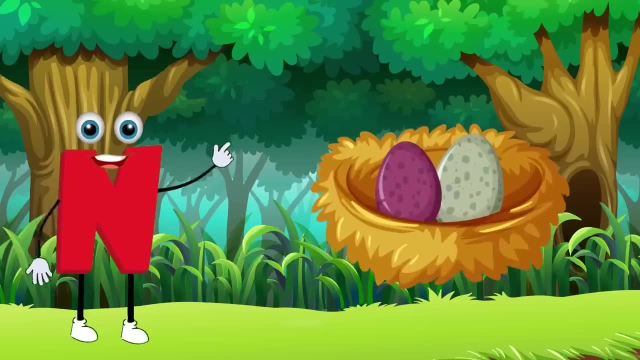 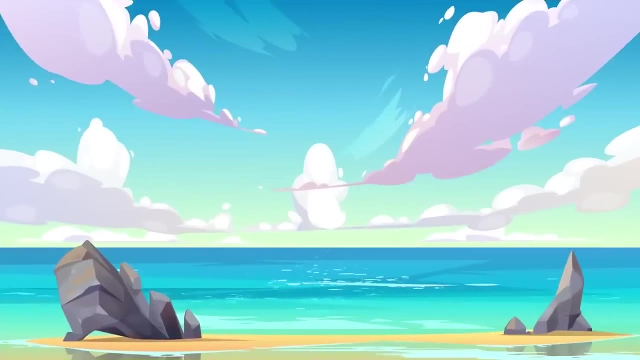 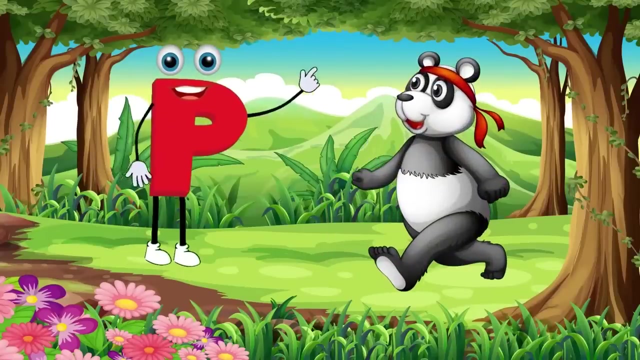 M for Mango, M, M, M, N for Noodle, N for Nest, N, N, N. O for Oboe, O for Ocean, O, O, O, P for Penguin, B for Panda, P, P, P. Q for Queen, Q for Quail. 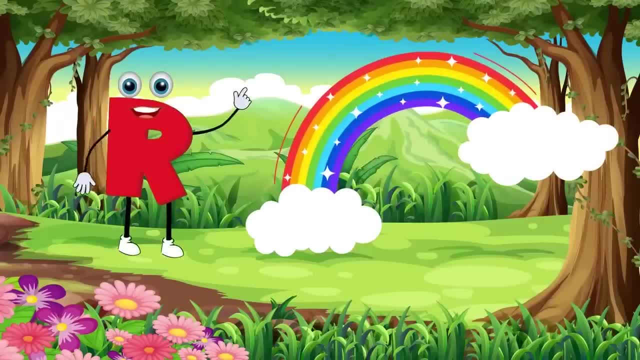 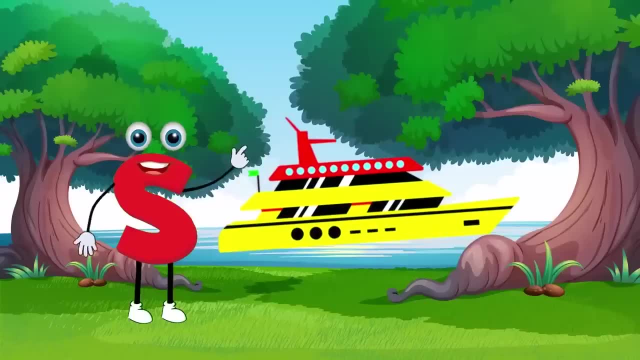 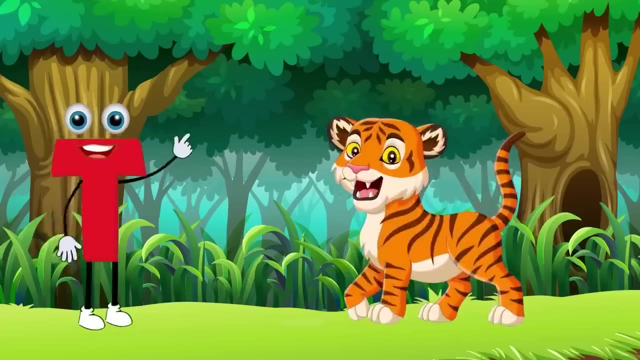 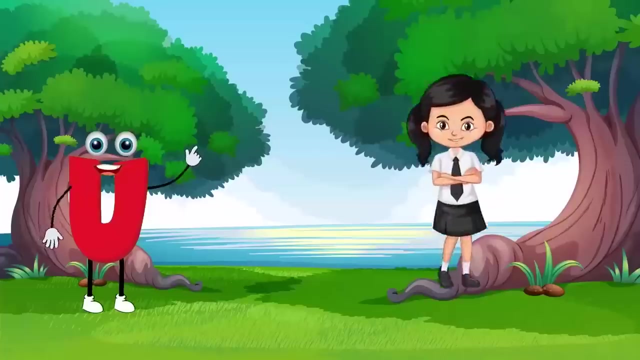 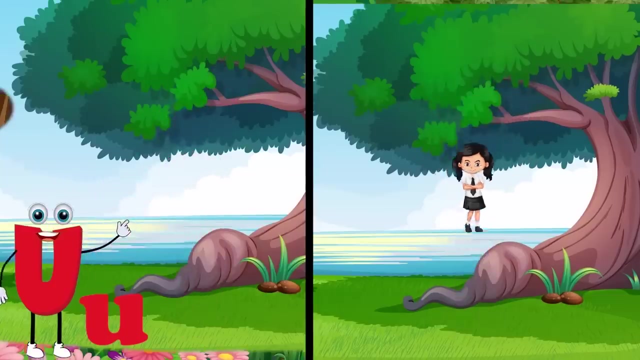 Q, Q, Q R for Rainbow, R for Rabbit R, R, R S for Ship, S for Shark, T for Tiger, T for Tongue, U for Uniform, U for Unicorn V for Violin. 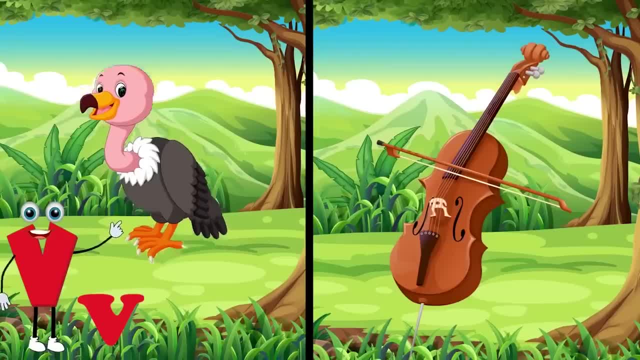 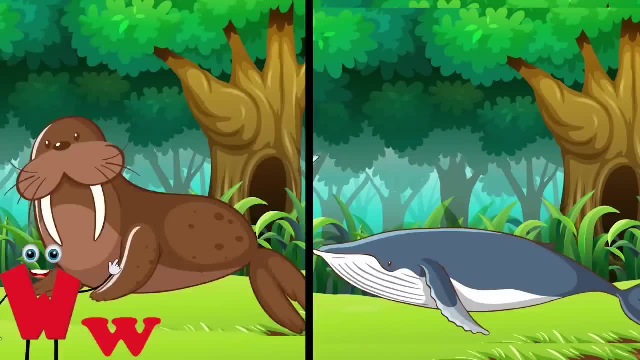 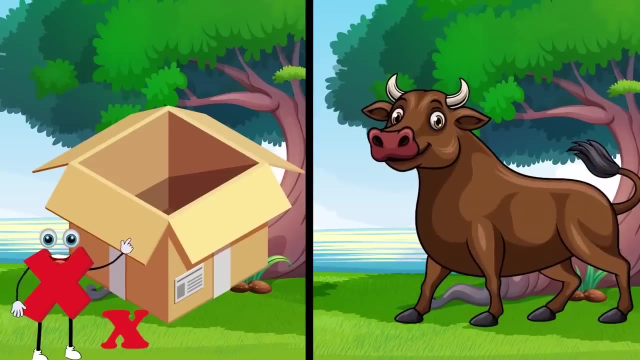 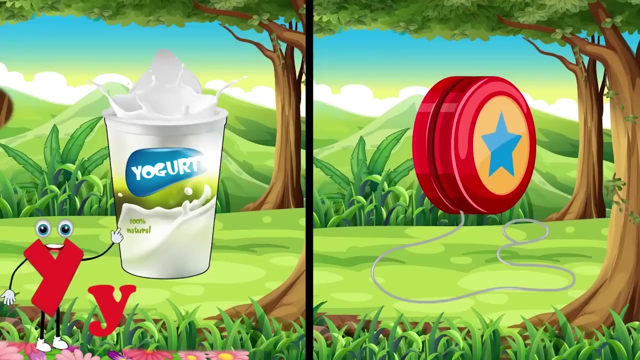 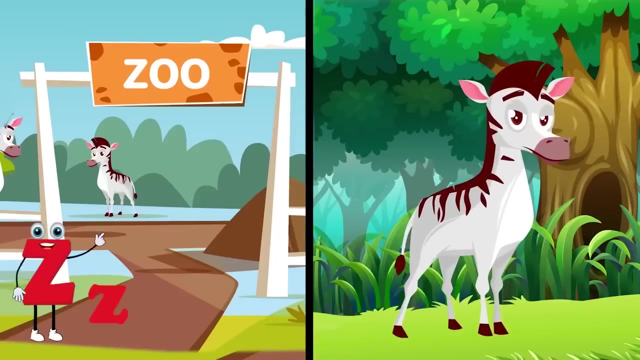 V for Vulture, W for Whale, W for Walrus, X for Ox, X for Box, Y for Yo-Yo, Y for Yogurt, Y Y Y, Z for Zebra, Z for Zebra Zoo, Z Z Z. 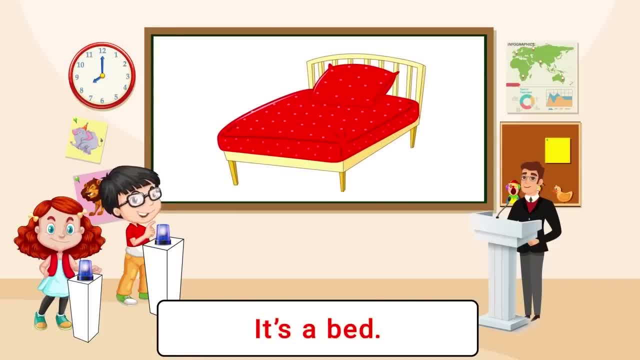 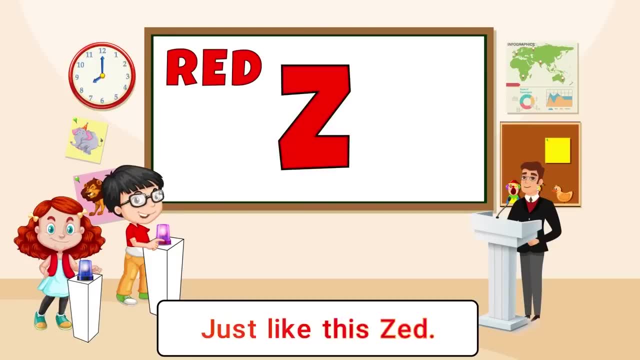 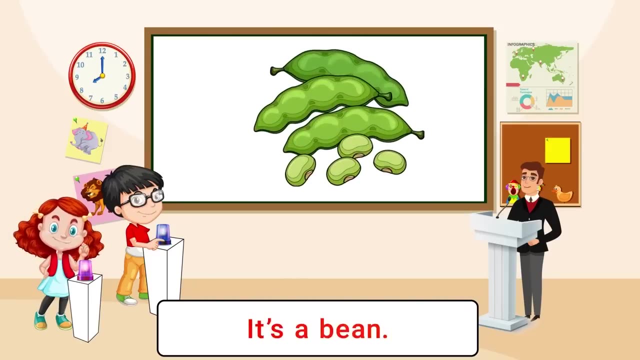 What is this? It's a bed. What color is the bed? Bed is red, just like this Z. What is this? It's a bean. What color is the bean? The bean is green, just like this G. What is this? 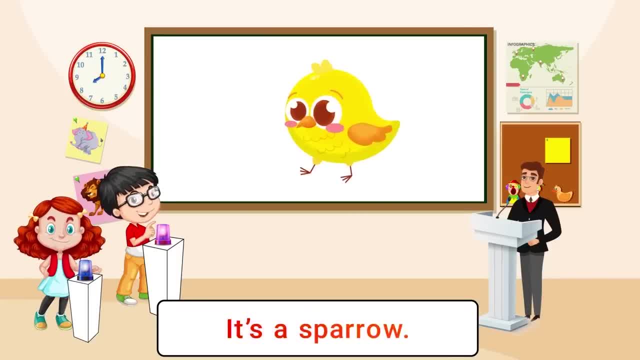 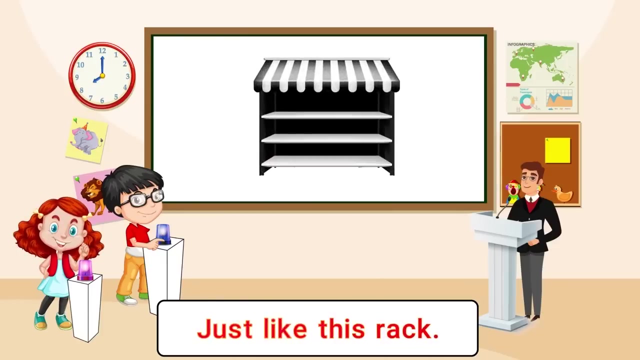 It's a sparrow. What color is the sparrow? The sparrow is yellow, just like this color. What is this? It's a cake. What color is the cake? The cake is green. What color is the cake? The cake is black, just like this rock. 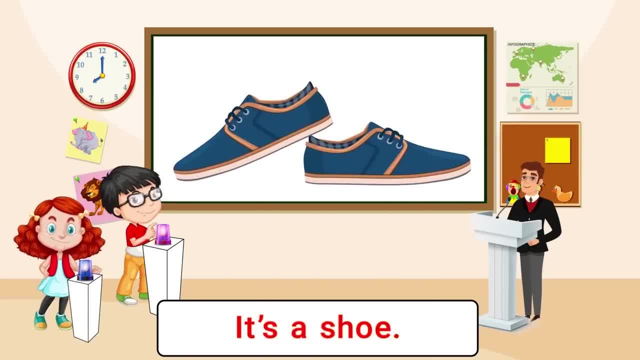 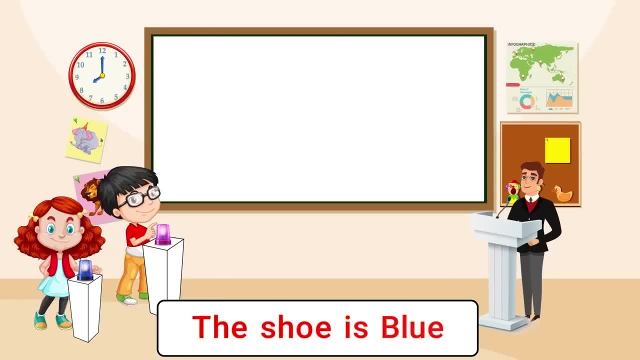 What is this? It's a shoe. What color is a shoe? The shoe is blue, just like this screw. What is this? It's a sausage. What color is the sausage? The sausage is orange, like this orange. What is this? It's a mink. What colour is the mink? The mink is pink. 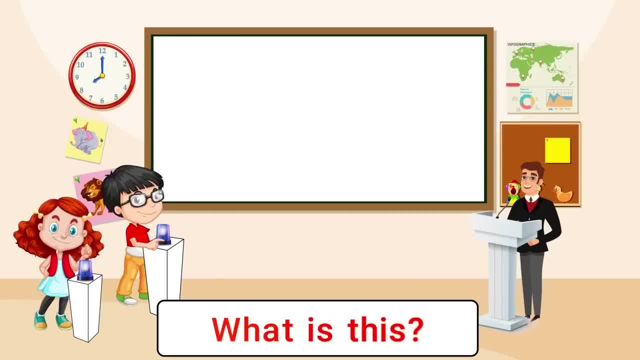 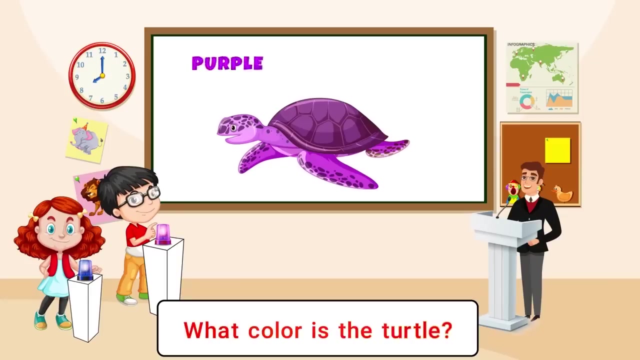 just like this egg. What is this? It's a kite. What colour is the kite? The kite is white, just like this bright. What is this? It's a crown. What colour is the crown? The crown is brown, Just like this ground. What is this? It's a turtle. What's the colour of the turtle? 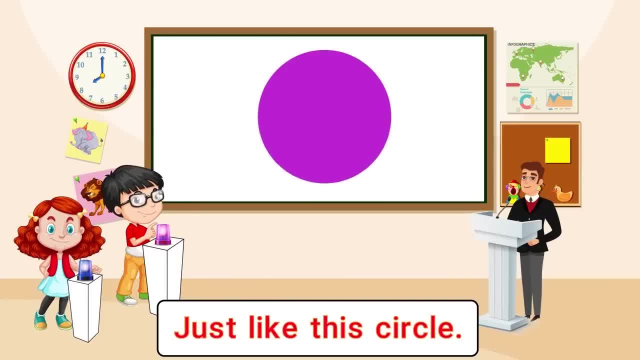 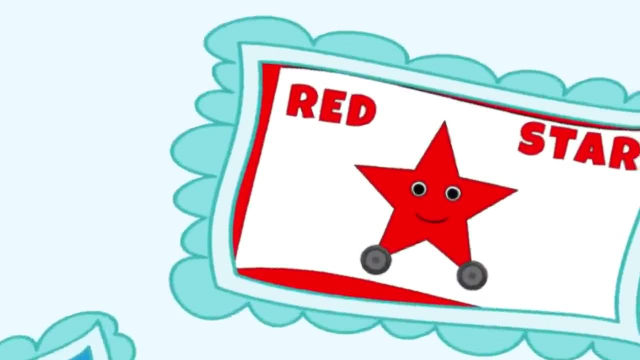 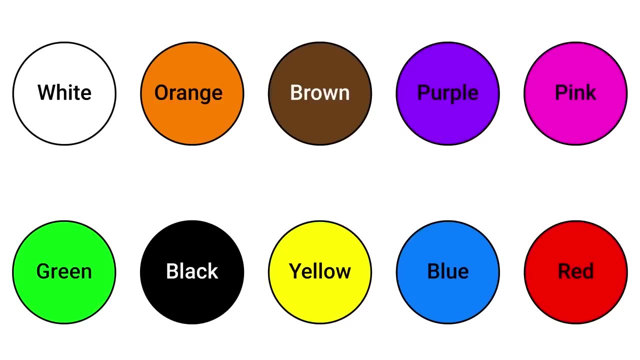 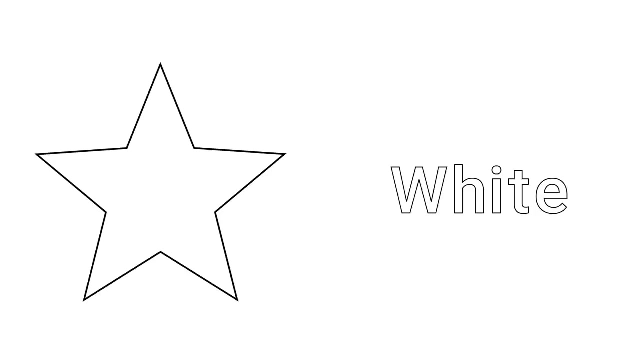 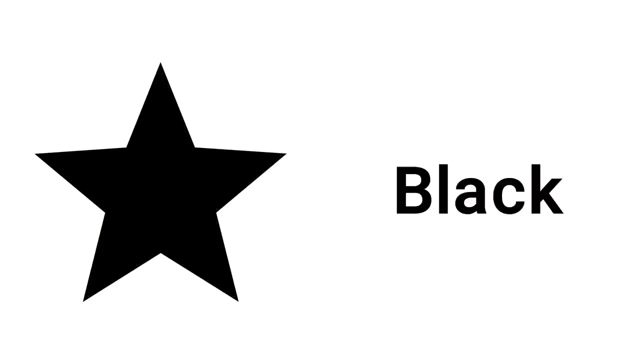 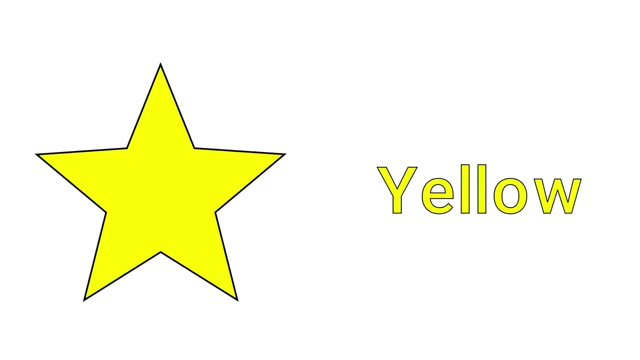 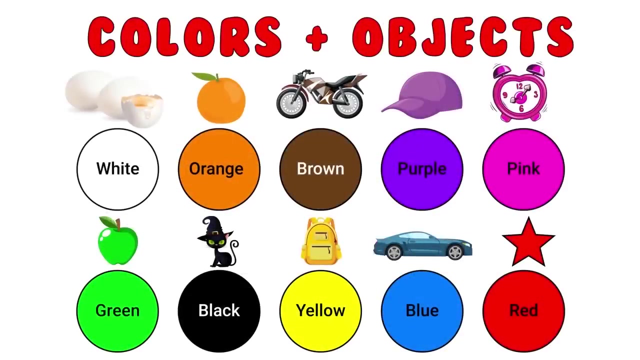 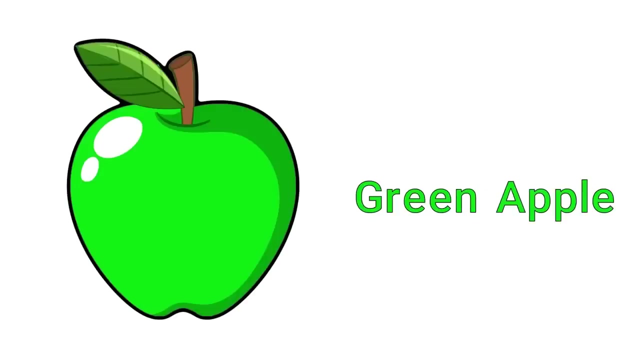 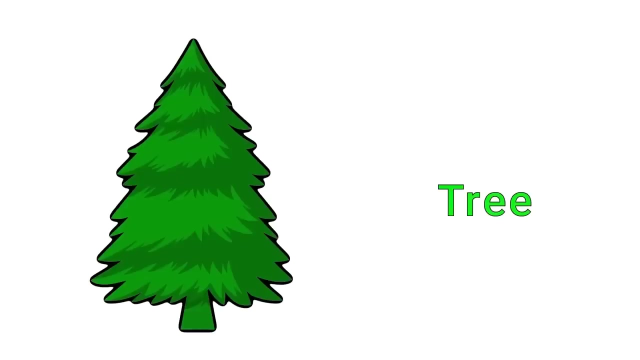 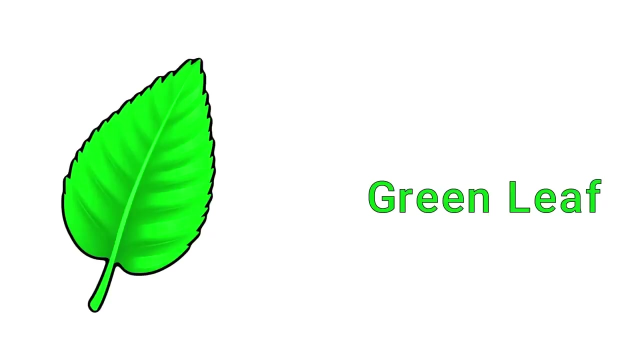 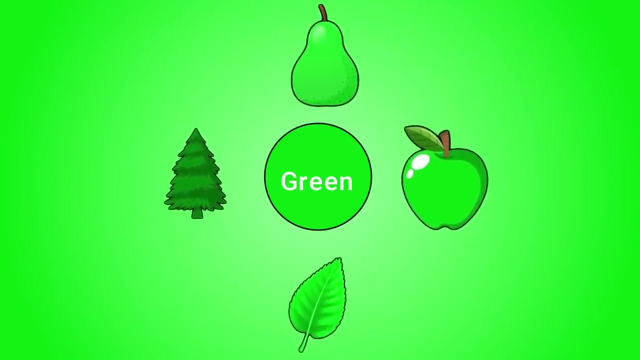 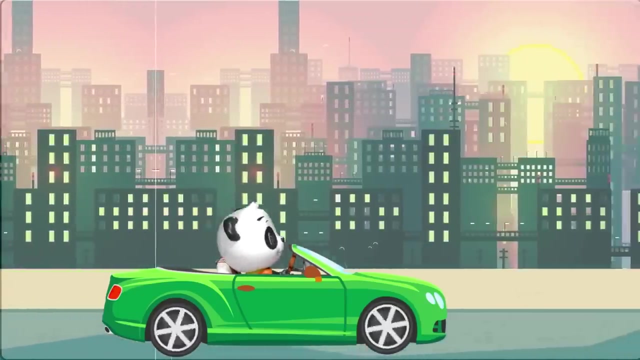 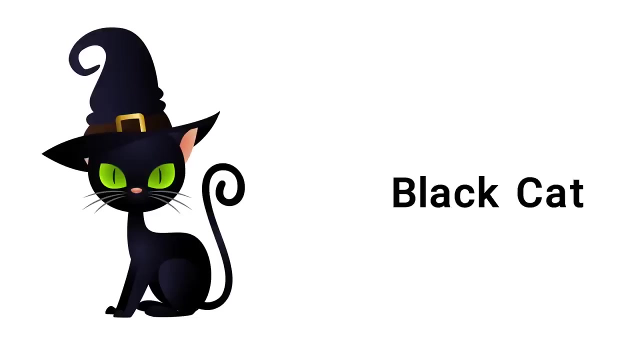 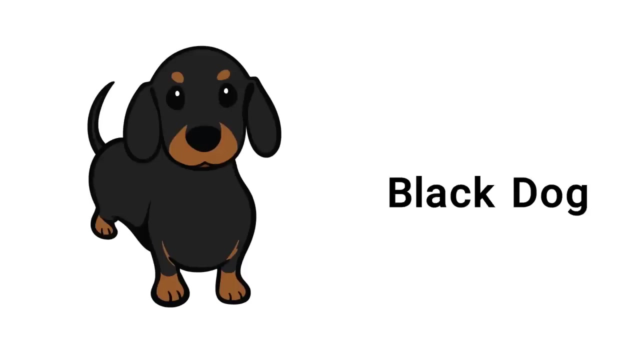 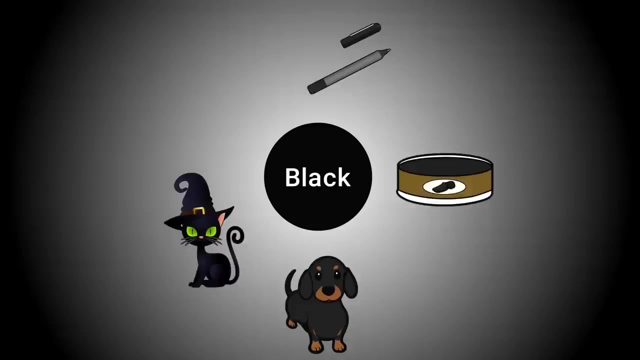 The turtle is purple, just like this circle: White, Orange, Brown, Purple, Pinkごぼう think green, green, green, nerd Green, Black, Yellow, Blue, Red, Green, apple, Pear Tree Leaf, Green car Marker, Black marker, Cat, Black cat, Dog, Black dog. 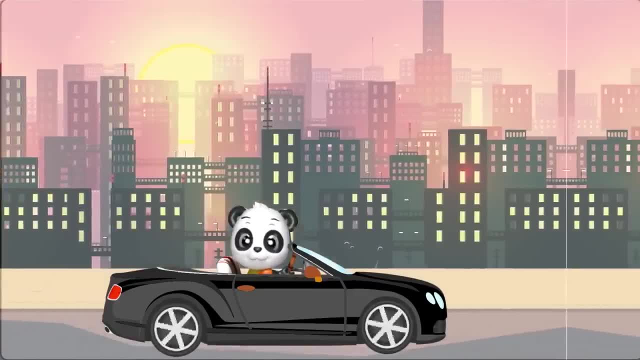 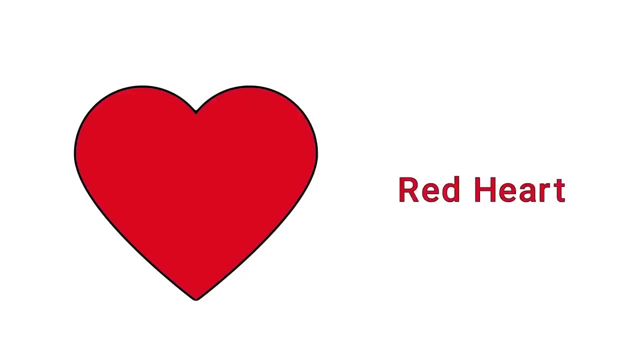 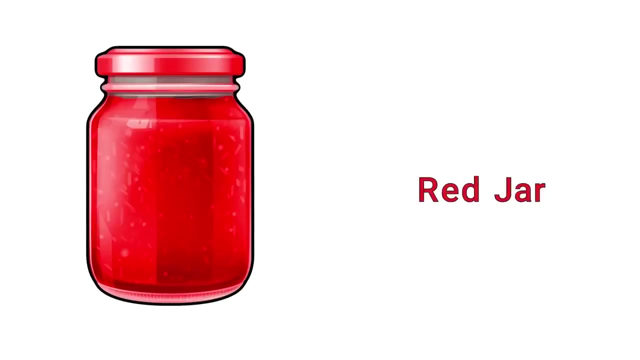 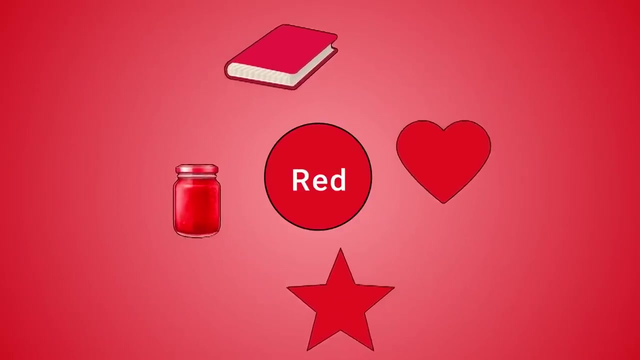 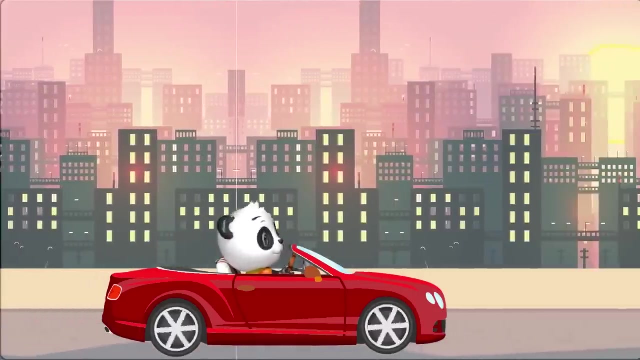 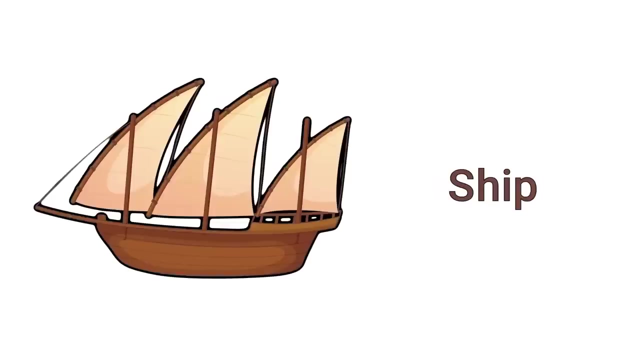 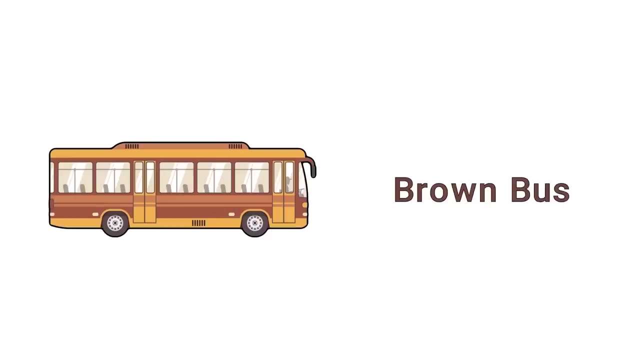 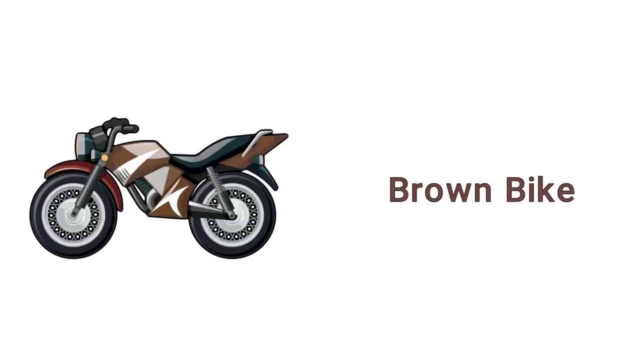 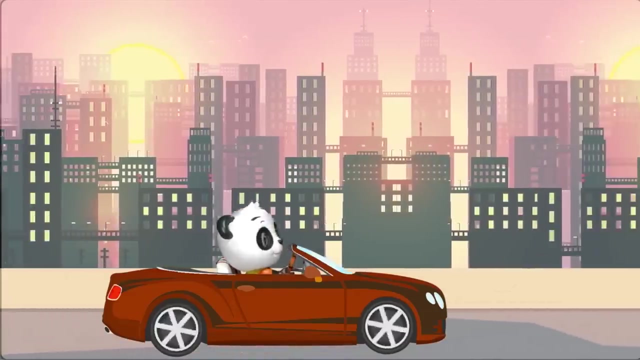 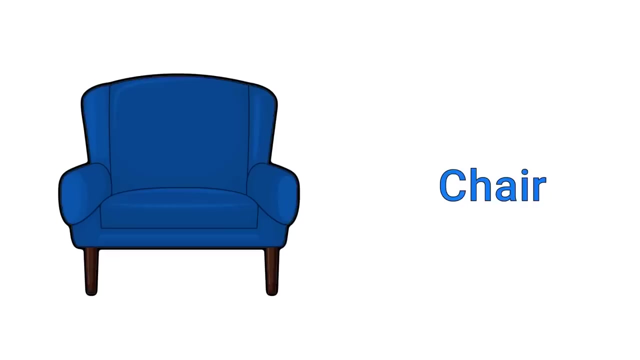 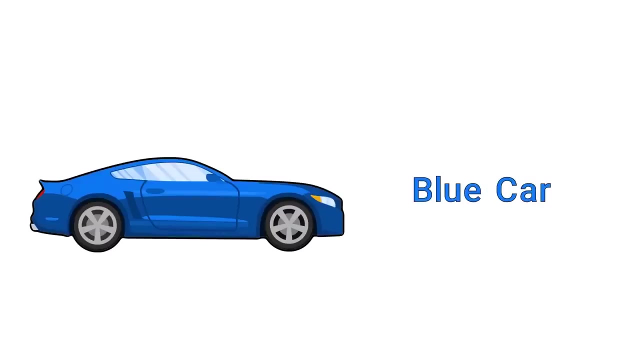 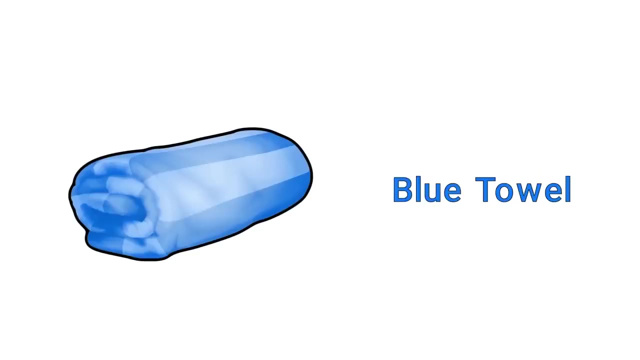 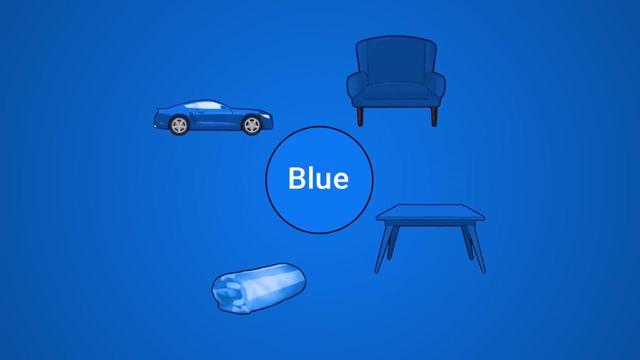 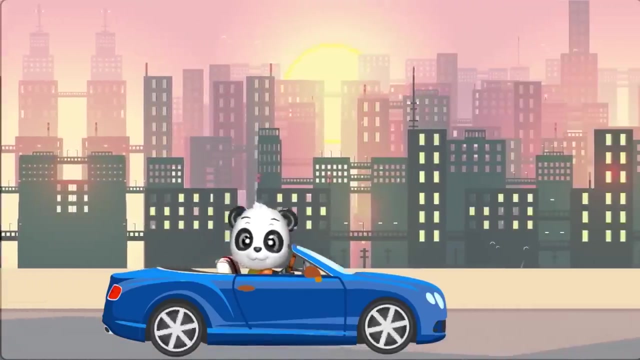 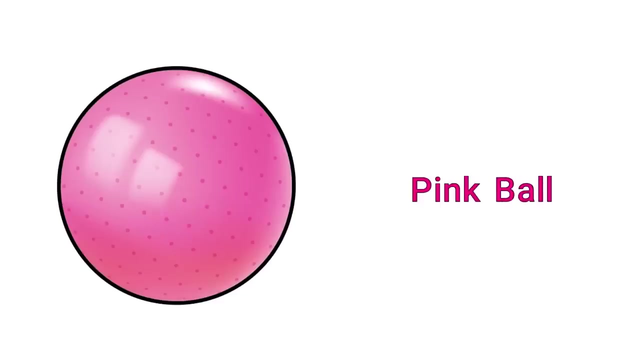 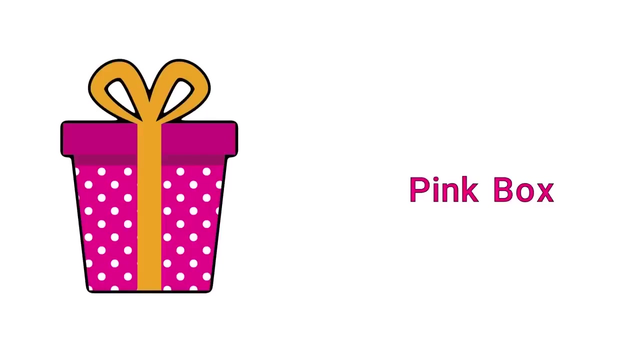 Black car, Heart Red heart Book, Red book, Star Red. star Jar Red, jar Red car. Van Brown. van Ship. Brown ship Bus. Brown bus. Bike. Brown bike. Brown car. Brown car. Chair Blue chair Car. Blue car. Tower Blue tower. Table Blue table Blue car. Bell Pink, bell Box, Pink box. 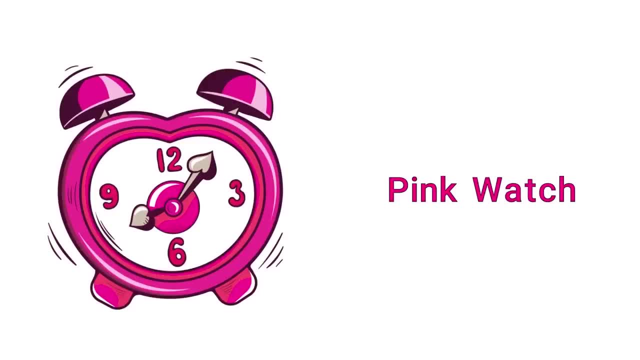 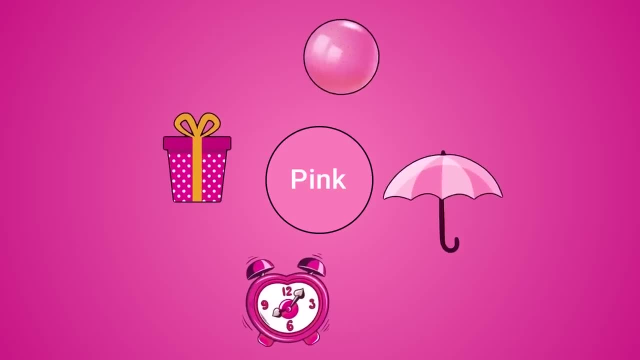 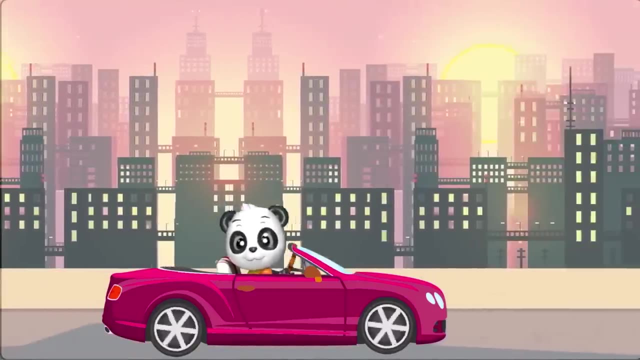 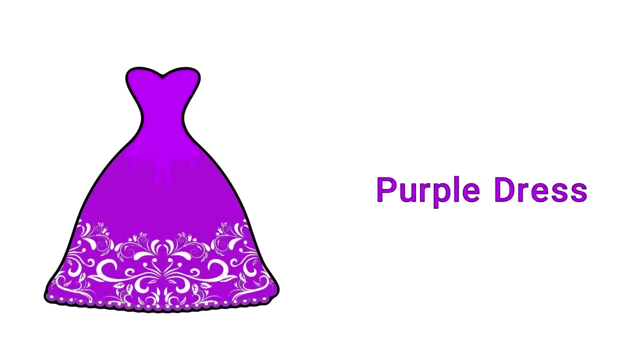 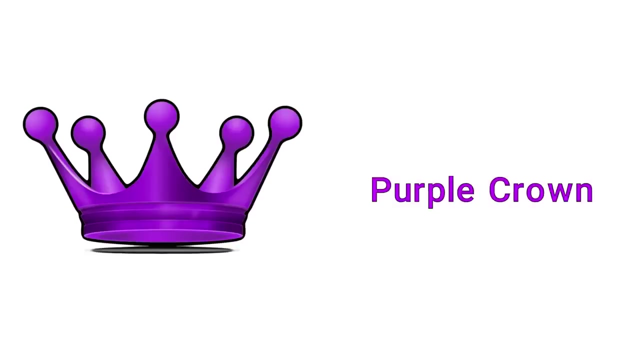 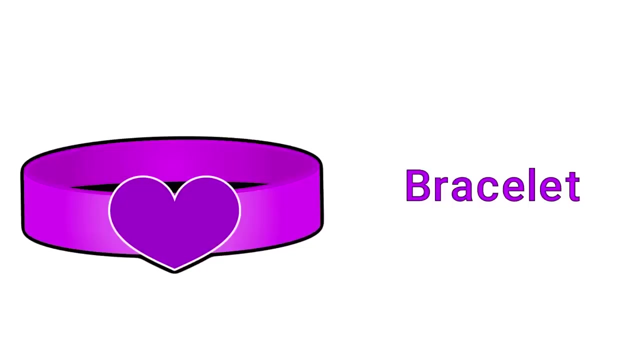 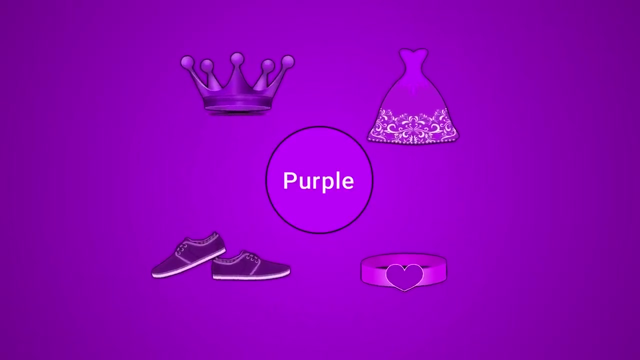 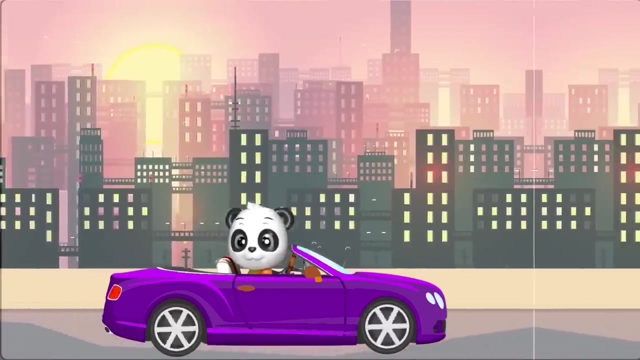 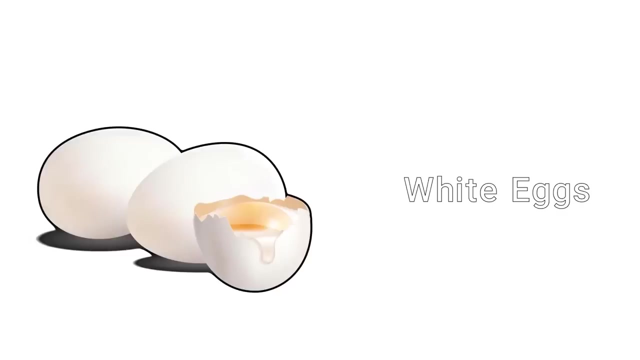 Watch Pink, watch Watch Apple, твои Umbrella, Umbrella Pink, umbrella, Star, Pink, car tonight, Red dress, Purple dress. Coz Shoes, Purple shoes. Bracelet, Purple bracelet. Paprika Egg, White egg, Pig, White pig, House, White house. 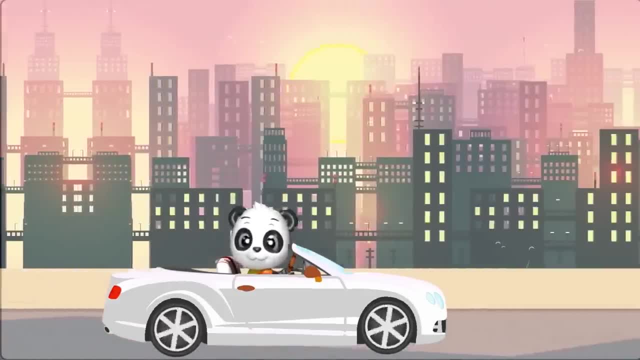 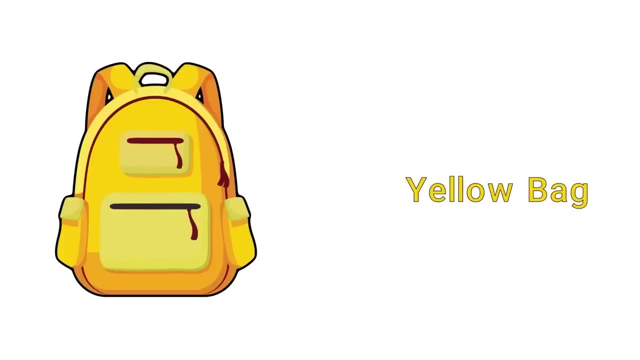 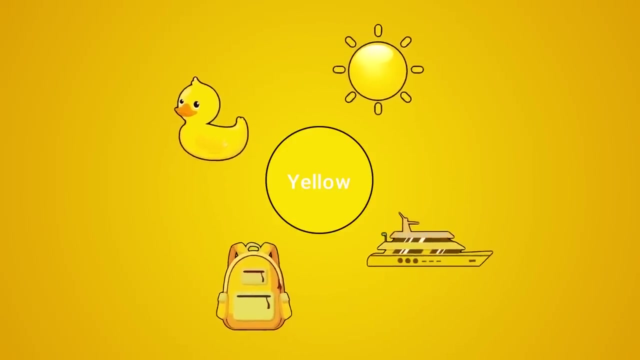 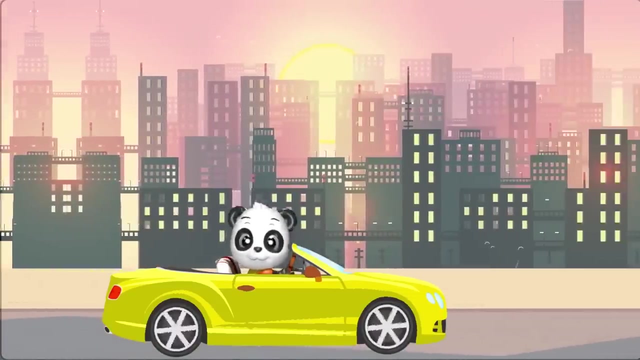 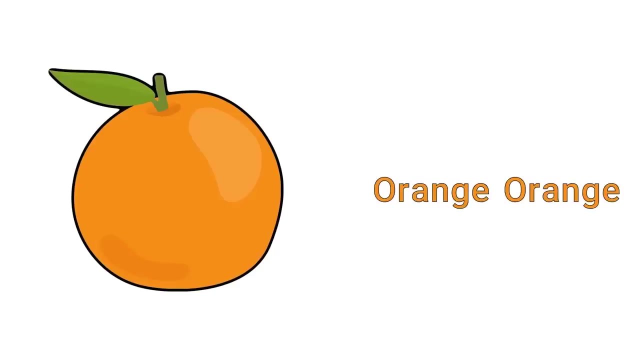 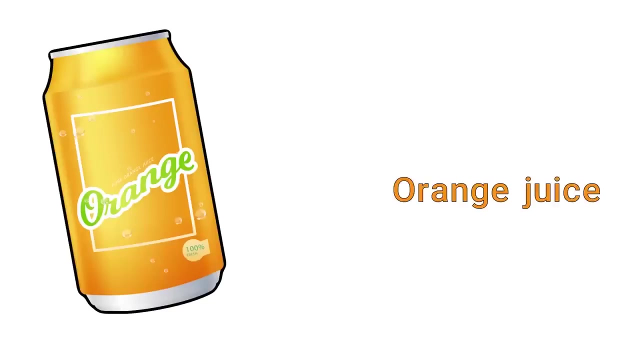 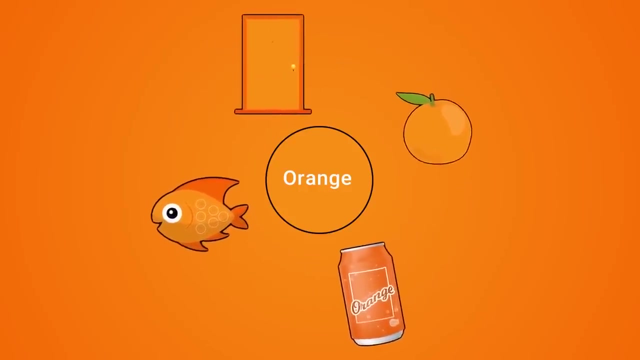 White car Bag- Yellow bag, Sun- Yellow sun Duckling, Yellow, duckling. Yellow car Car. Orange- Orange- Orange Door. Orange door Fish, Orange fish Juice. Orange juice- Orange car Car. 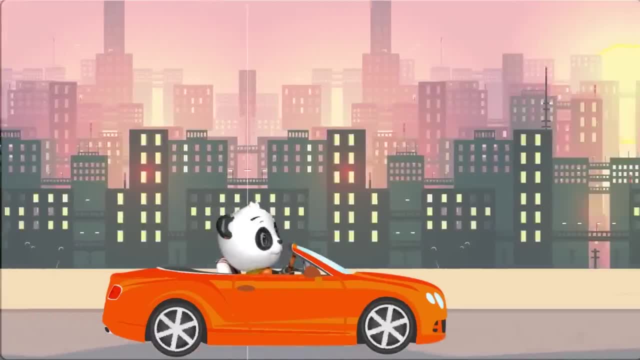 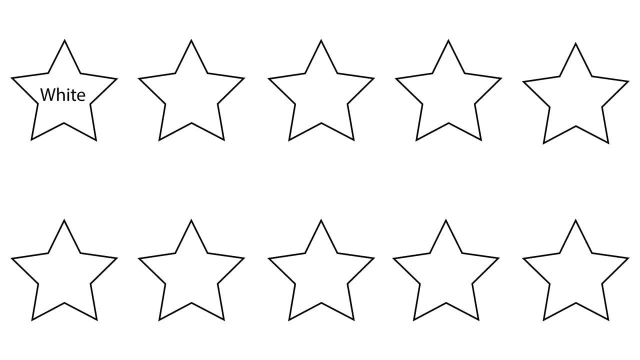 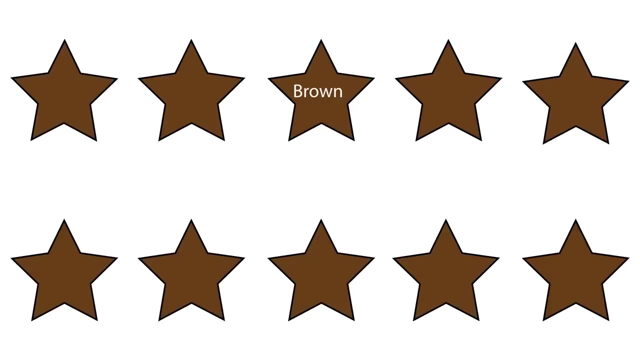 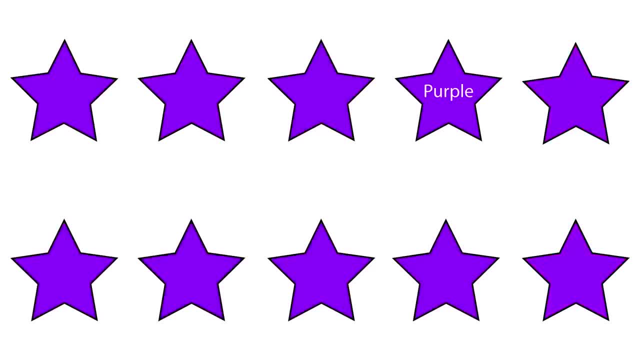 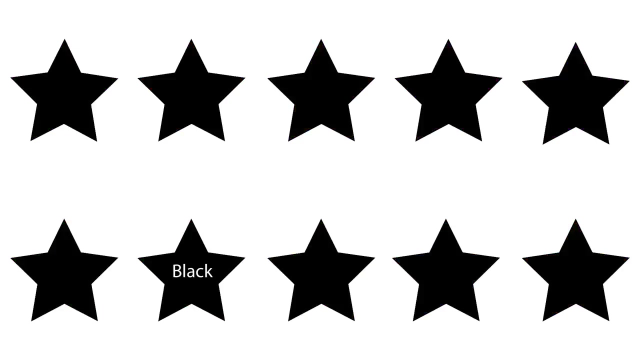 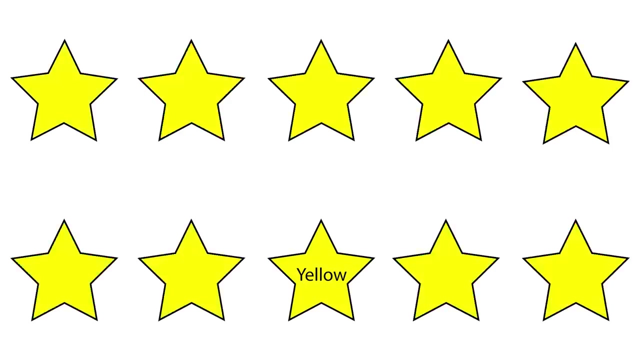 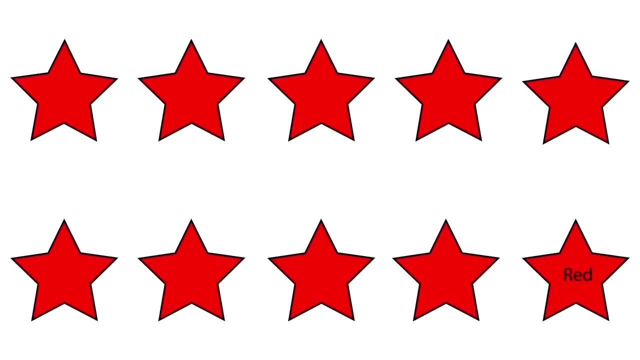 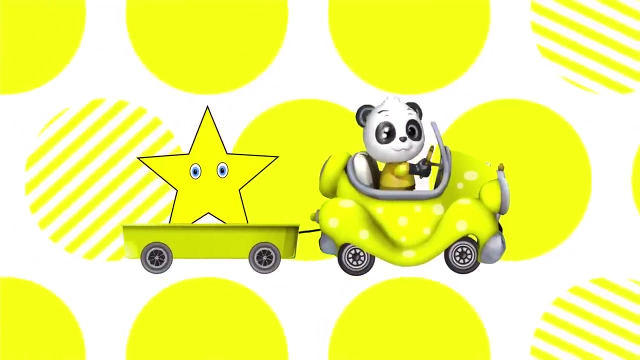 ninguna. Did you all see orange stuff in these bubbles? Wow, Original blue. Final example: White, White, Orange, Orange, Brown, Purple, Pink, Green, Green, Black, Black, Yellow, Yellow, Blue, Red, A little yellow, Little yellow, Little yellow. 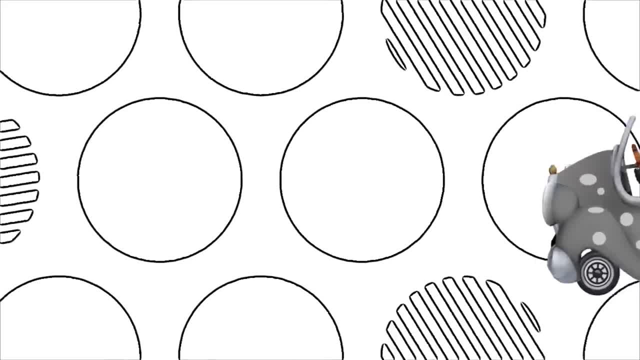 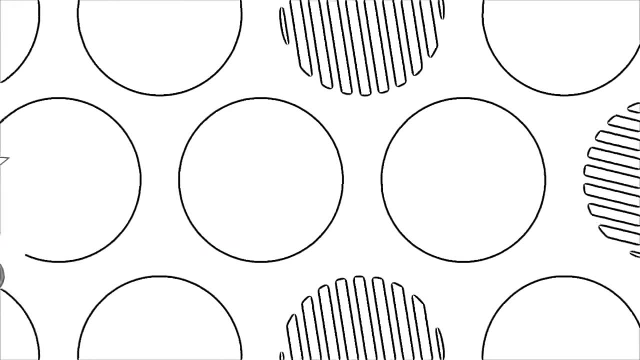